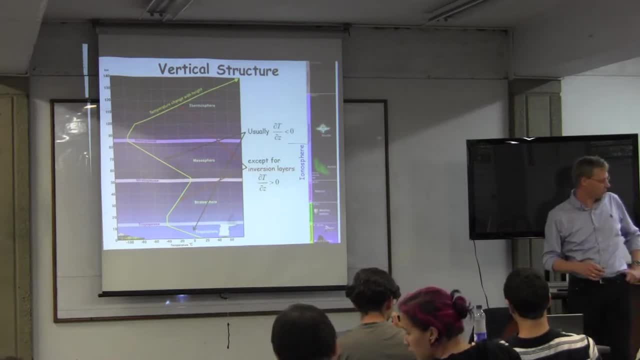 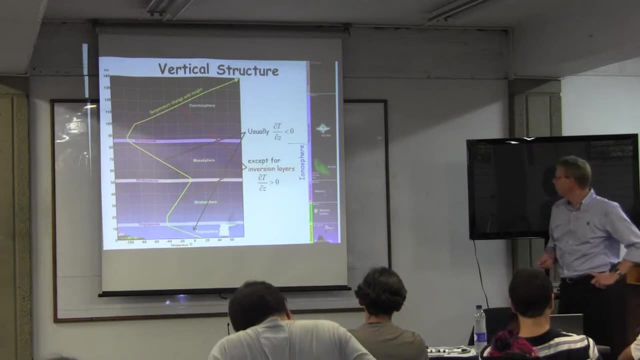 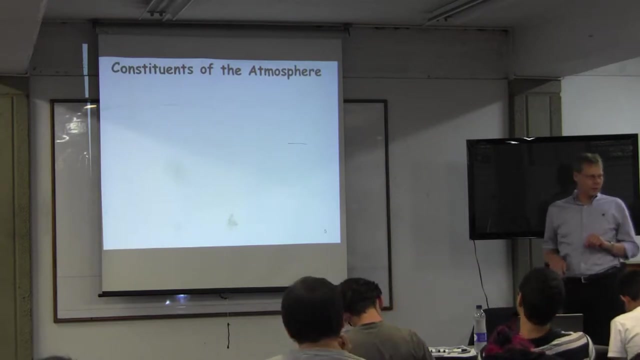 So I think it was once possible actually. Yeah, And astronomers said that if you go up hundreds of kilometers, then you're close to what people consider outer space. So don't turn your sheets around, Don't, don't leave them. 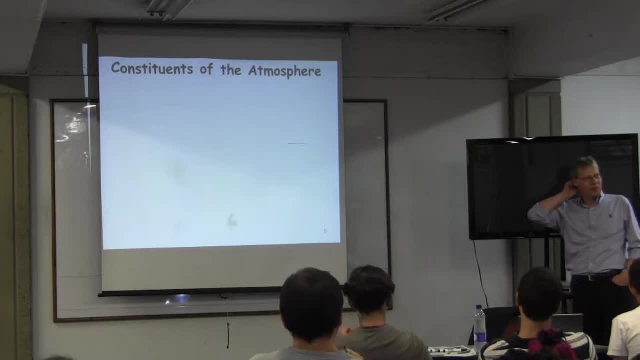 What do we know about the atmosphere? What other constituents can we? What's in the atmosphere? I have a question. I have a question. This is- I mean the list that we will look at here, of course, this also that's very relevant to astronomers. 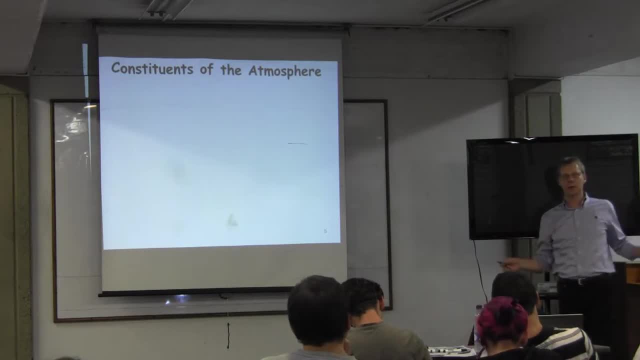 And yeah, there may be other elements in there. Of course, if you live close to a factory, you may have all kinds of poisonous gases. I didn't list it out here, But what's important for astronomy? of course, for everyone. it's important to have oxygen and nitrogen there. 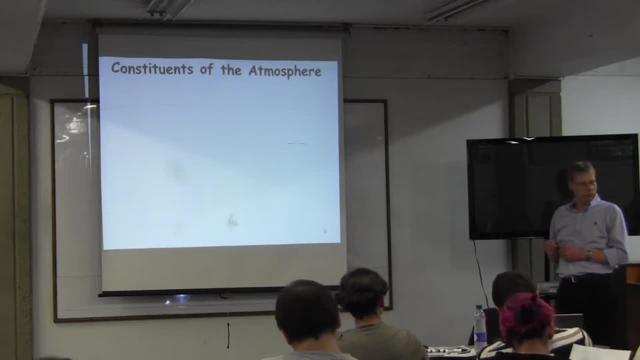 You know approximately what relation, in what percentage It's close right. So 87% oxygen, 21% the same nitrogen. So that gives us 99%. 99% of the atmosphere is oxygen And that's actually a relative constant ratio up to 100 kilometers. 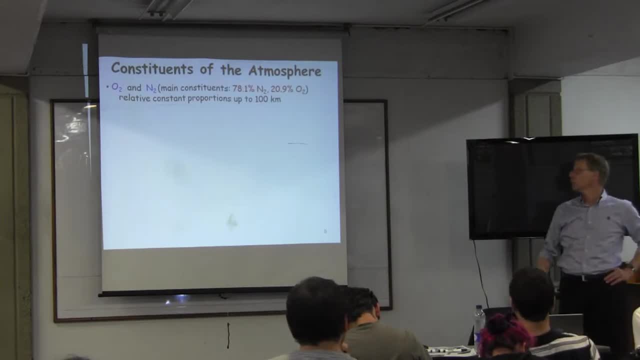 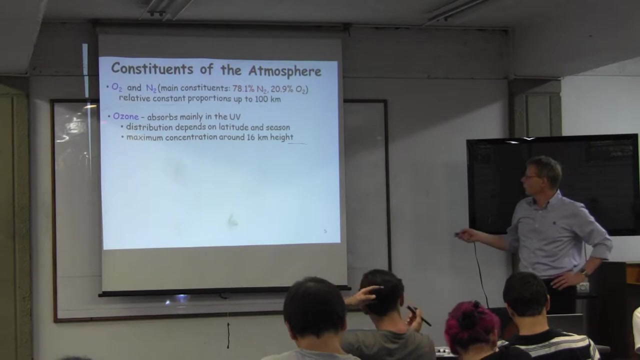 So it doesn't matter how much oxygen you have, It doesn't matter if you take a balloon and measure, you will always find this ratio up to very high. Then there is ozone, And of course ozone also, yeah, well, it's a very I'm not sure how it's here. 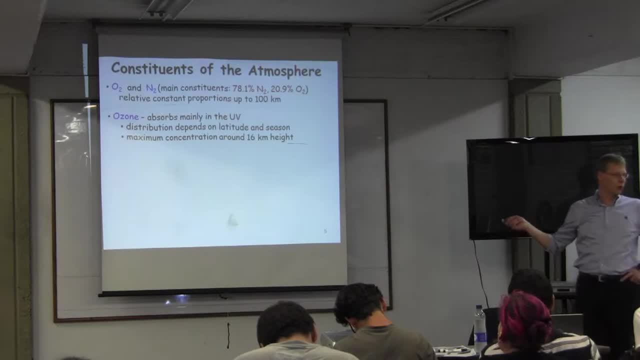 but at least in Europe there's often ozone warning which you should take seriously. if you go jogging or run aeroports when the weather is really high a lot in summer, Right, And there's some increased ozone content, But astronomically speaking, it's mainly because it absorbs the UV radiation. 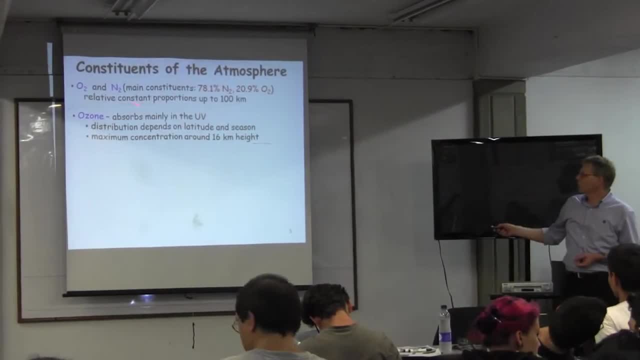 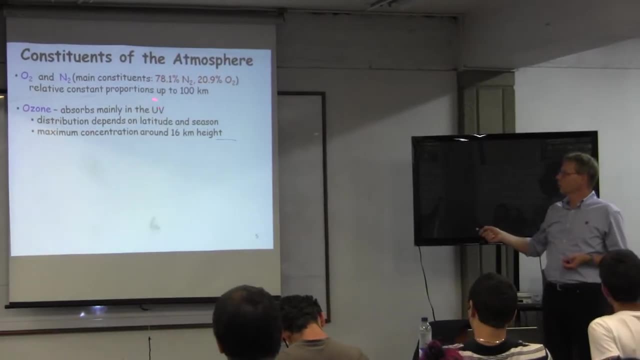 And well, of course we know that from climateology studies. right Where you have a hole in the ozone layer up there, then of course a lot of the UV light comes through. This is, of course, where parts of Australia, for example, suffer from. Simply because, well, there's very few animals there. Some burn, But then the distribution depends very much on the latitude of the season. But, as I said, it's the maximum concentration around 16 kilometers height. Then of course we have CO2.. 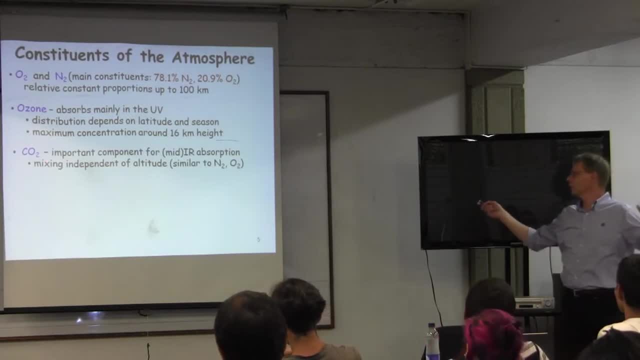 Now that's going to put we all well. cars produce CO2. And it's important it is, of course, I mean there's not much left here, since this is 99%, But the CO2 is important. The CO2 is important because it's very strong absorbed. 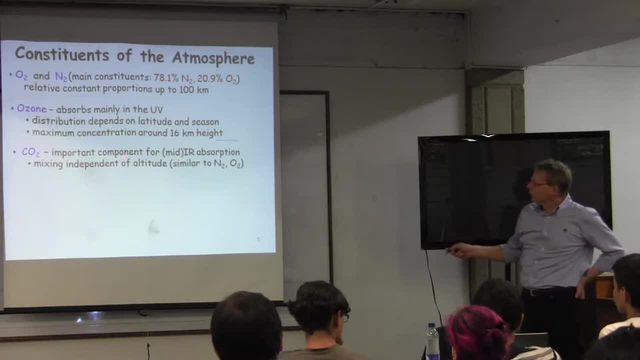 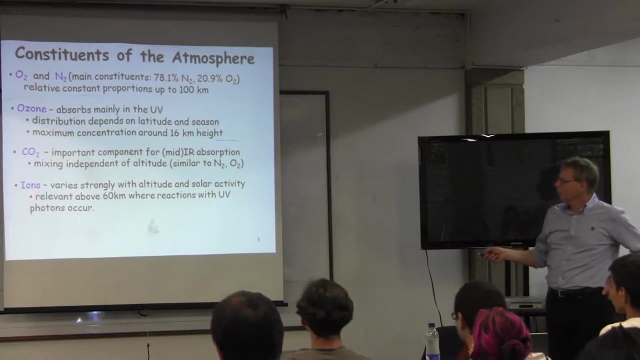 Meaning that it absorbs. we see some spectra later how things get absorbed, But it takes out a lot of the radiation that we've been through And that makes it very difficult on the ground. Then we have ions, And those ions are mainly above 60 kilometers. And that is because, well, the sun produces lots of uv photons, And the uv photons from the sun they bombard the upper layers of the atmosphere And then they ionize whatever is up there. And because the density is low, these ions, they well remain ionized for hours. 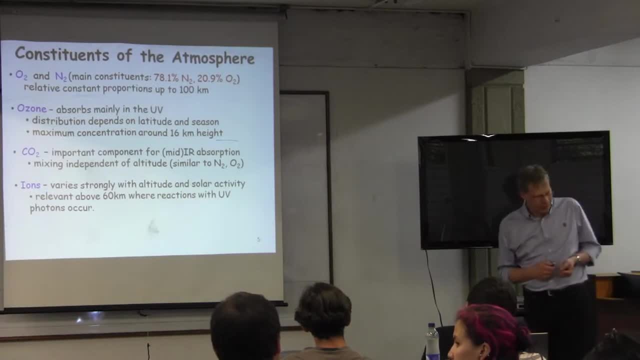 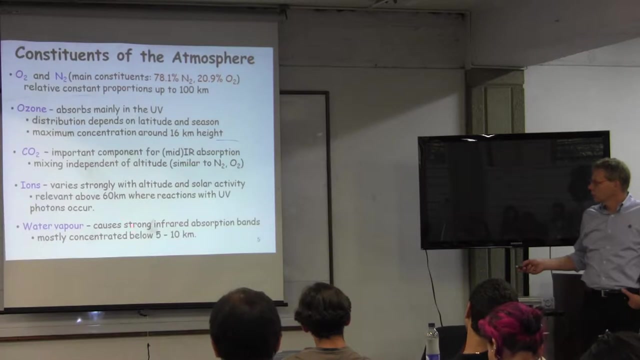 They do not immediately recombine, But they remain ionized And this absorbs a very specific wavelength. And then, finally, there is water vapor, And so, if I ask the Brown-Weiser Observatory in Colombia, that may be one of the reasons. 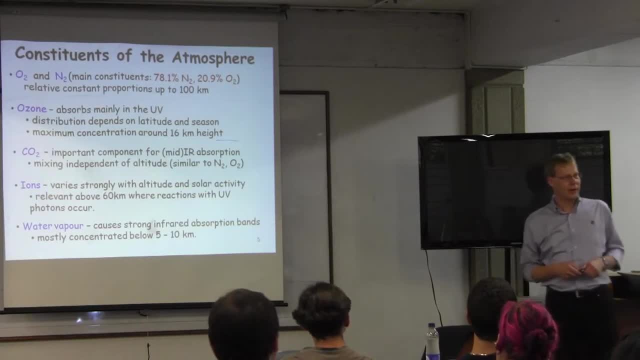 Because clouds are bad And there may be. I mean, even if it doesn't really show up as a problem, if it doesn't really show up as a big cloud. the water content is significant, And so it absorbs a lot of the radiation. 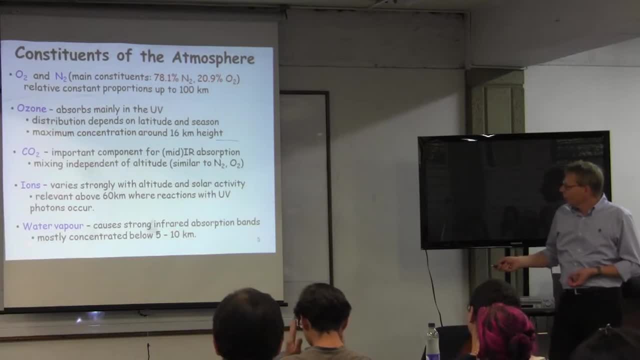 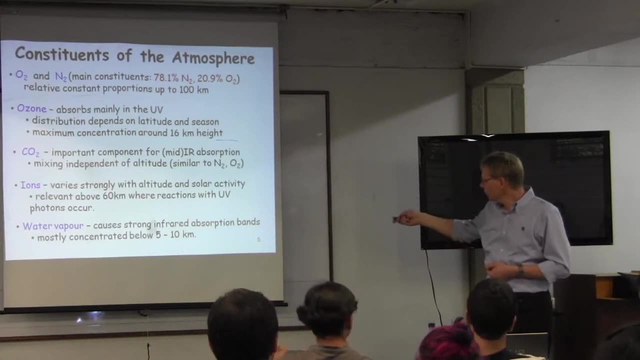 And then, yeah, that kills the observation. Now, the water vapor, however, is mostly concentrated below 5 to 10 kilometers, which is actually good. So if we have- well, like Mars has right, If we have- a mountain that's higher than 10 kilometers, 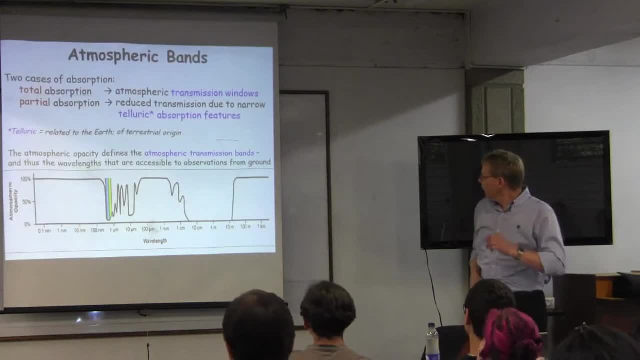 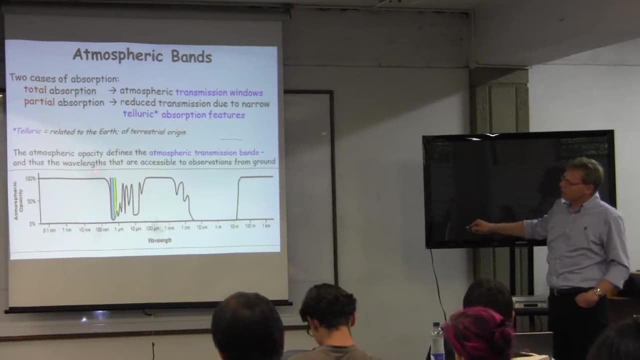 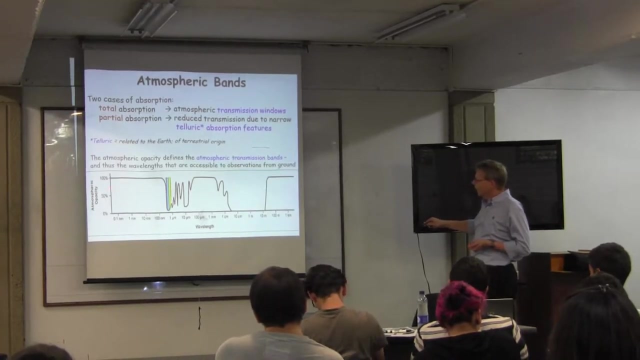 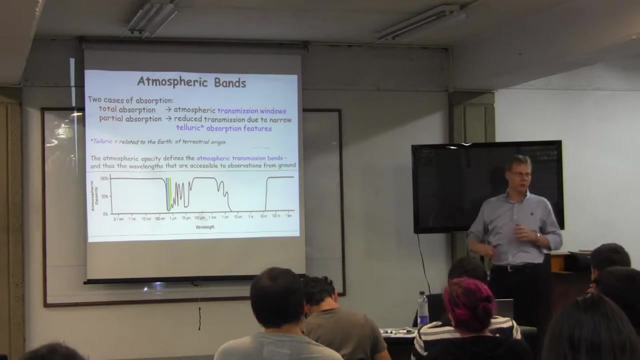 it's not going to absorb a lot of radiation. But let me show you what's happening here. This is a plot of the atmospheric opacity, Or you could say transmission- Oh sorry, Opacity versus the inverse transmission, Meaning that if it's 0%, perfect, if it's 100% opacity, it means nothing will hit. 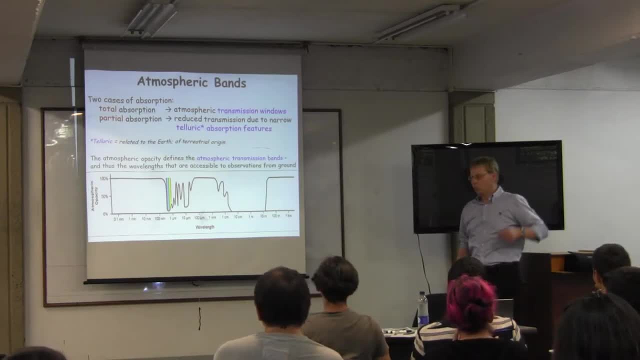 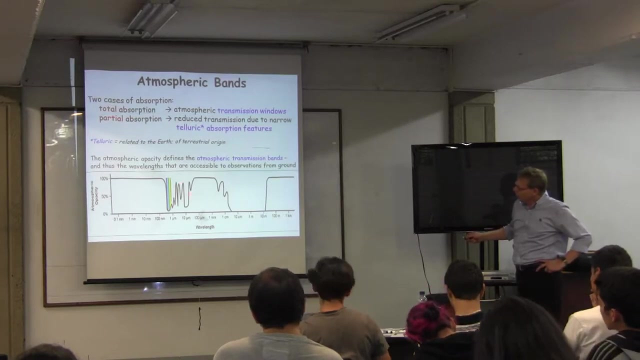 Right. The window is close to 0. The wall has opened. So you have generally two cases of absorption. You have bands or wavelengths ranging from total absorption, like here, And your light will be observed on the ground through those wavelengths, And you have partial absorption, like in this range here. 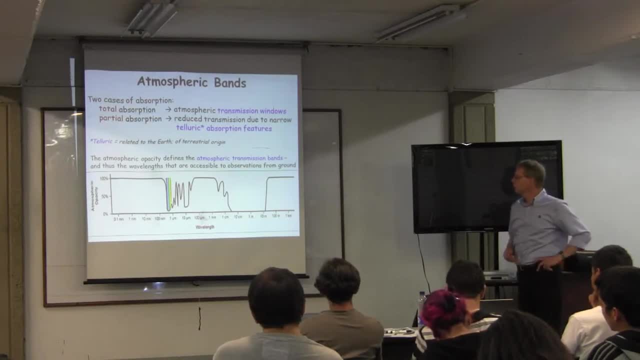 where, on average, transmission is reduced, But you will still be able to see something. So it's not perfect. Well, at the visible inverse it's perfect, And it's probably not a coincidence that humans have developed eyes that are sensitive to the light that we can see. 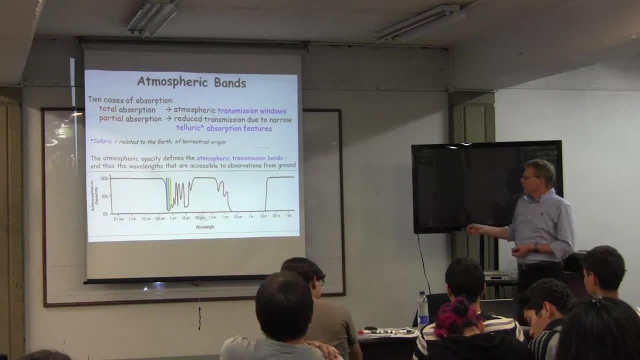 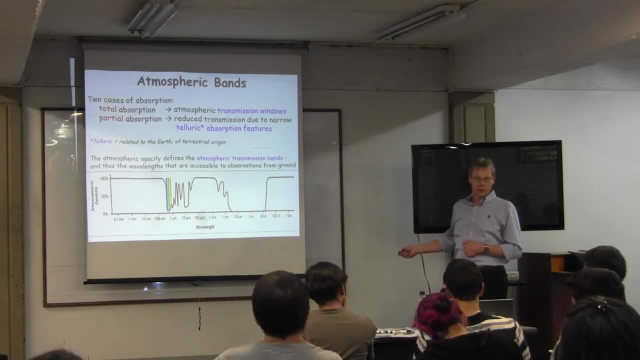 and not to wavelengths that are being absorbed. But yeah, So this is the spectrum we all have to deal with when we do observations, Where this little percent, this cluster of no visible light is because there are people who are wide awake. 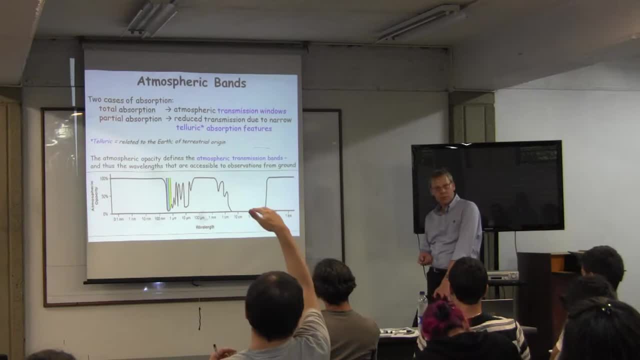 Because I was supposing that the visible light reached the sub-virus totally. but Oh, you mean, the sub-virus is not at 0%, It is close to 0.. But well, if you would take a, let's say, a very high-resolution spectrograph, you would see lots of individual lines from the atmosphere. So even in the visible wavelengths there are lots of individual molecules- sorry ions- and elements that absorb the light We actually can. I mean the situation is very good there. It gets worse as longer wavelengths. 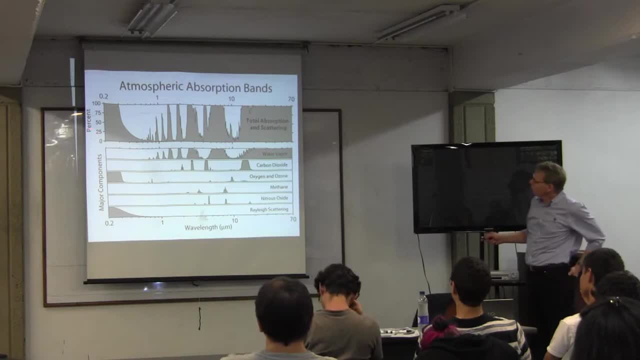 and we can see how it is. So this is again the percentage. This is a function of wavelengths, so you can see how it goes down here And there you see the different components that contribute to this absorption. So if there is a lot of gray it means it's bad. 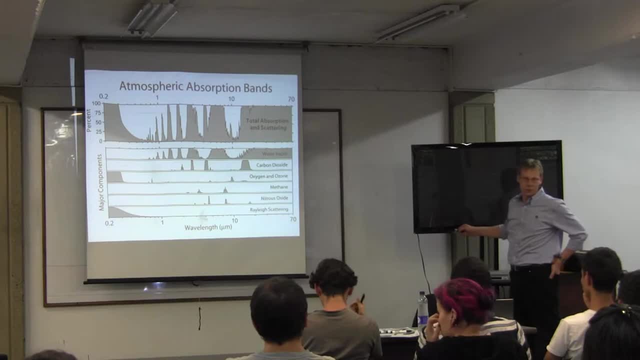 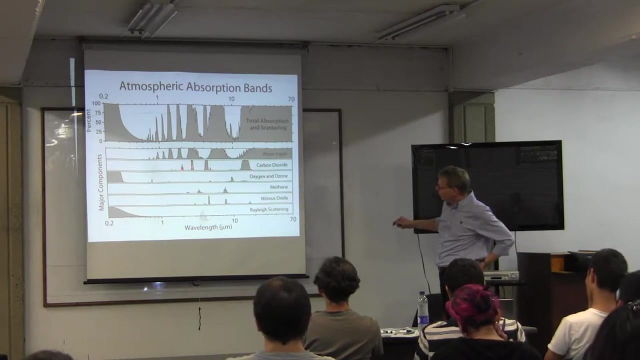 So obviously the water weight there is probably the worst thing, And the water weight absorbs everything for a longer period of 15 microns almost. Then you have carbon dioxide, CO2, and you can see there are very distinct wavelengths. It makes the atmosphere opaque. 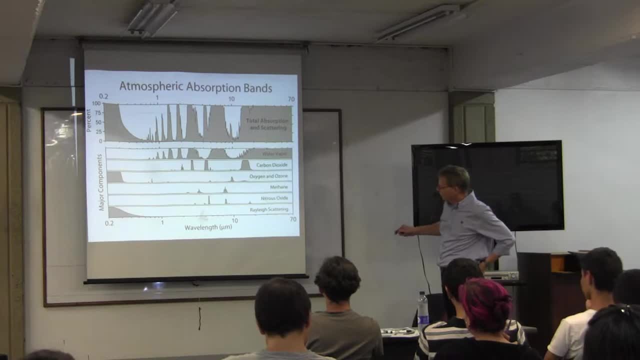 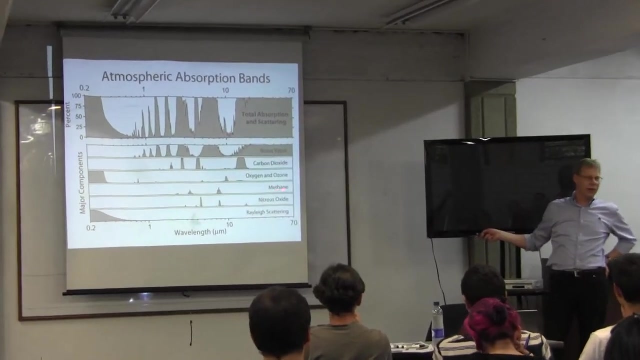 Oxygen and ozone, as I said before, in the UV, but also some features here, And methane is an. I know who you are. you may not like methane. It's a key molecule that you would like to observe in exoplanets. 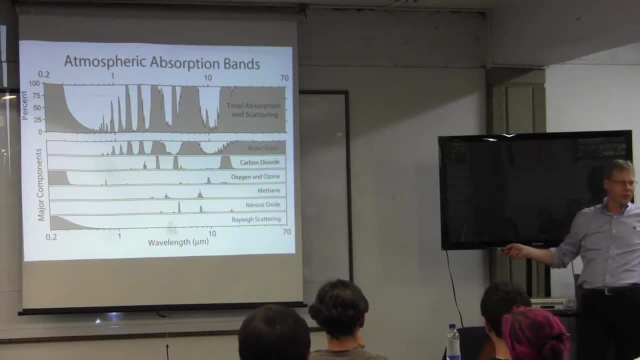 And once you see methane, of course, then it's a good measurement of the composition of the exoplanet atmosphere. The only problem is the light that comes from the exoplanet goes through the atmosphere of the exoplanet and then it goes through our atmosphere. 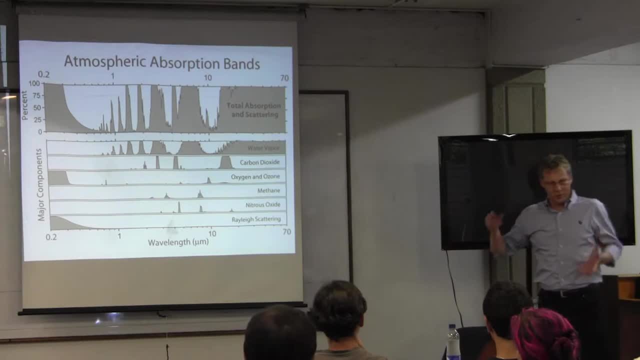 And it's also methane. And so to figure out, do I really see methane in the exoplanet or is it just because I didn't calibrate the atmosphere of the Earth properly? That's one of the big challenges. So well, you can see, it's very nasty. 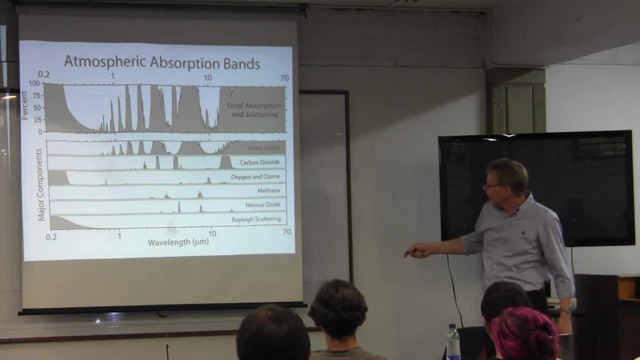 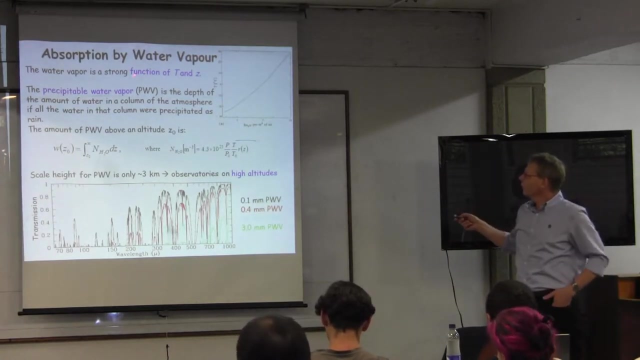 And you can also see here that in the visible wavelengths here a lot of the or a significant part of the, the defenses are down to zero. It's simply from ray scanning. And let me say something about the water vapor. This plot here shows temperature. 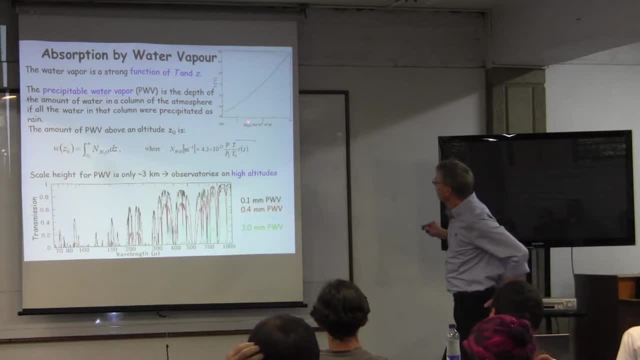 as a function of the- let's say, the amount of water per cubic meter of air. So how much water can this water vapor contain in a cubic meter of air? If it's a lot more, then it starts raining And you can see that, of course. 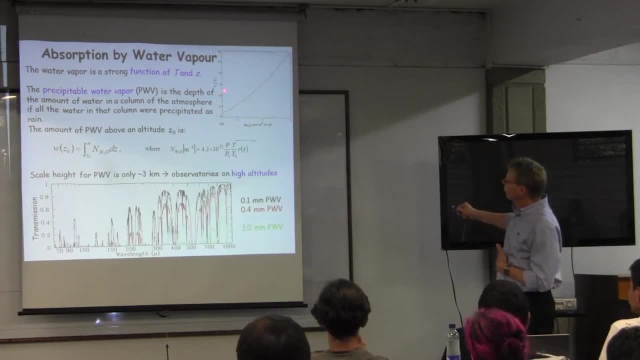 if the warm air is warm, then it's warm. Here is the temperature. But there can be a lot of air, a lot of water in the air. If you cool it down, then the content is very small, And so if you go up on a high mountain, 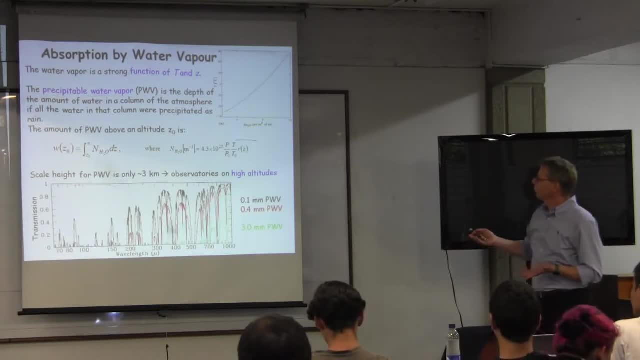 where the temperature is low, then you also have very low water vapor And it's actually called the reciprocal water vapor- And I always have to practice that word- Reciprocal water vapor And it's the amount of water essentially in a column. 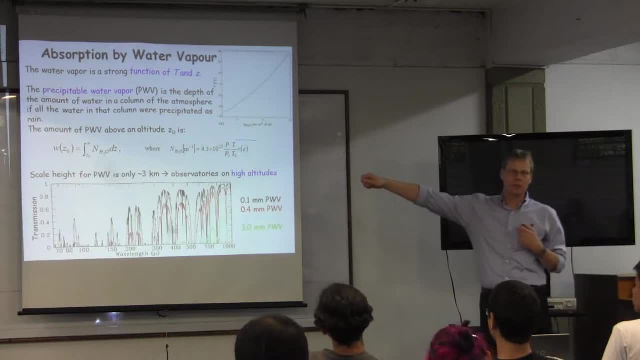 You look in a column and you just integrate along this column And then you have, if this were all sort of raining out, you could measure it. oh, it's about one millimeter of water altogether, But of course, in reality, 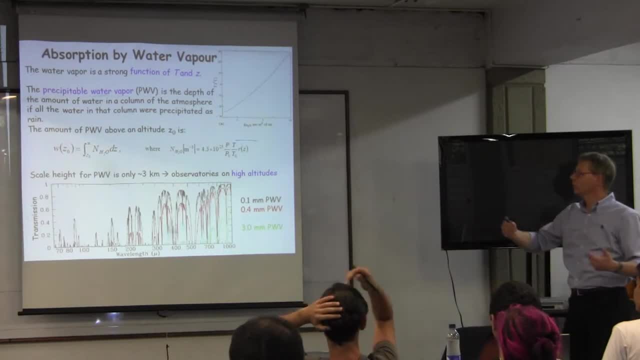 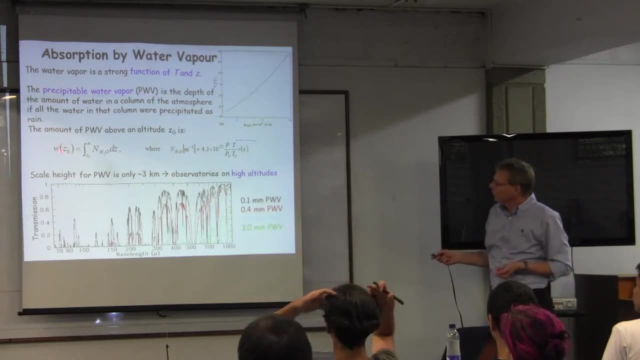 it's over kilometers dissolved as water vapor in the air And okay, so you just have to don't worry about this equation here. but so the water vapor is simply the integral from where you are to infinity, across all the water along the line of sight. 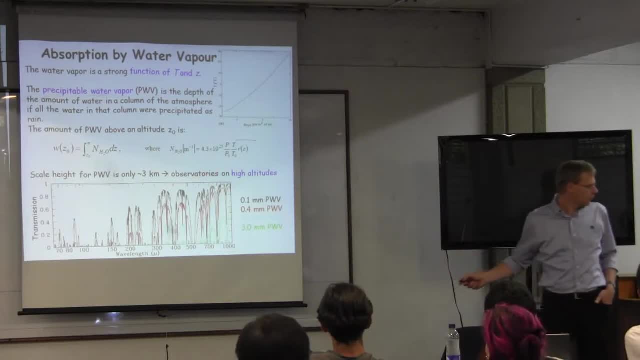 And it has an impact immediately. Sorry, Which is the units of this? zeta in the yes is meters or centimeters or millimeters. Zeta, Zeta, Zeta, Zeta. So this has grams, This has, so this is a gram. 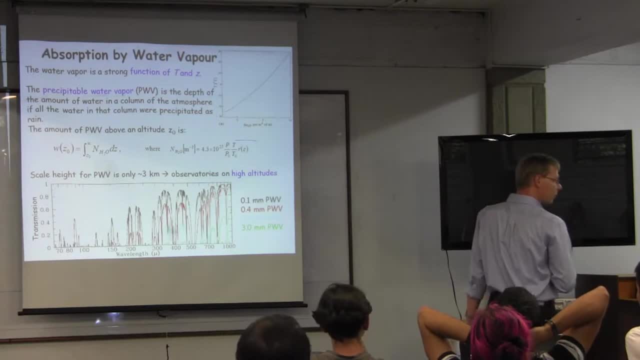 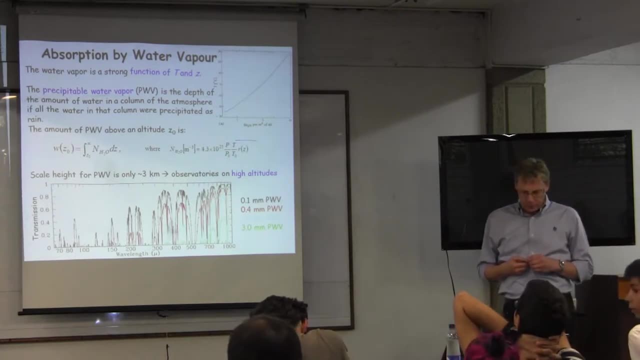 It's like a G. This is a G Grams of water. Grams, Grams of water per cubic meter. Okay, so this shows again the transmission for a longer wavelength. I think the optical will be here, So from 70 microliters. 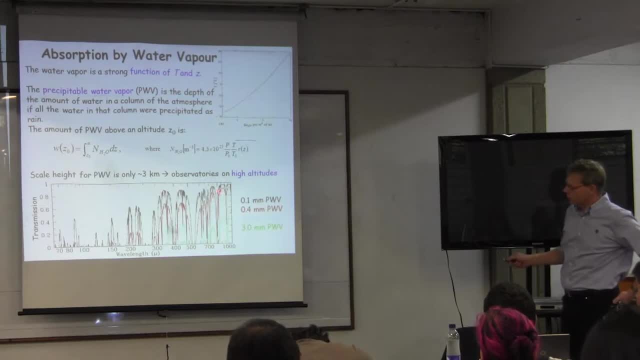 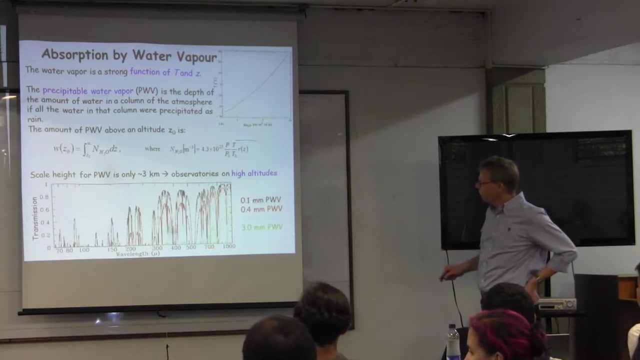 to 1000 micrometers. This is already the radio, this is the millimeter machine, the far infrared and the mid infrared. And the black line here shows you that if you had only 0.1 millimeter of water vapor, you would still have 80% transmission. 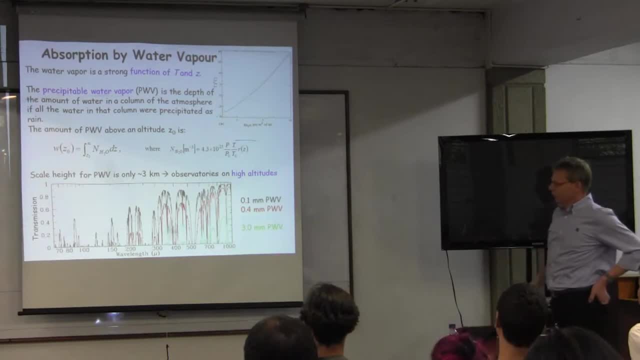 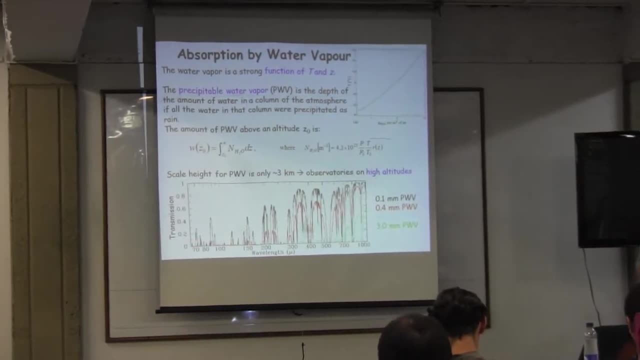 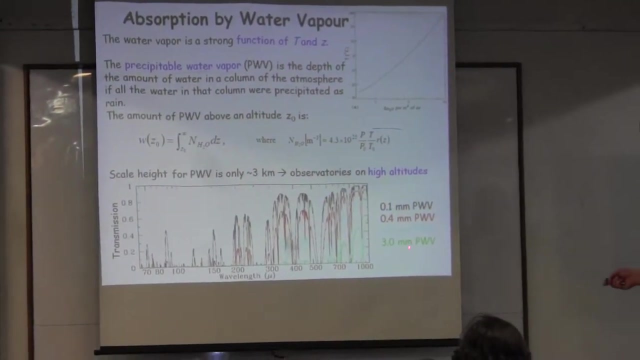 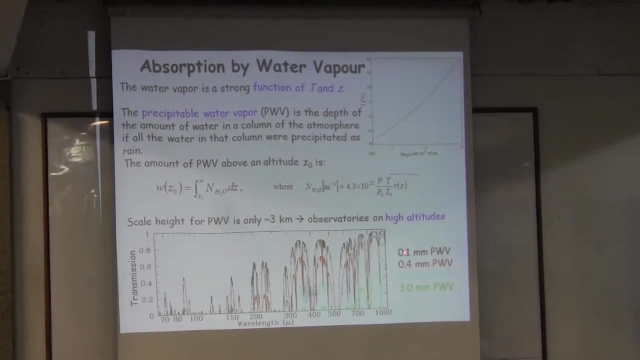 That's correct. If you had 3 millimeters of water vapor, well, this is the green curve here. well, you have 5% transmission. Forget it, Don't even waste your time on it Now. these numbers may not mean much to you, but 0.1 is exceptional. 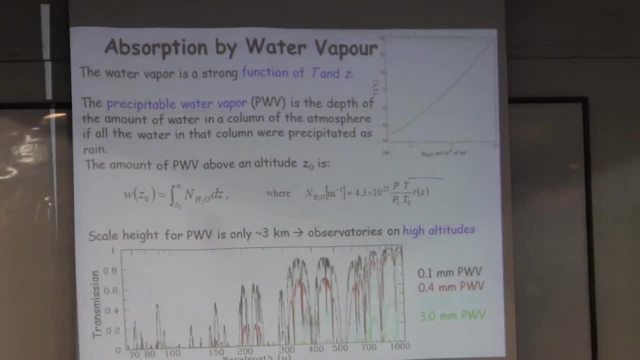 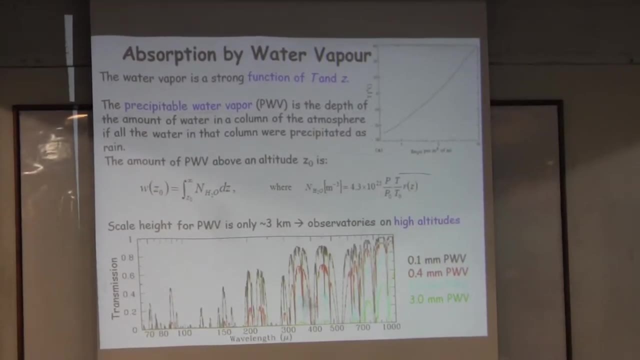 I think that the South Pole, where it's really cold, you have something like 0.2 millimeters. So people are planning observatories at the South Pole and that's one of the reasons: Because it's so cold there, the water with that vapor content is very small. 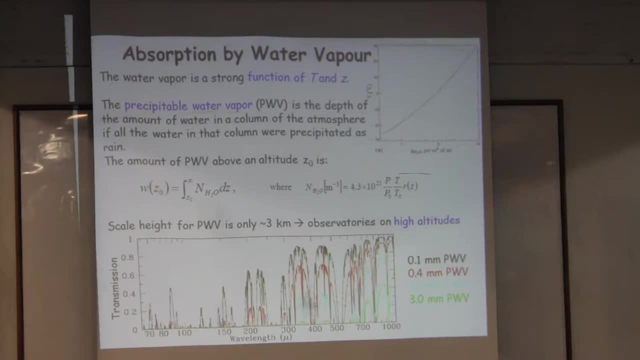 and it opens up all kinds of windows in wavelength space for observations. So for this AND function and a wire, do you measure or calculate that number? It's high data. This is something you can measure, Okay, And of course people making models of the atmosphere could also calculate it. 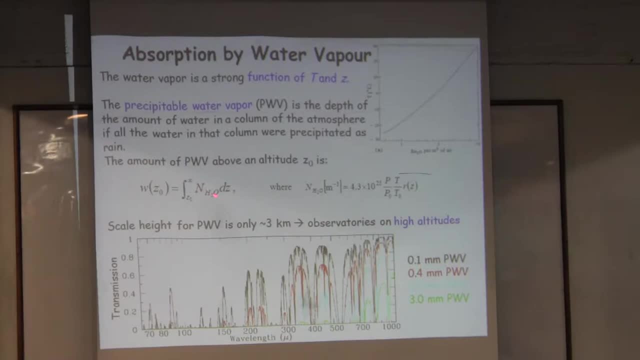 I think you need the model to then see how it's actually distributed, if it's not such a nice curve in reality. But I mean, usually we measure it and we assume it, But how do you measure the water vapor in the atmosphere? 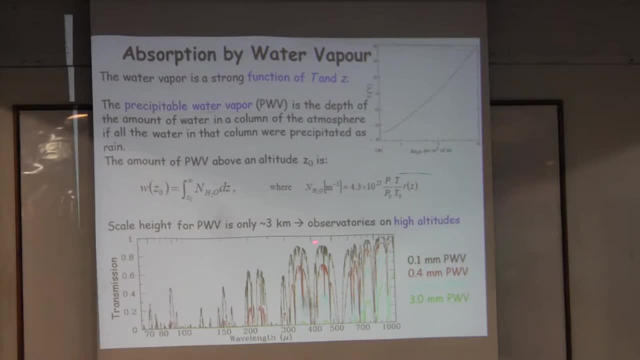 How do you measure it? Oh, you just look at. You know how the molecules are absorbing and you just measure the local known features to measure how far these are absorbed. So you make a differential measurement. I mean, let's say you look at the black body. 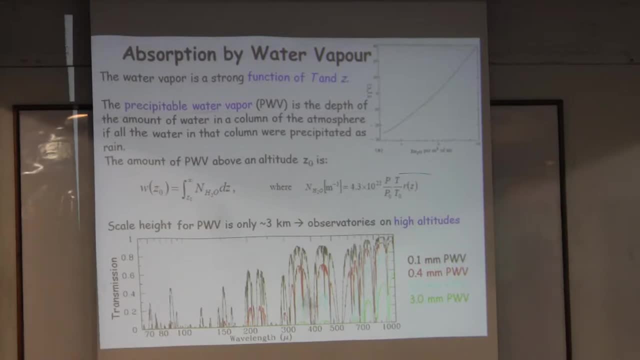 You have some continuum. You just need to look at the absorption At the light, at the absorbed wavelengths, and the light at the transmitted wavelengths, And the ratio tells you immediately what the reciprocal water vapor is. Now, if you go to dry regions in Chile where many modern observatories are being built, 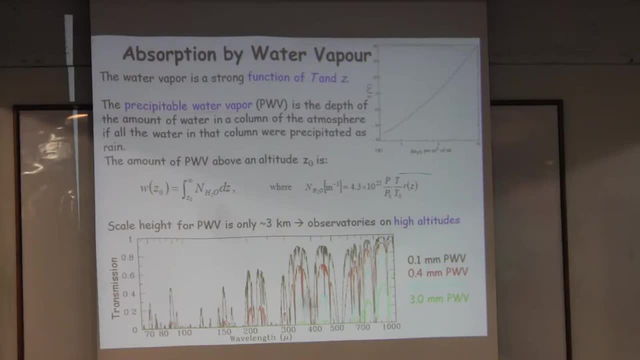 I think you have something like 26 millimeters. It's called driest place in the world. I mean there's a few clouds but it's warmer than at the South Pole. We have something say 0.5 millimeters, 0.6.. 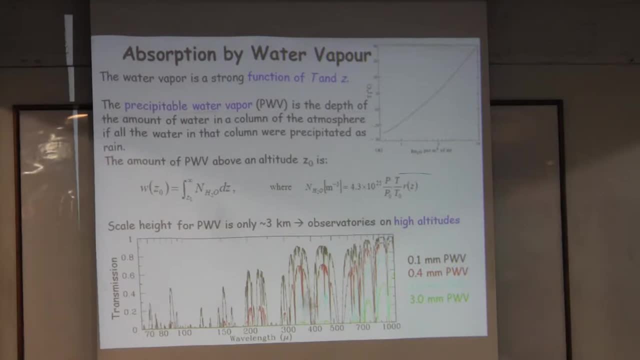 I think the green curve is more representative of light, And so we don't have any mid-dose probes there, apart from the radio, where this doesn't matter, And yeah, so it's very important to go for longer wavelengths to go up that very high mountain. 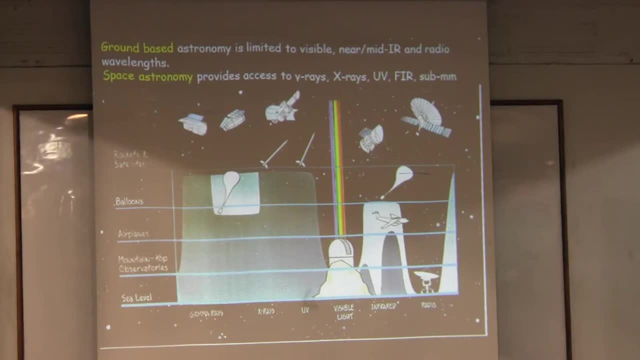 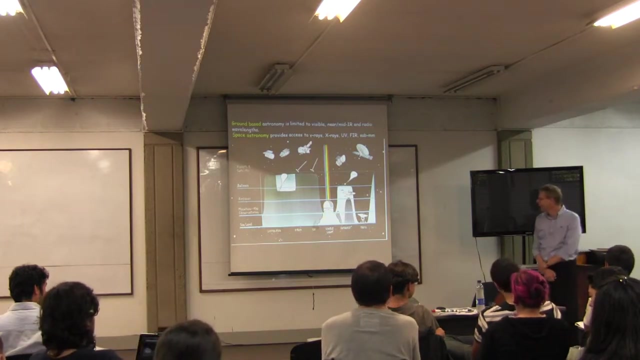 So I have this question: Why don't we build more telescopes on the Arctic or the Antarctic If it's so avoidable for it? which is the main reason: Cost and convenience. So far, the South Pole, Yeah Yeah. I think it's a good question. I mean you should look at the logistics of the South Pole. There is the human factor. Maybe it's a good training site for people who plan to fly to Mars. But I mean it's happier dark. 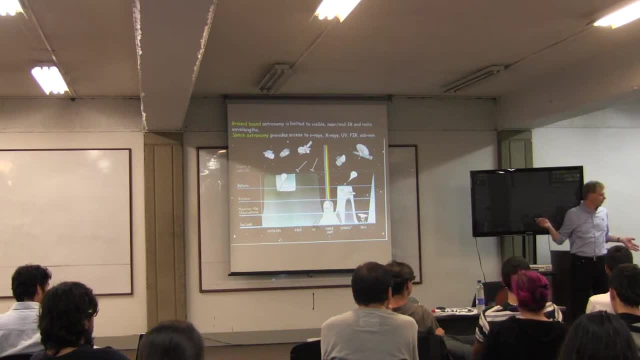 I mean observations are usually done during the winter. It's only one night, but it's a long night, And then the human factor is important. The human factor is important. so being surrounded by darkness for half a year and just some crazy colleagues is typical. 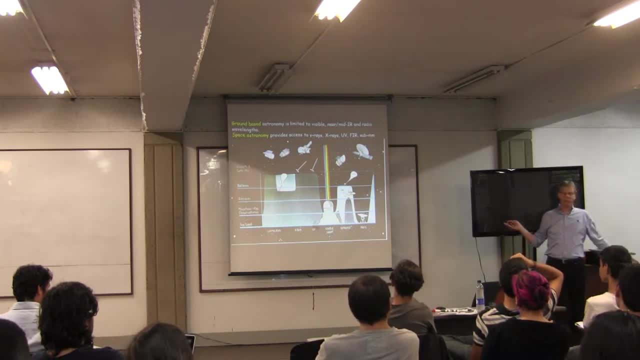 Operating here is also typical. I mean you have the great temperatures and low temperatures. I mean I'll give you one simple example. You have to work outside. You take a drill machine with a power cord and you have two minutes to make your drill your hole. 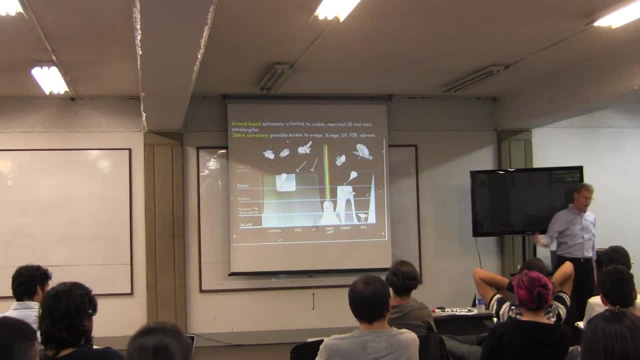 And you have to run because otherwise the cord gets frozen and you'll never get it back in. So this is just one example, I mean from everything else- restrooms. it's expensive to ship all the equipment here. It's cheaper than to space, but it's very expensive. 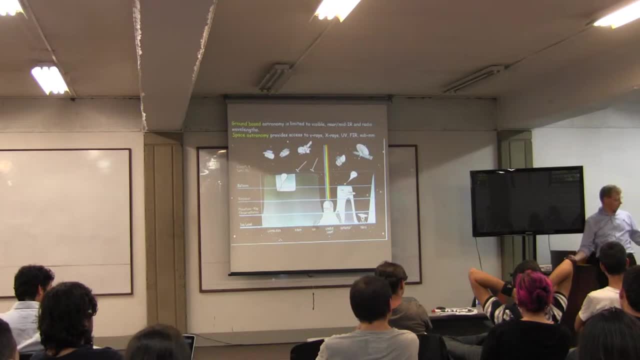 And then you don't have a power cord, You have a perfect solid surface, Because the bigger you make the toes, the more weight there is and it sinks into the permanent ice. So does your hotel. if you build one right, After 10 years it's under the snow or the ice. 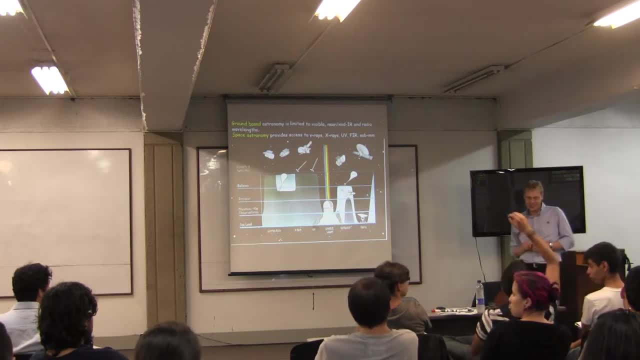 So there are problems. Excuse me, what about a kind of robotic telescope, Something like that, right, Yeah, Well, what is it? I mean, there are robotic telescopes all around the world that simply save the cost for the people operating. Because you don't have to send someone. The problem is they're not foolproof. The reason why space astronomy is so expensive is that you have redundant mechanisms for everything. You have everything tested for years before it gets launched. Nice, You have robotic telescopes. 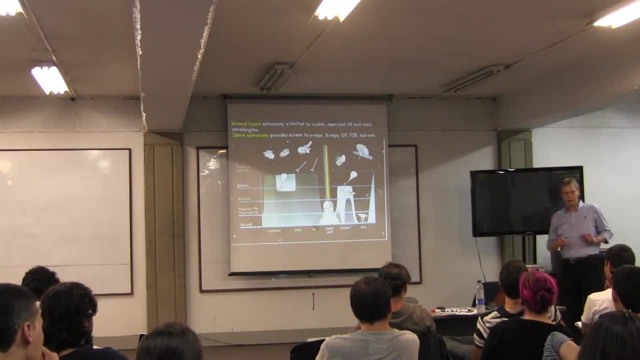 You just put a motor there and you assume it's working. Now, if you ship through a robotic telescope that was built in that way to the South Pole, I can guarantee that it will fail during the first night. Something will break and it was not considered properly. 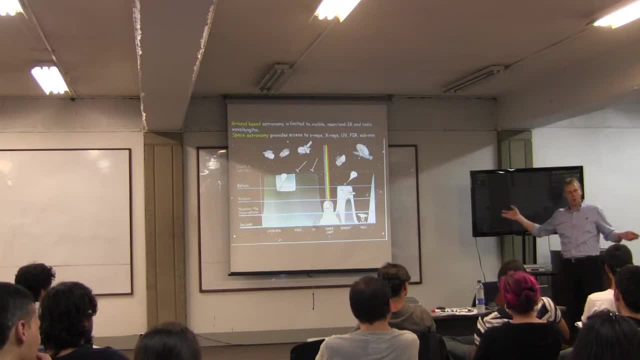 And then you need people to repair it, And so you don't have, Or you make it like space, and then you have your observatory at the South Pole, and it costs $5 billion, And who's going to pay for it? Space has at least the advantage that you 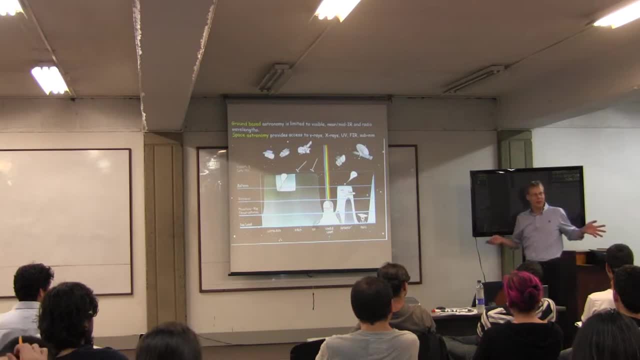 I mean you can excite the public. You say, oh, that's a space mission and we sent astronauts there, And politicians like the idea that the South Pole is too far away To spend a lot of money, A lot of money. 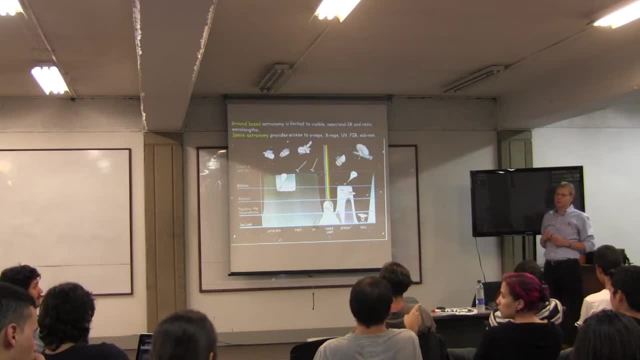 But I know a lot of A few projects of To To establish robotic telescopes in the South Pole. In fact I was in Argentina last year And my advisor is working on a project to install a little telescope in the Argentina part. 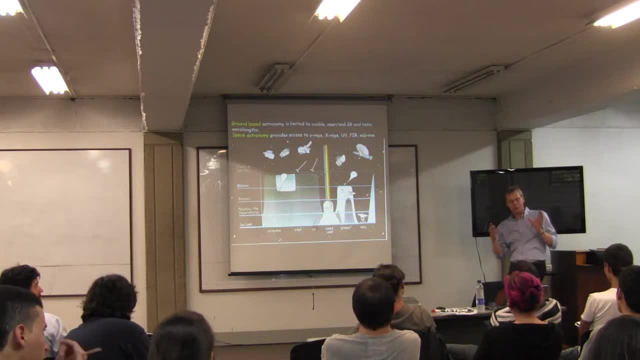 Yeah, no, That works. Good point, But they're small telescopes. Yes, It's proven technology, But of course the idea would be that you move the 8-meter telescope from somewhere here, maybe Hawaii, to the South Pole. 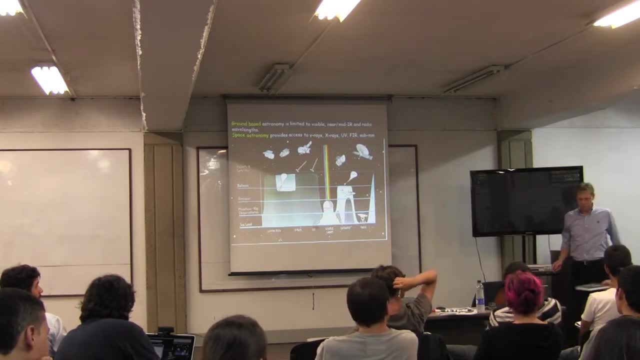 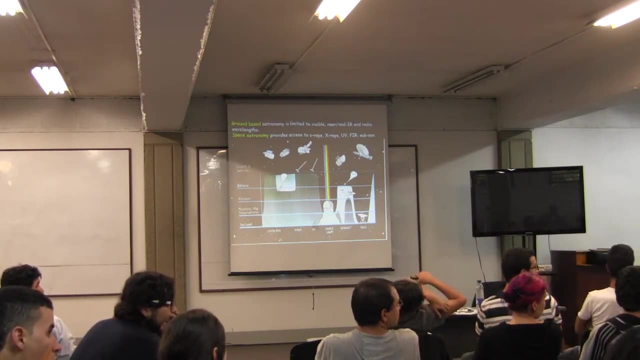 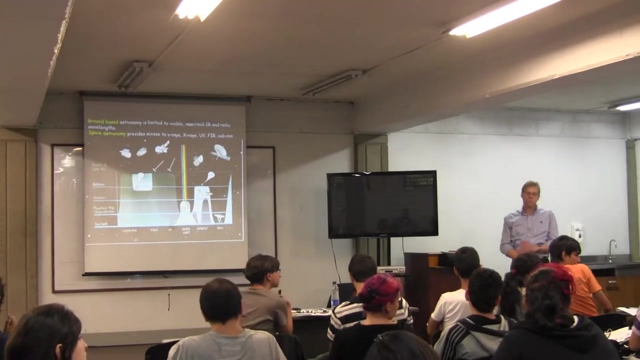 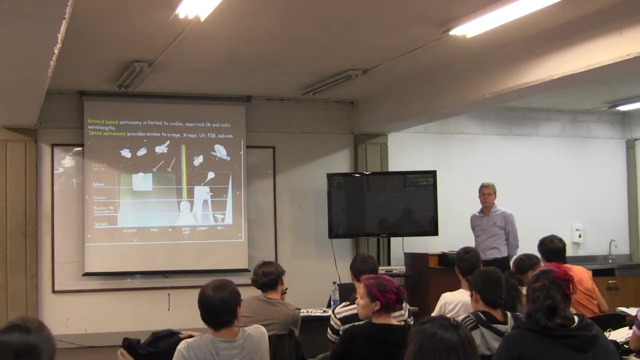 And then the problems start. Yeah, There was another question. Yes, That's That's another. Yes, Yes, That's another good reason. Yeah, And it's. It's important also that, Well, actually the southern part of the sky is. 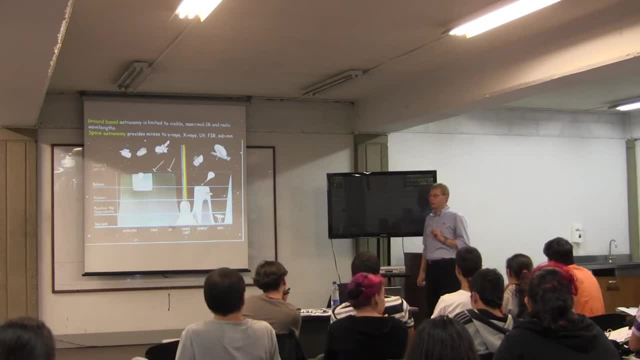 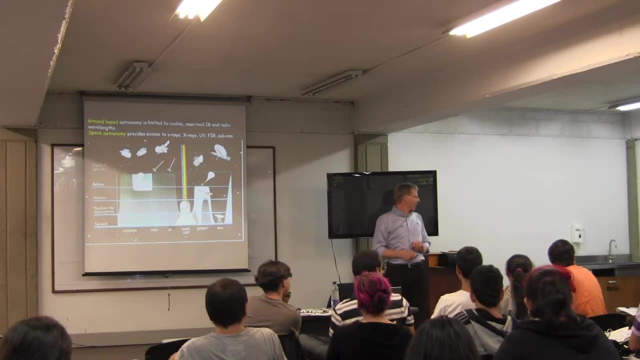 Is the better one. So we are closer. Yeah, It's fine, Yeah Well, But I mean the big ALMA, for example, is on the southern hemisphere, And so many Yeah, Yeah. 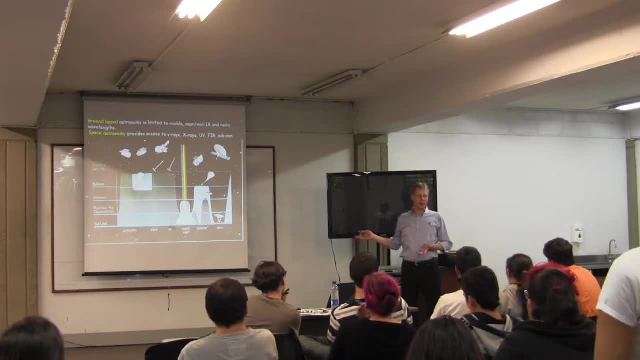 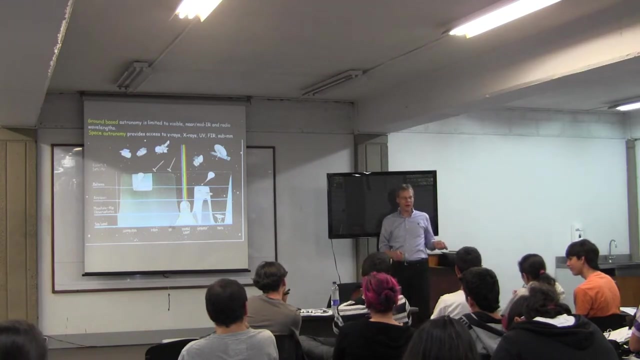 Yeah, Yeah, Yeah, Yeah, And so we have much more information And so many many survey projects. I mean, nowadays you have the big discoveries by buying, often by compare, by combining different wavelengths, radio observation, if you combine them with Hubble data and so on, then by looking, 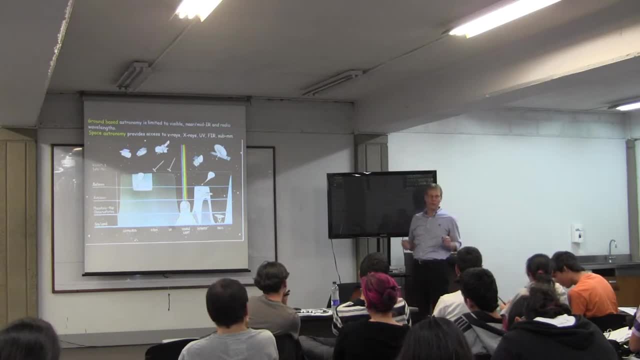 at the All the wavelengths. this is where you find something new about objects. And that, of course, requires that you can- I mean you are able- to combine your radio data. This is where you find. This is where you find something new about objects. 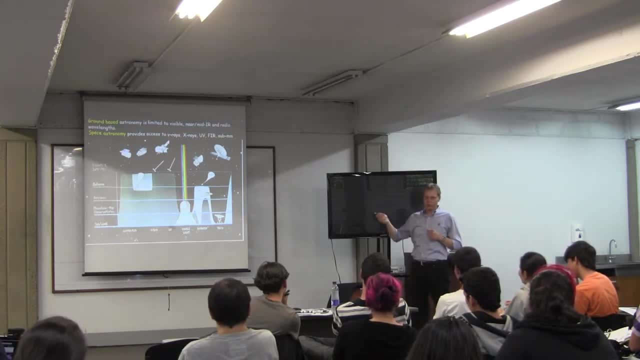 And that, of course, requires that you can- I mean, in order to be able to combine your radio data, you need to have the same objects, the same hemisphere. that was one of the reasons why ESOL said the ELT has to be in the 1000 meters. we have invested lots of money in ALMA and in the VLT. we have all the data. if we don't start on the northern hemisphere then we have to start from scratch building up data bases. this is a NASA cartoon that shows that in the visible you can do it from a mountaintop. 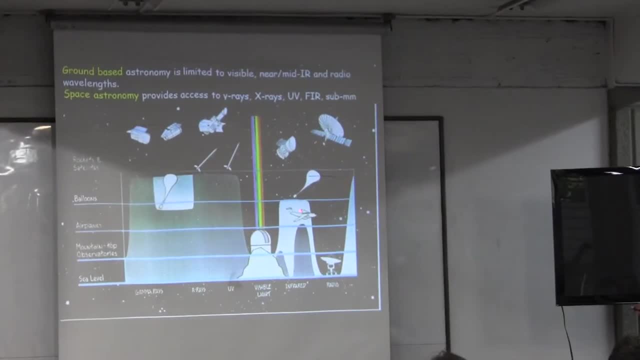 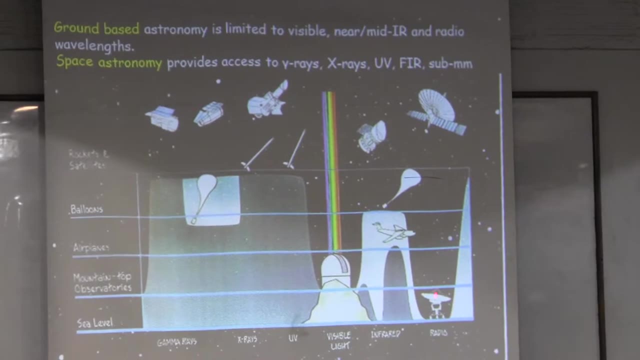 but if you go to infrared you need an iron mountain, or you take an airplane or you go to space, maybe a balloon. the radio is nice, the radio is on the ground and we know that the atmosphere is transparent by radio waves. 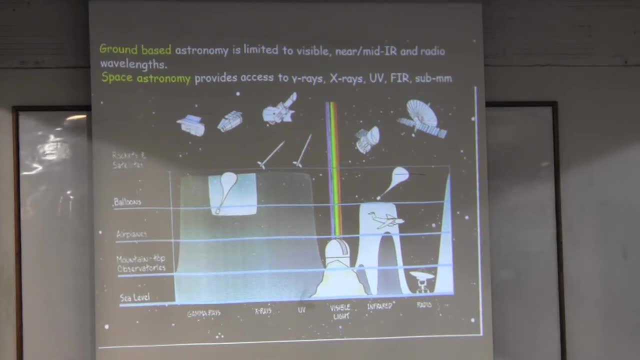 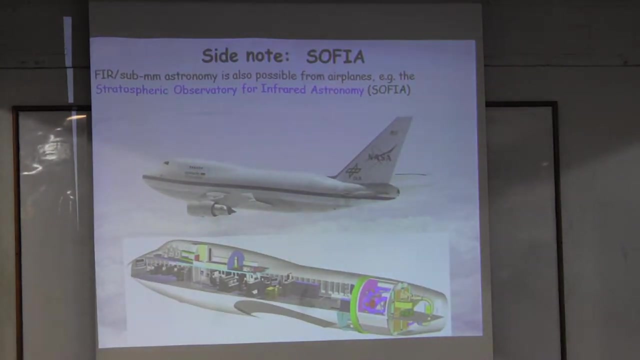 and we know that every time we turn on the radio. but then if you go to the UV X-rays, that's actually quite unfortunate that the atmospheres will take the X-rays and the arrays, but that means you really have to launch the satellite. there's one example for an infrared observatory called SOFIA, the Stratosphere Observatory for Infrared Astronomy. 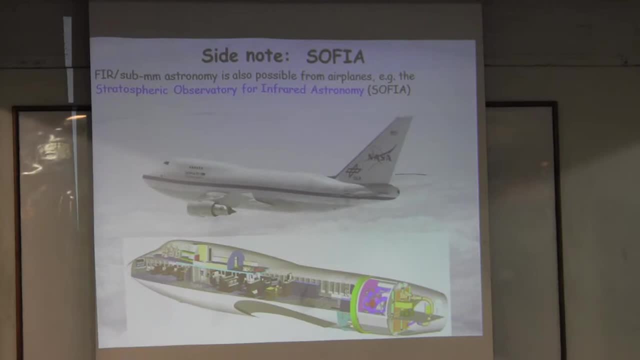 where they have taken an old Boeing 747, cut a hole here in the back with a drill and the door that slides off put in a 2.5 meter telescope and so you fly at- I'm not even sure- 14 kilometers, 15 kilometers high. 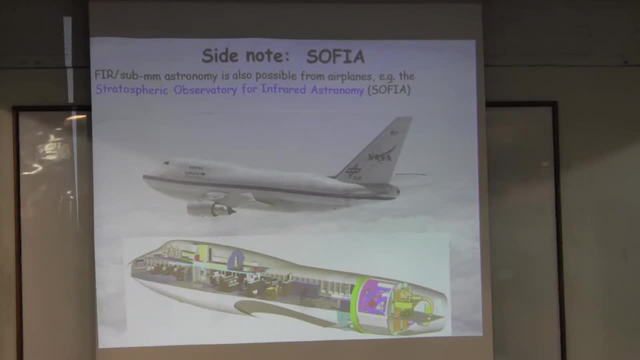 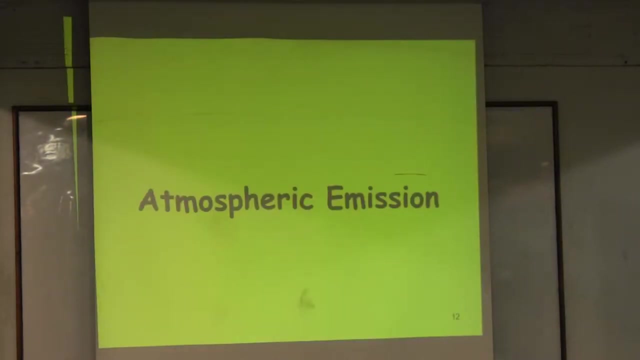 and then you fly around, take off in currently California or maybe Hawaii, and then you fly around and, of course, in this case it's easy to select your objects. you tell the pilot to turn around and yeah, ok, so that was the absorption. 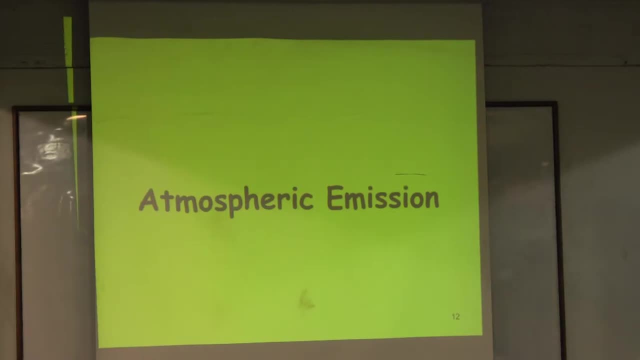 but the atmosphere is also emitted and there are two types of emission. there is the fluorescent emission and the thermal emission. I already mentioned the fluorescent emission when we talked about ions in the atmosphere, ions in the ionosphere, essentially. so you have the UV photons from the sun. 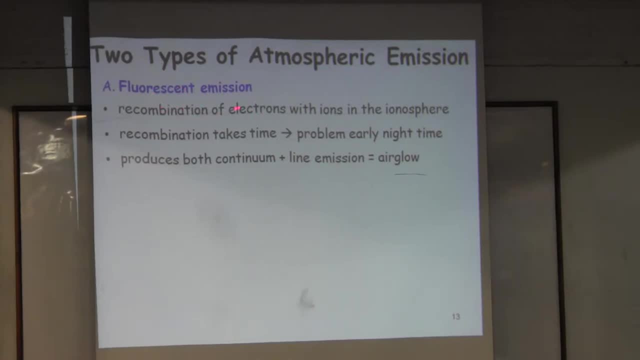 ionizing the atoms in the atmosphere, in the upper layers they recombine, but not very fast, so the recombination takes time. now, of course, that problem goes away to some extent during the night because, well I said, the UV photons come from the sun. 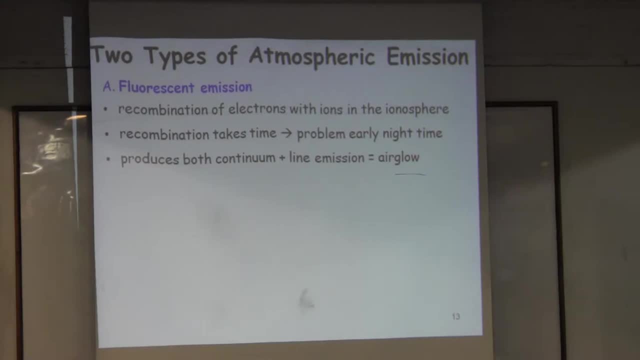 and you observe during the night because there is no sun. but since it takes a couple of hours for the ions to recombine, you will have a much stronger fluorescent background in the early part of the night in your observatory than in the later part of the night. 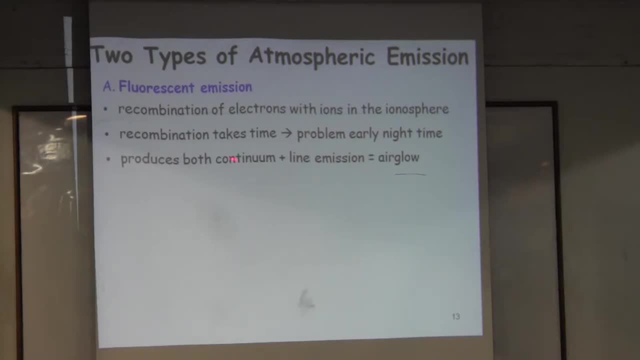 actually it's quite nice and warm. so these ions produce both continuum emission and line emission, but altogether it's called the antler. so that's sort of a sort of the sky is not dark, it glows brightly and mostly in a short wavelength, and then there is the thermal emission. 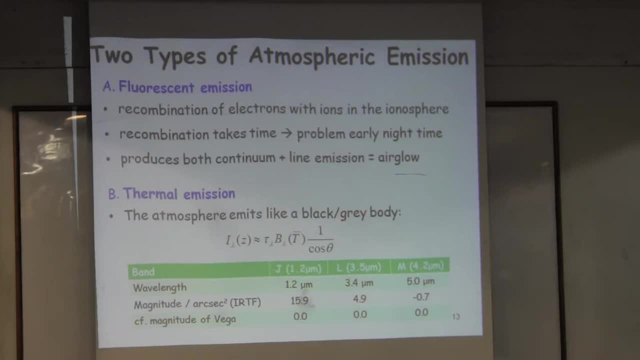 we just assume that the atmosphere emits like a black or a grey body- and I think Helena will get back to black body emission in her lecture later this week. so the intensity is simply a black body function times, the times, the factor here, and anyone who hasn't got here. what does this stand for? 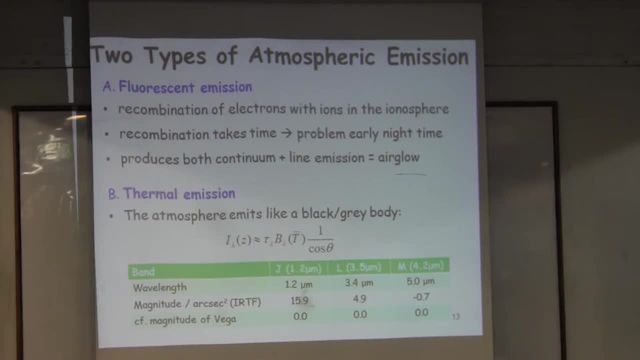 alright. so what's theta? lambda refraction, yellow refraction? no, not quite. this is a simple, very simple geometry of 1 in the year. it's simply the Theta cycle, because what counts here is, of course, the more atmosphere you see, the more emission you see. 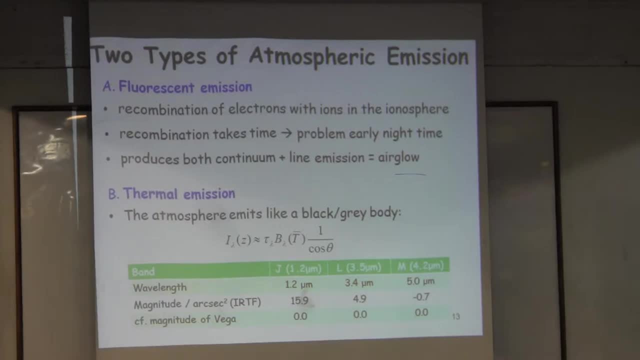 if you look up through a Theta and Theta you only look through one atmosphere. if you look close to the horizon right, the length through the atmosphere becomes a lot longer. and plane parallel atmosphere, plane parallel. yes, ok, and just to show you, I thought I'll calculate some numbers for you. 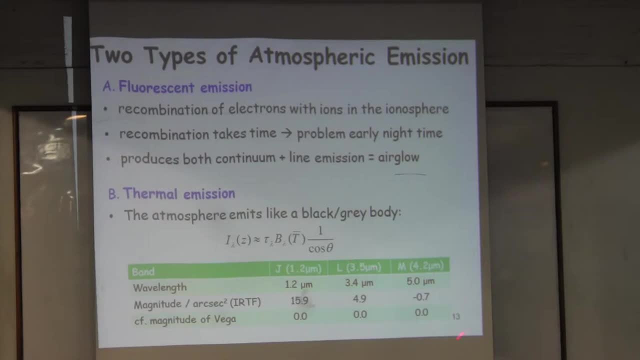 this is the Theta-Helian-Inferior wavelength: 1 micron, 3 microns, 4 microns- I'm not sure why I listed that twice, but this is the magnitude per square arc second. I think you're familiar with magnitudes: the magnitude per square arc second. 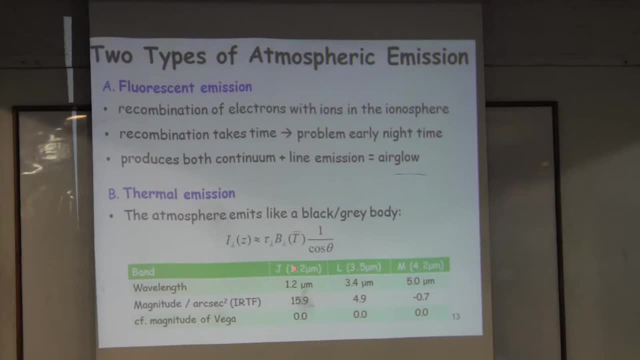 and the telescope. so in 1 micron the thermal emission is fairly small, probably 16 microns. but what does IELTS? oh sorry, that was measured with the infrared telescope facility, which belongs to NASA. this is not my idea, alright, but you can ignore that. 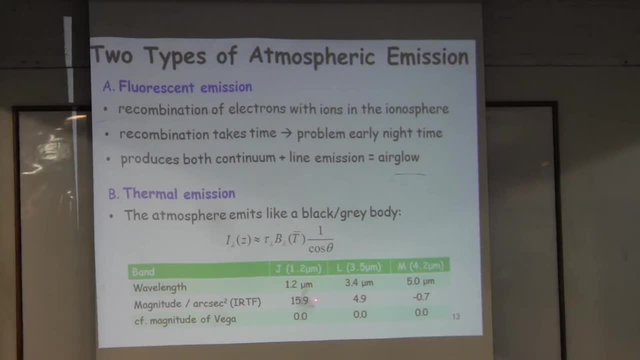 the main point is here that the thermal emission gets much stronger when you go to lower wavelengths. in fact, when you observe at 4 microns, you can see that the sky brightness is brighter than the magnitude of Vega, which is the magnitude of zero magnitude. right, that's like. 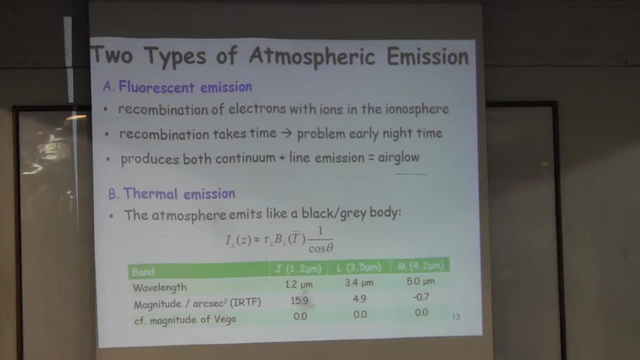 so, if you, because of that background, because the atmosphere radiates at longer wavelengths, this is almost like like observing during the day. right, this is mid infrared observations are like daytime optical observations. the sky is so bright, brighter than the stars, and so this is, of course, very 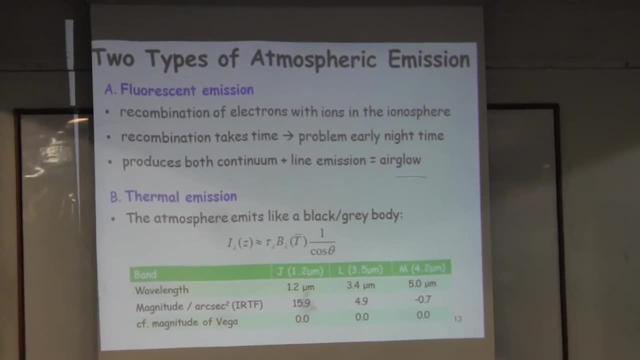 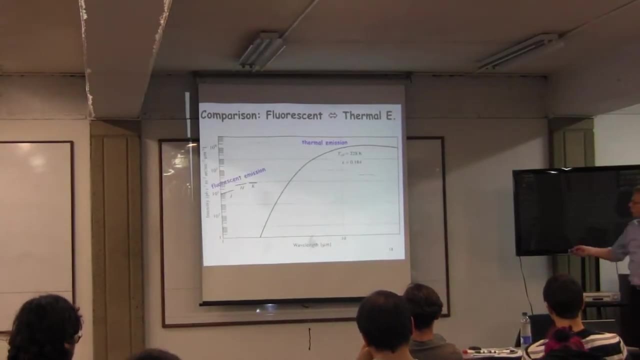 you can still do it, but you have to have a way to subtract the background, to calibrate that out right, and we can. we can just compare here. this is the intensity. I hope the units agree with what Willem has said at this earlier stage, but the intensity is a function. 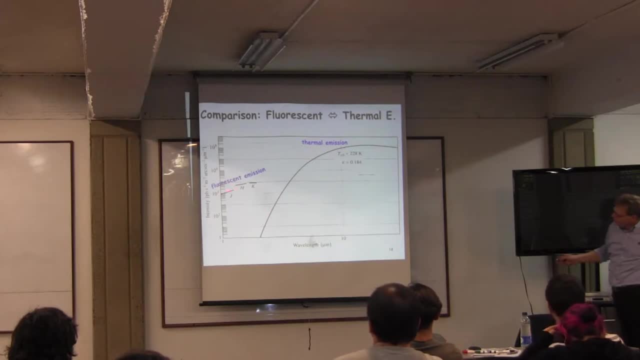 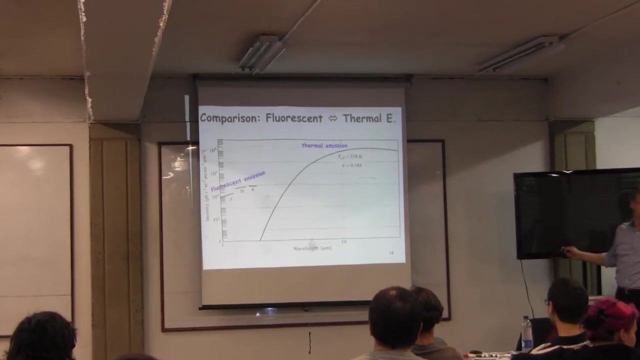 of wavelengths here for the near infrared lens, GHK, so it's 1.2, 1.6, 2.2 micrometers, and then you have the thermal emission here and you can- I mean this is one you should be able- to recognize the shape of the black line. 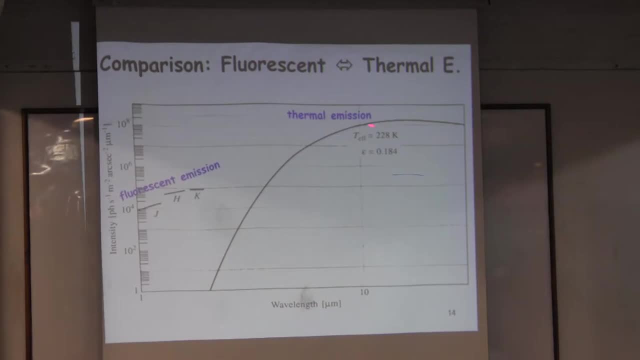 right, so this is really for a, in this case an effective temperature of about 230 Kelvin, with a with a small emissivity, but it dominates the background entirely in a longer way. alright, sorry, yes, do you know that an effective temperature is just an average, or? 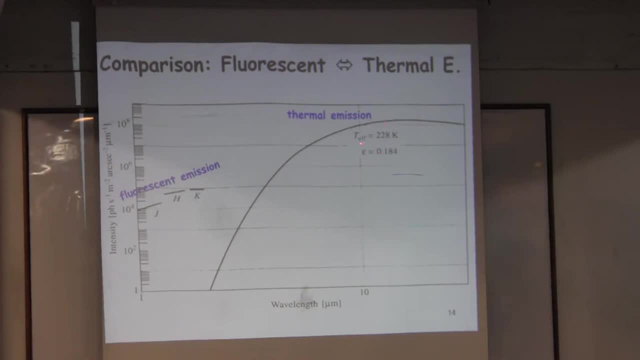 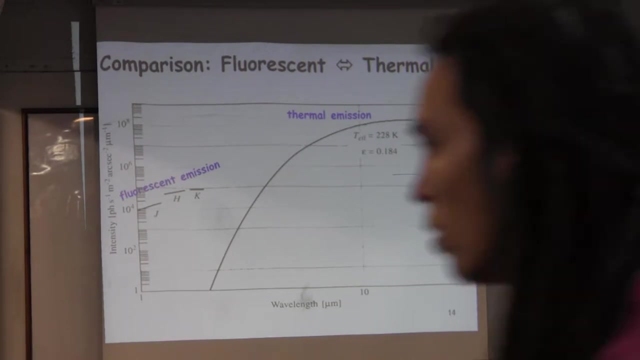 it's well. well, yeah, I mean you could calculate it and measure it. but you could, I mean you can. there are various ways to do it. but you could also just observe at different wave banks bands and assume it's a black body and see, okay, and this was just. 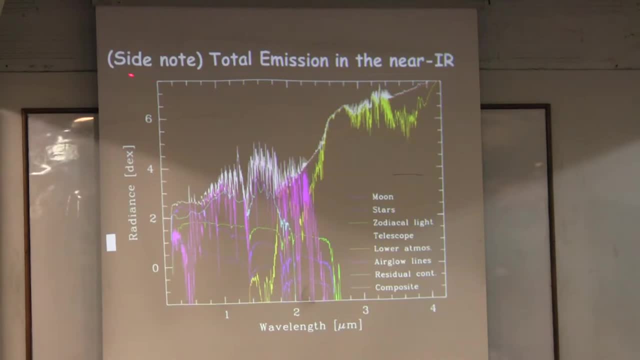 I mean you will find in the lecture a couple of times things like that are in brackets or labeled side nodes. so this is more as a background information for you that you might, might ignore or look up it's, it's or it's- just to understand the risk better. 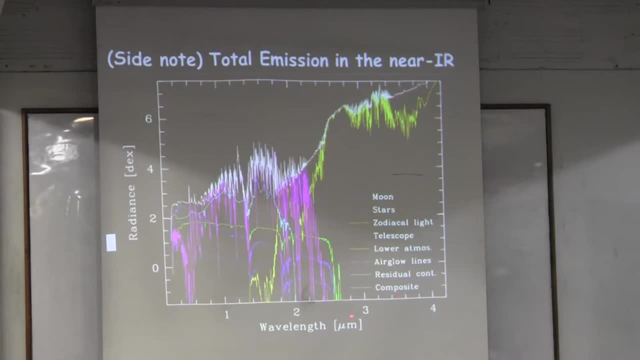 this one is additional information, just to show you how complex things are. if you would take a spectrum- I don't know it's gradients, but it doesn't really, it doesn't actually matter. just say that this is the, the brightness of the background as a function of wave lengths. 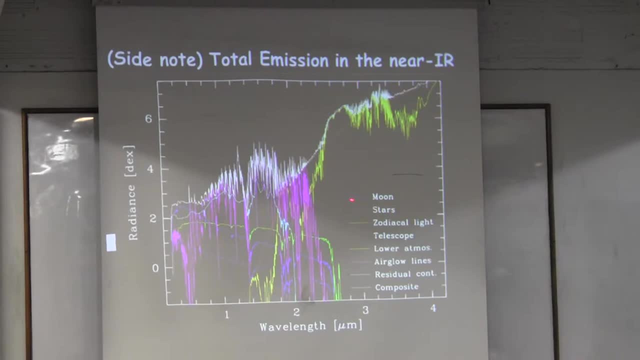 and here you see the individual components: from from the moon, which is always what can can be the problem of the sky, or the clouds, or the background from other stars, which is faint. so diacolite, telescope emission, lower atmosphere airflow, so this is the fluorescent emission. 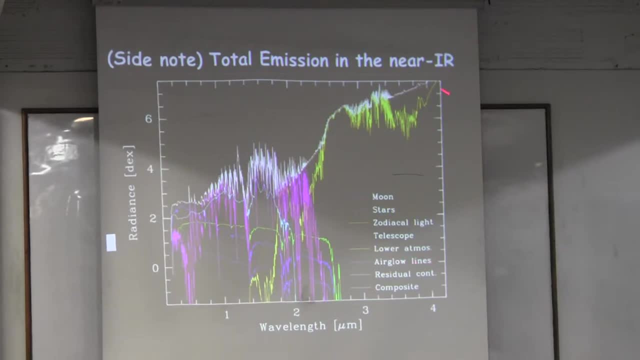 and and then if you put this all together, I mean you have a very complex structure over here. it's very complex and you have no astronomical source in there yet, so you have to calibrate for that. of course you have to subtract that out in order before you can publish. 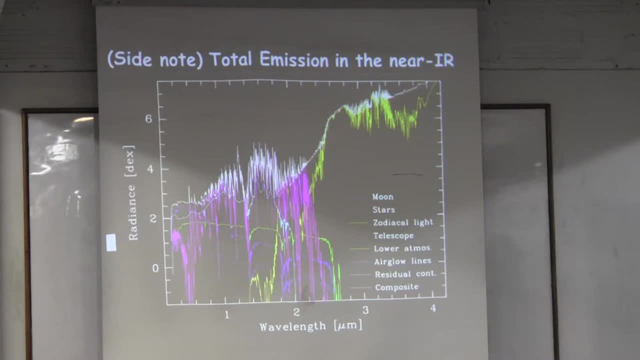 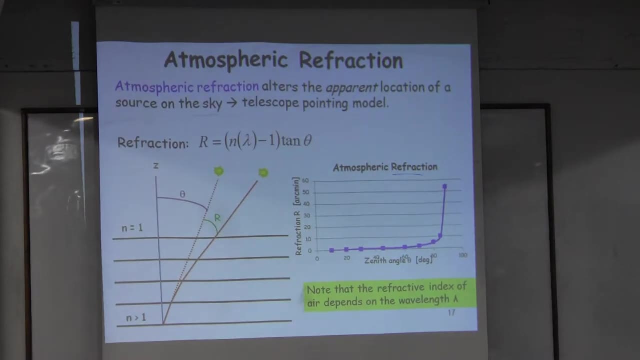 the spectrum of your galaxy. okay, and then we have a few more. there is the, the atmospheric refresh, and I think- yeah, I think a lot of people know about it- who has a, a small telescope, or have a look through it or operate it? you do it. you never told me that. 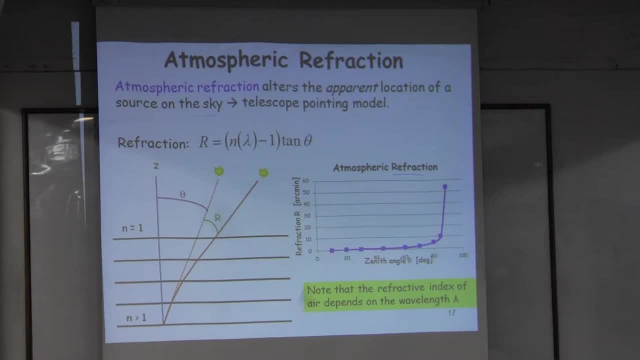 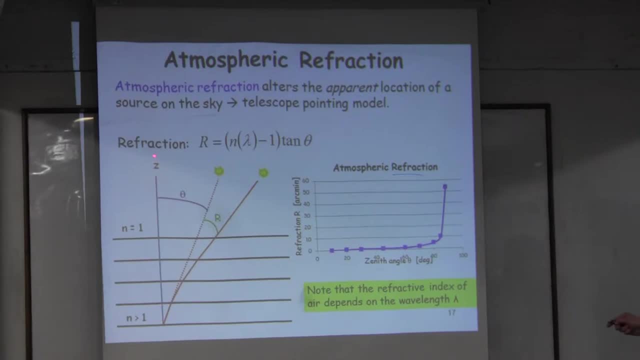 and, and, and. then we are. so this here, here. but there is something, this, this comes from which I my than 1.0, and 1.0 would be vacuum. So if we were all, if all the Earth, if we would do this on the moon, let's say, without an atmosphere. 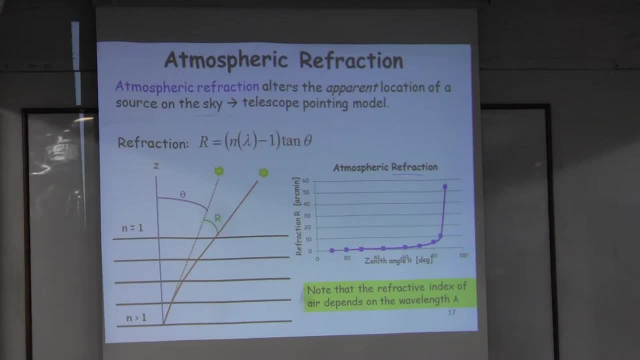 this would not be an effect. But since we have an atmosphere that's getting denser and denser as we get closer to the surface of the Earth, the light is bent actually here. So there is an angle between here and here. Of course, this is idealized, right. 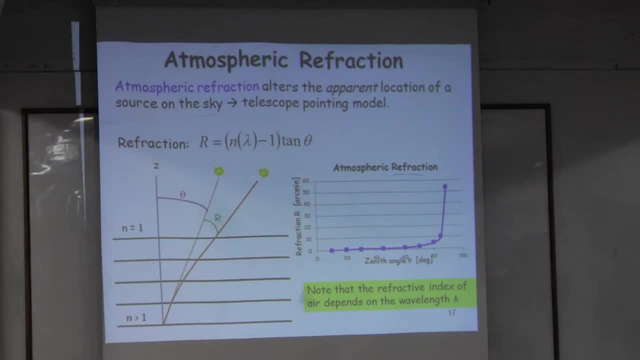 So we just have an atmosphere that consists of five layers. In reality, this is a smooth gradient, but I think you get the idea. So the light it's like. assume this is like a lake, right, The light travels in here, but then the light will be bent. 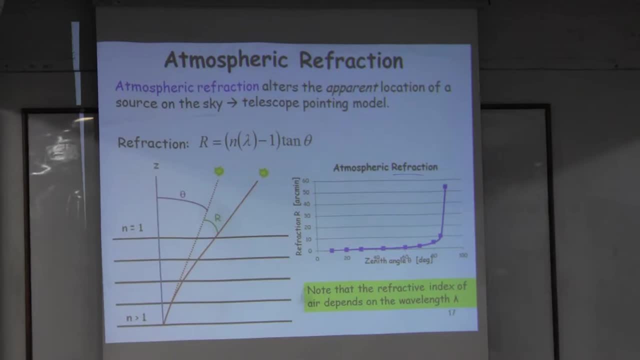 and the ray is under a different angle, right. That's why it's difficult to whatever catch it. Don't catch fish in your swimming pool, And so the light gets bent. so it's a different angle here and here and here. 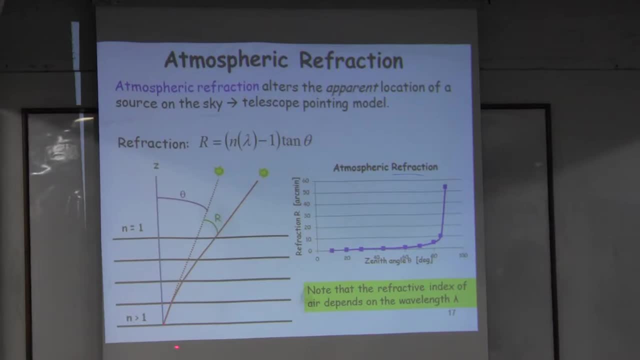 And then, finally, this is the direction where it reaches us, And if we sit here and look up on the sky, we see this direction, And this direction, of course, follows, seen from here, follows the dotted line Right, So the star appears to be here. 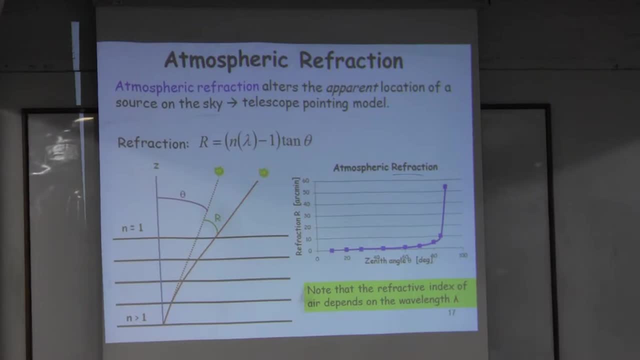 while in reality it's here And this oops- sorry, this is highly lonely here Because of this tangential theta function. So the refraction r, meaning the angle here, the offset between the true and the apparent source position on the sky. 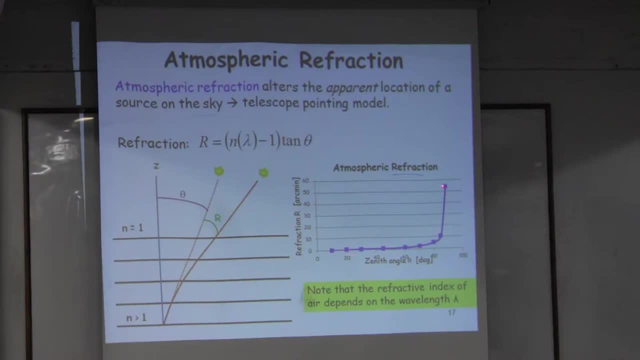 since it's multiplied with that factor, it increases. the refraction increases dramatically with large angles. So you can see here large arc minutes. actually it's so small that it's hardly noticeable here. If you just look at 10 degrees in distance then you would not, at least with a small telescope with large field of view. 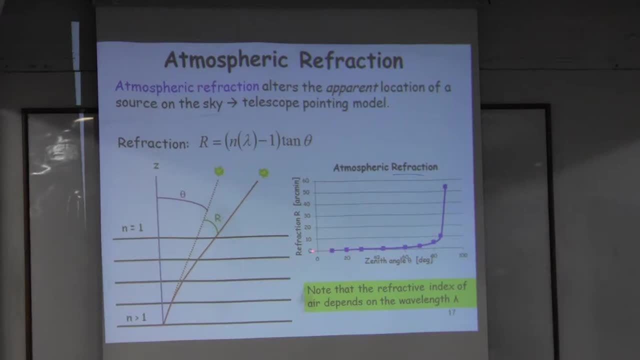 you'll always see the source. It may not be exactly where you expected it, But when you look at something at the horizon, well, it can be 50 arc minutes, but it's almost one degree, So larger than in fact it can be larger than the diameter of the full moon. 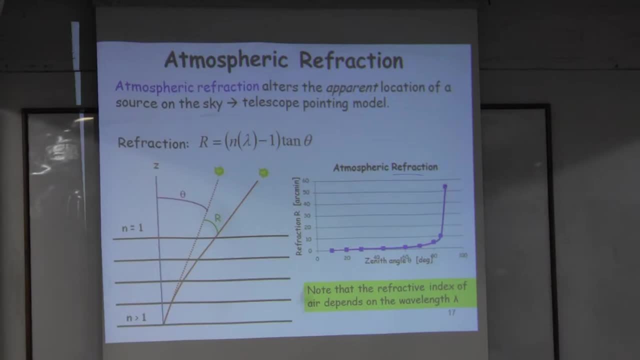 And yeah, this is, of course, important to know about, because big telescopes usually have small fields of view. So if you don't know about this and you point your telescope, you will not see your source because it's somewhere else. 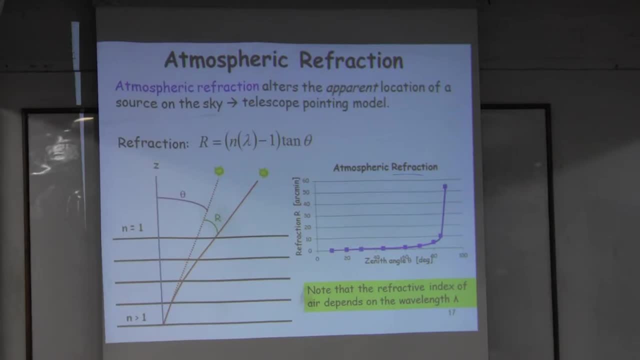 But the good thing is that of course most telescopes are. You know about this. This is a very simple mathematical form. So you tell your telescope computer and it knows. OK, I go to 60 degrees, 16th of a distance. 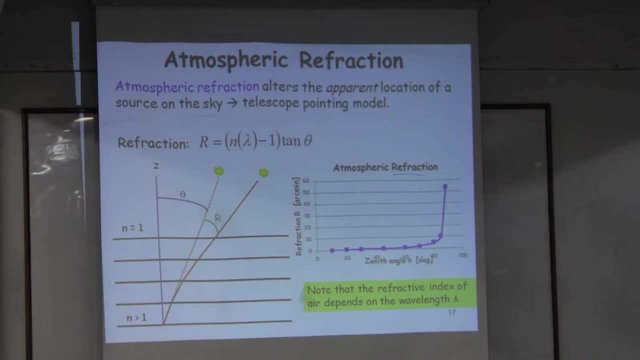 so actually I have to go to whatever: 16,, 1 or 7 or OK. So this is the atmospheric refraction. It's a large effect but it's easy to take out. However, note that the refractive index of the air 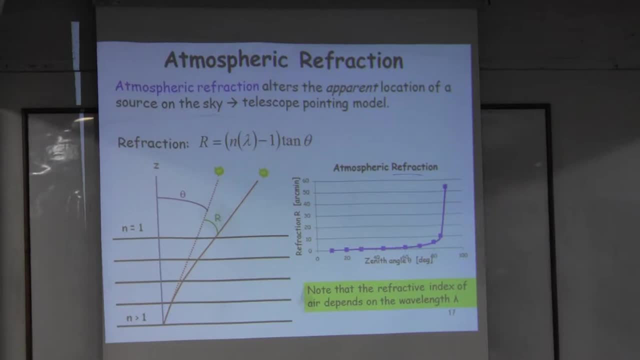 like the refractive index of most materials- glass or some crystal or liquids or gases- is not constant with wavelengths, but it changes with wavelengths, meaning that this effect with wavelengths depends. So depending on your observing wavelengths, it may be closer here or here. 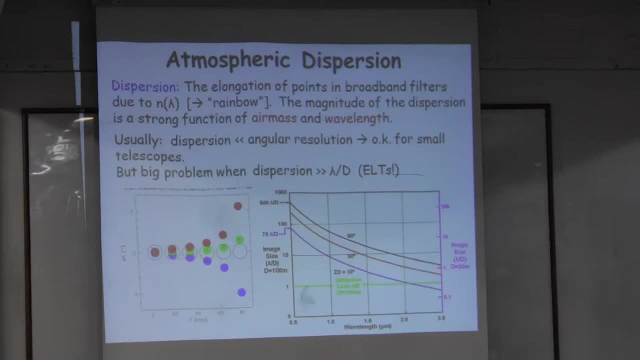 And it's a small effect And the effect is well, let's say, the effect is tiny. If you have a backyard telescope, it doesn't worry about this, But what it does, and this is shown here. so if you, 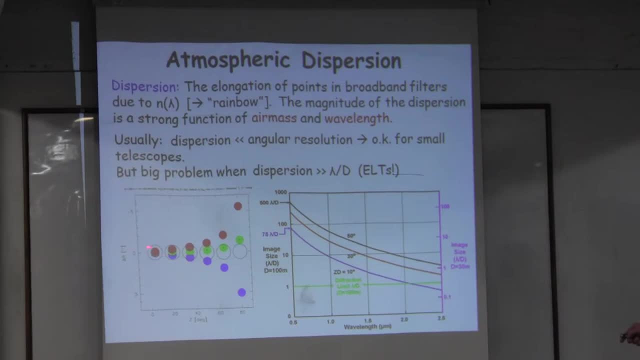 because it's wavelength dependent. if you observe at zenith, the red light and the green light and the blue light of your star overlap. they are focused on the same spot. If you go to higher zenith angles, because of this dispersion of the atmosphere, 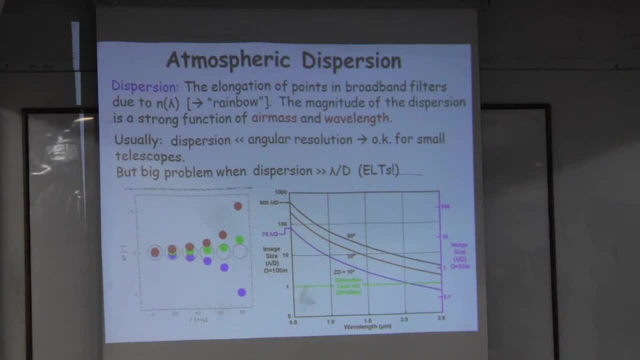 you will see that the red light is actually at a different position than the green and the blue one, And I'm mentioning this here although it may for most telescopes not be relevant. but if you go to for the next generation of large telescopes, 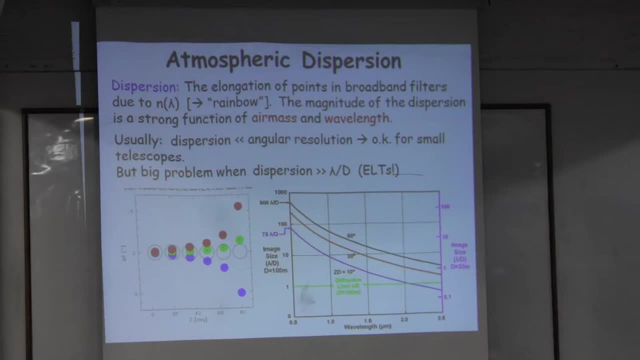 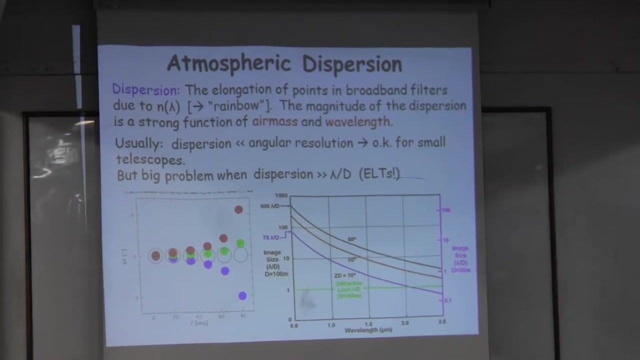 bigger than 10 meters. this will be a problem In the sense that the sources will be really elevated like a rainbow, much larger than the resolution or the size of your, the diffraction that you did, size of your star And well. 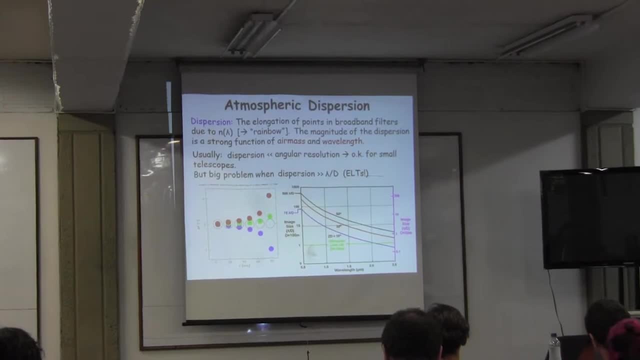 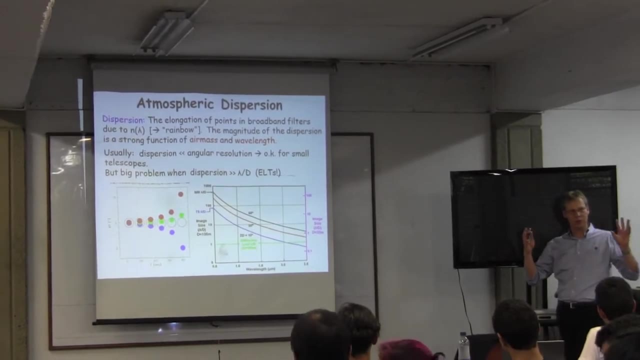 astrometry is becoming a very. I'm always surprised, because astrometry I mean just to record and study the positions of objects on the sky. whereas it was a big topic some 50 years ago, and it still is, it becomes more and more important. 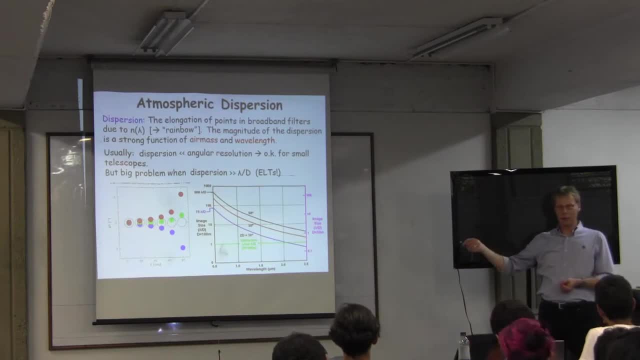 because with proper motions Elena will actually discuss that in her public talk on Tuesday next week when she talks about galactic center. So measuring the positions and even how they change with time tells you about the dynamics of the system. So you can look at the star cluster. 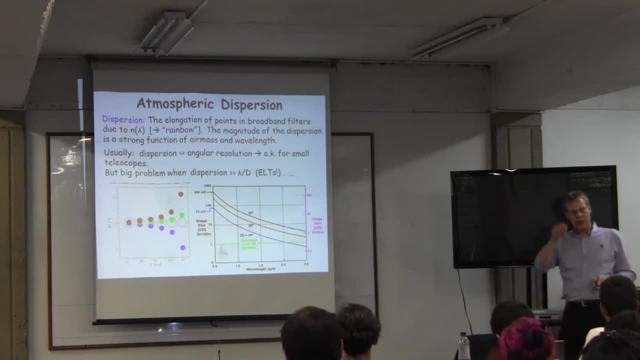 you observe it now, you observe it again in two years, and then you may have seen the stars move, And from that motion you know something about the gravitational potential in the cluster, You know how much mass there is, And, for example, 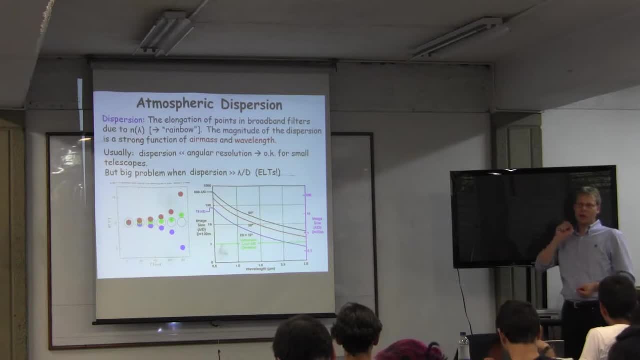 there are many more cases where you really would like to know exactly the position of the sources. The problem is that the stars are far away and they move a really tiny, tiny, tiny bit. So when we say tiny, I mean something like 50 micro arc seconds. 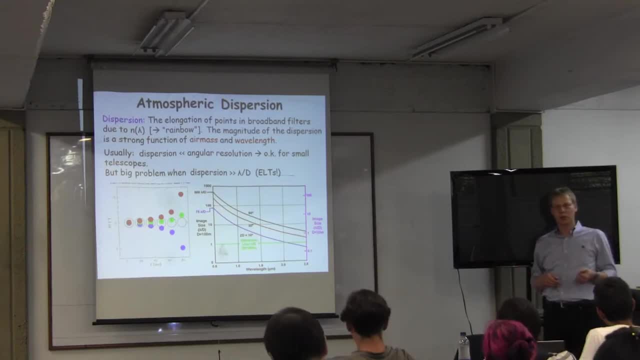 And arc seconds. that's what you get through the atmosphere of the regular star cluster. If you use the Hubble Space Telescope, you may get to 50 milli arc seconds. But now we talk about knowing about the source. position affects a thousand better. 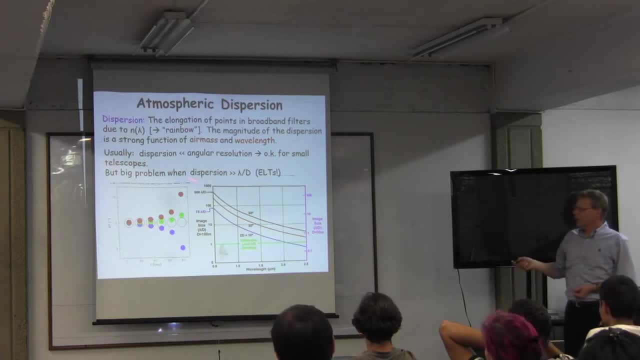 50 micro arc seconds, And then all these effects become very, very important. You don't know the spectrum of your source, You don't calibrate that out, And actually here is the challenge for you: It's a, it's a. 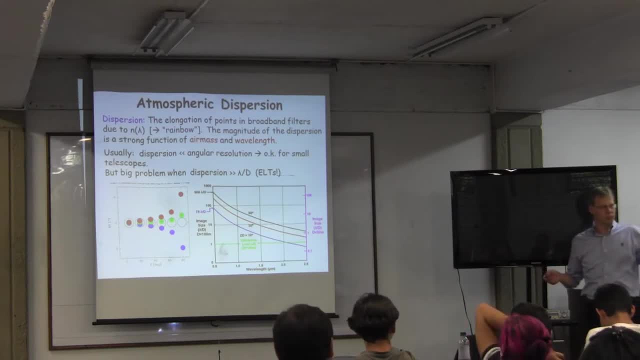 it's not not part of the test, But I, I, I say I promise that the argument will add an extra point to the to the grades, If you, if you tell me tomorrow how this could be compensated for. 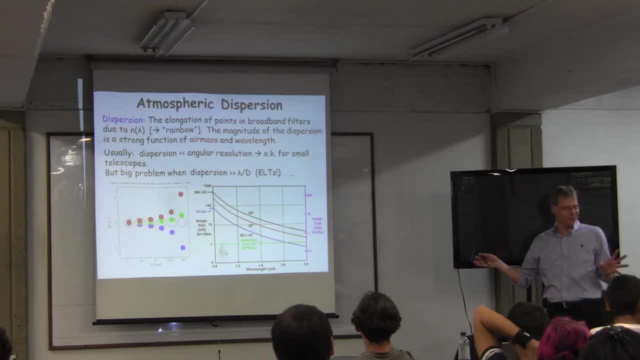 And if you have this effect, you have an idea. Folks, this effect is is a problem, As I said, and what people are working on technical solutions? Do you know how to do that, Like we know With? 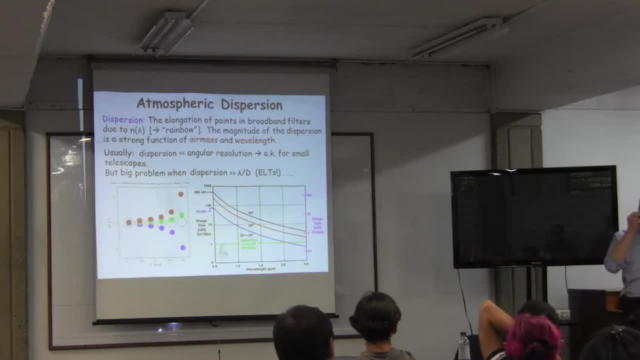 or without God, Without God, Whatever, Whatever, So. so I have a question. So you will, you will have no extra point. You will need the, the inspection, the solution and the source in order to, in order to do, 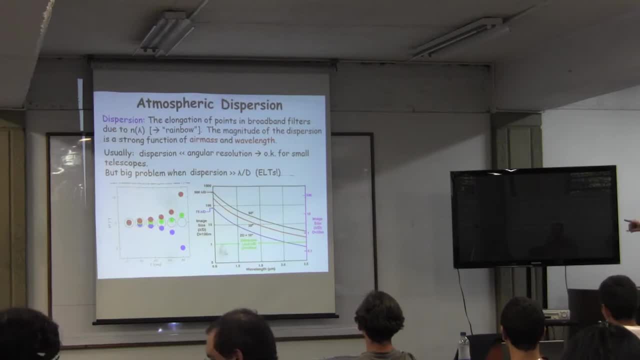 so, in order to do, you will need this inspection. The problem is that, in principle, in principle, you could, you could have, you have the rainbow and you could look at the center, Yeah, And if you would always look at the star cluster? 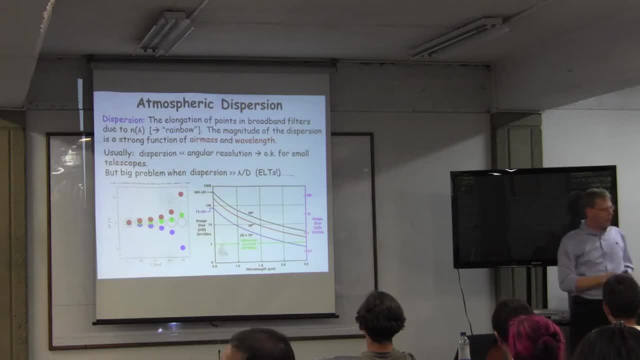 at the same angle, it doesn't matter. But if you uh track the, the objects on the sky over the night, the angle and the will change and so does the dispersion. And if you have objects of different spectral type, 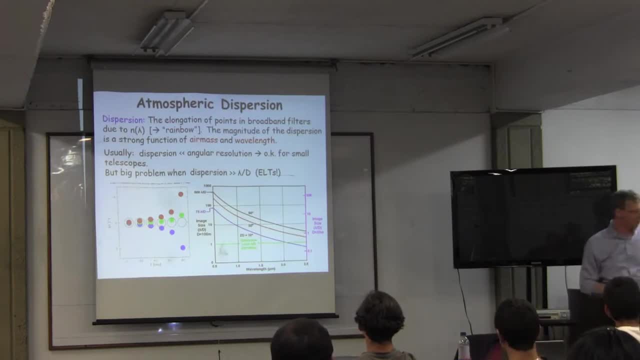 say: you look at the cluster that has some red giants and some white dwarfs and whatever that already have a different centroid. they move them relative with respect to each other, Right, And then what you, what you think is proper motion. 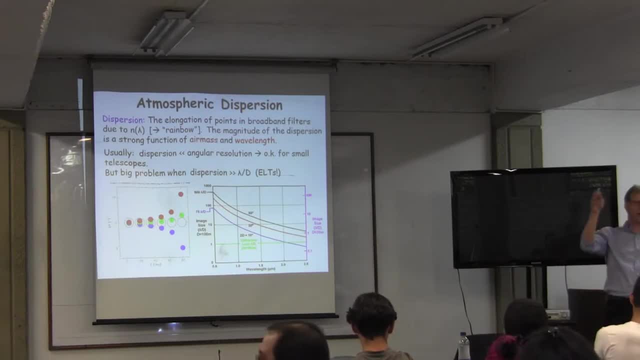 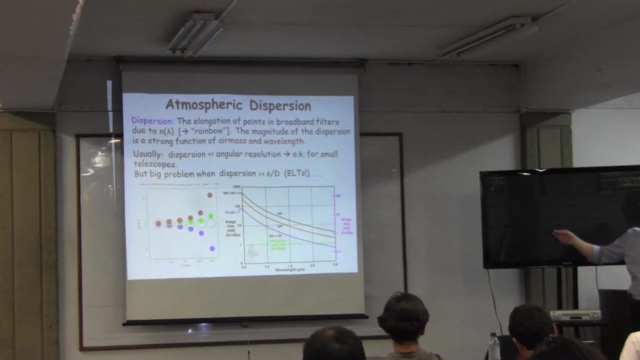 although there is a whatever big flag over there, because I see the stars move, is only an optical effect. Okay, So okay, But what can I do? I mean, if you do a, a, a, okay, 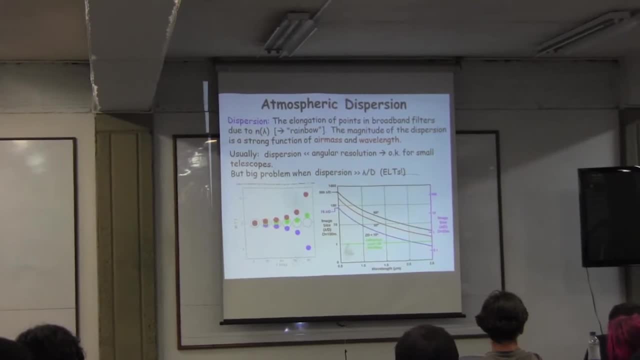 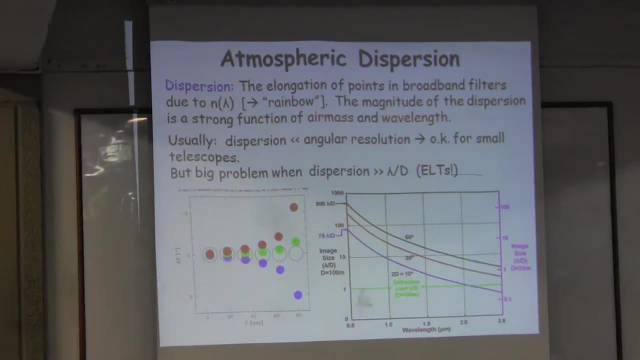 if you think you want to do a PhD in five years working on on some Gaia improvement of Gaia data, well, Gaia will then be up and running and- uh, these are really some kind of questions that that will be. 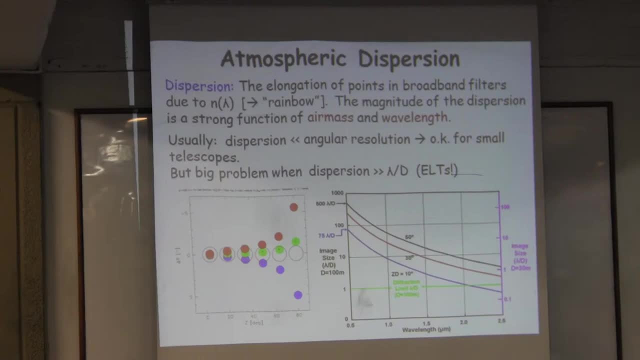 stable. But these are no problems. Actually, these are kind of like some kind of problem for me to to solve them. So so a a conscious programming program is actually spending 2 million to find a device to do that. 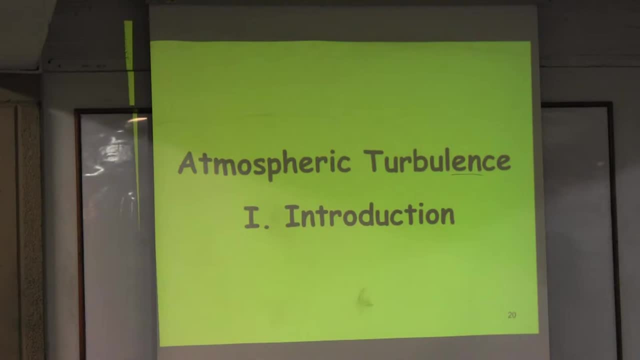 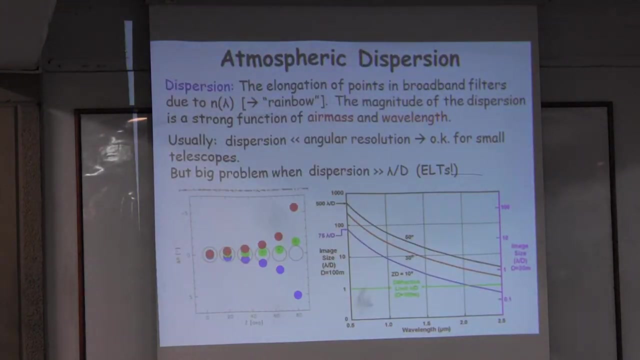 for an image or a video. Are you giving those to the student who answers your question? He explained the y-axis units, which is the y-axis. Oh, sorry, maybe that part is too complicated here. There will be no exam test on this part, but I'll try it here. 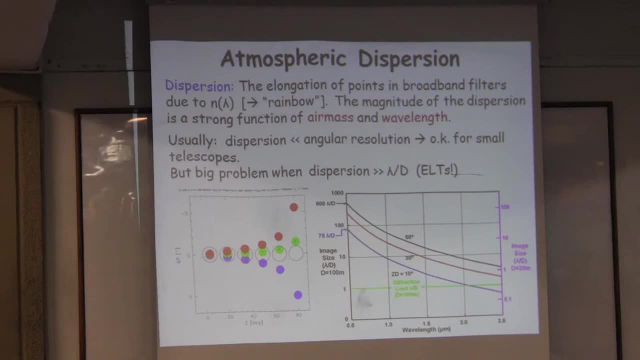 So ESCO learned on the first plane, lambda over d. that's essentially the differential unit of the telescope. That's how small your source can get. I said before that the star on the infinite distance is like a mathematical Taylor function. But then when you image it with your telescope, you will always end up with some extended log, no matter what you do. 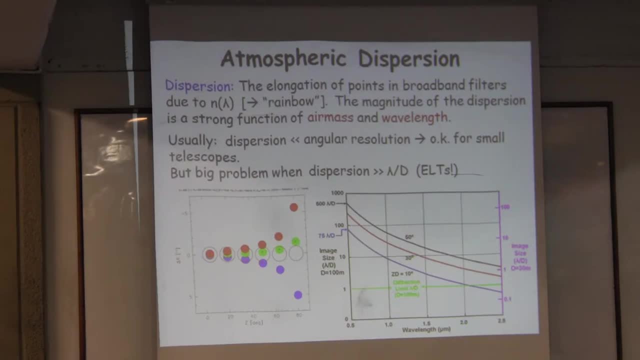 However, that log gets smaller and smaller If you use bigger telescopes. so lambda over d. d gets bigger, That factor gets smaller And lambda. well, that's the wavelength. Okay, so let's say you have the telescope here. 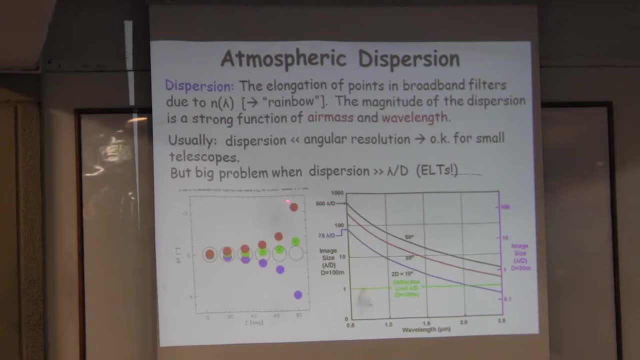 What this plot shows is the image size Essentially, if you would measure from here to here your image elongation And how it increases. looks for the wavelength Right. We said this is due to diffractivity index as a function of wavelength. 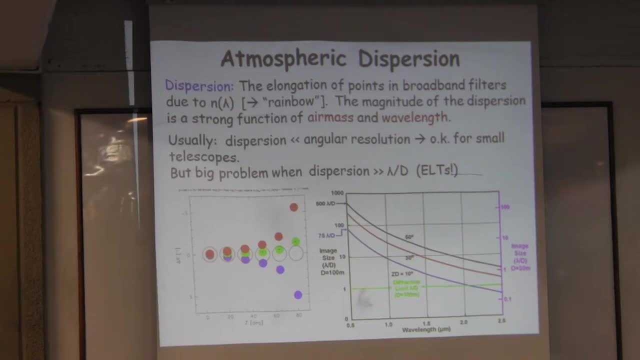 And well we also know blue light is refracted more than red light, So at shorter wavelengths the effect increases. But the main point to take away from this plot: just take one curve Right. This is just the difference in the distances. 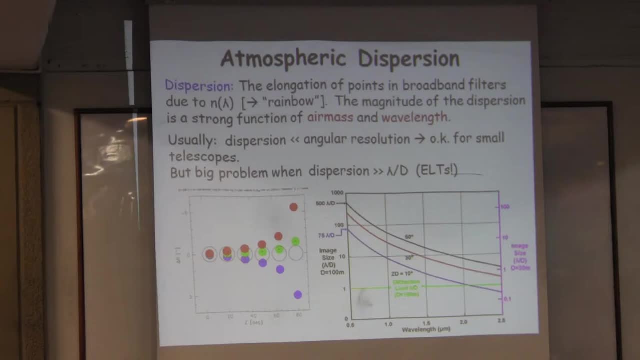 Let's look at 50 degrees, So we look at the star over there At one micrometer wavelength, And then we can see here that the size of the rainbow here is 10 feet. It's 100 times- well, probably 100 times- the size of what you would get without the dispersion. 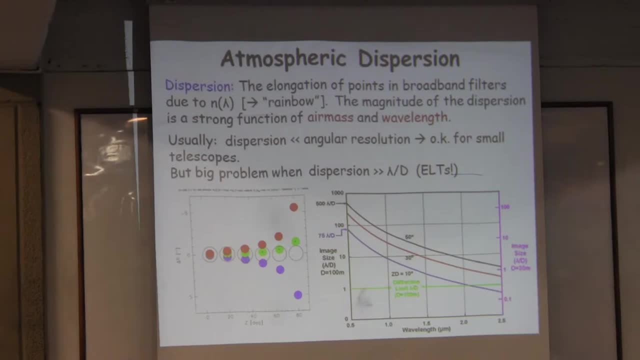 100 meters. It's 100,, maybe, maybe it is. yes, 100 meters. So if you take a 1 meter telescope, that effect goes away completely, Right? So you just have to divide to multiply that with 100.. 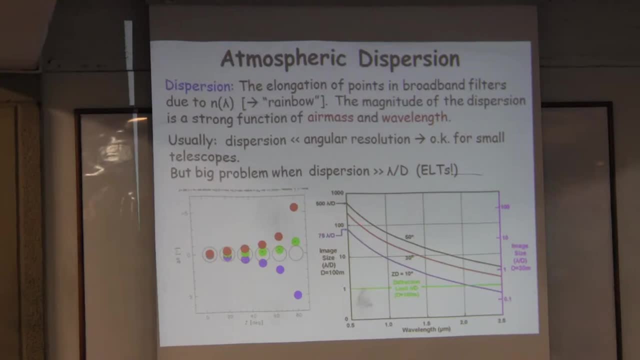 So if you have a 1 meter telescope, you will not see anything. If you take a 100 meter telescope, in one dimension the source has the same size as the source, Only that well, in the other dimension the source is perpendicular to the dispersion. 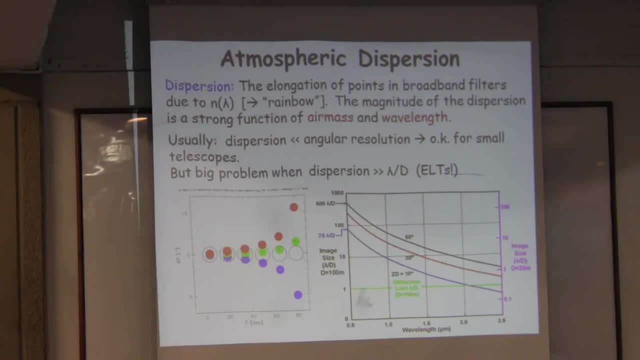 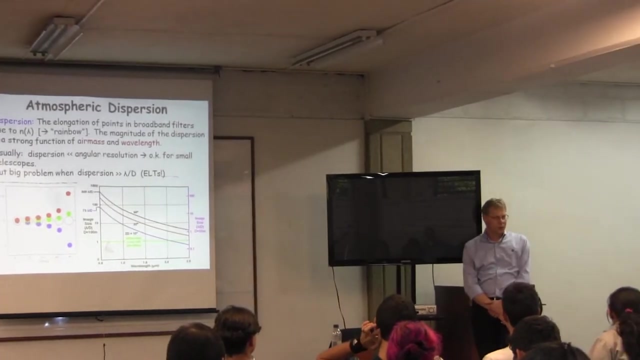 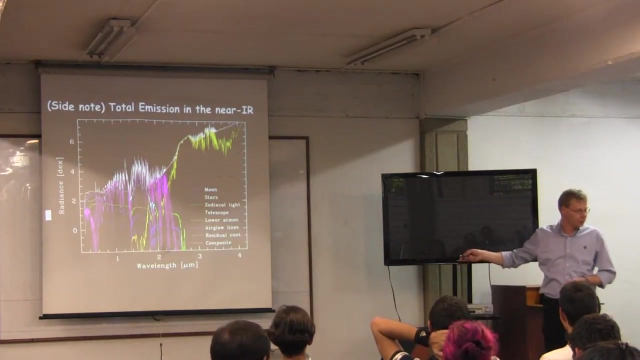 You will not see anything. We hope that is right. Okay, so much about refraction and vision. Do you have any questions? So far, Let's go to the test. Let's do this. well, the best thing. 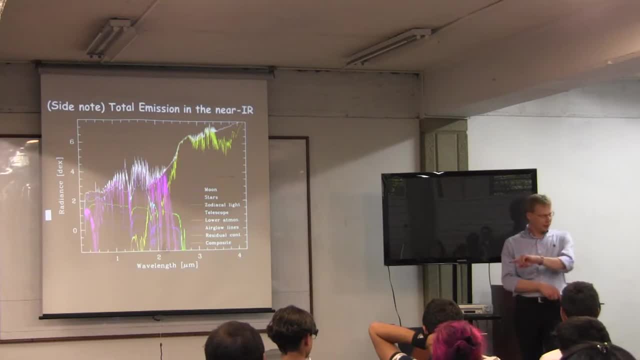 I won't get actually back to that later in this course, but the best thing you can do if you don't know all that. and of course people have models. I mean there are many people working on radiation transfer models and I'll talk about this today for the atmosphere. 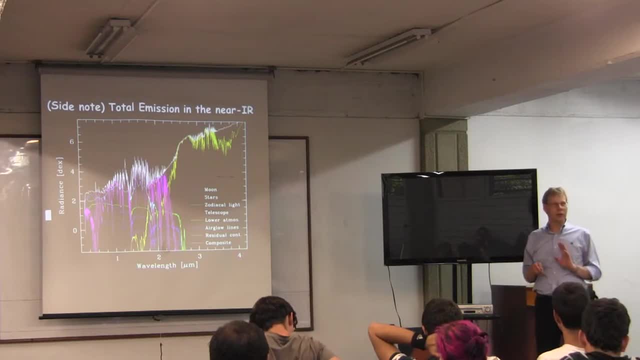 and they're actually quite good now. they're actually sometimes better than some of the calibration observations. so it's getting there. people really understand the physics of the atmosphere. but the easiest thing you can do is you look at the object, say your object, this is the bright object. 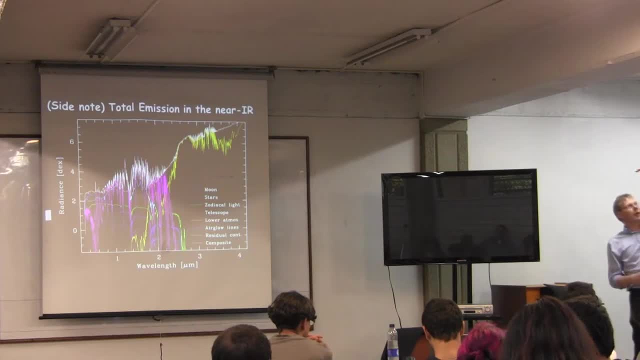 this is the light here and I observe it. the atmosphere is in between and I get both. I get the spectrum of the lamp and I get the spectrum of the atmosphere and I get the spectrum of the atmosphere and I get the spectrum of the atmosphere in between. 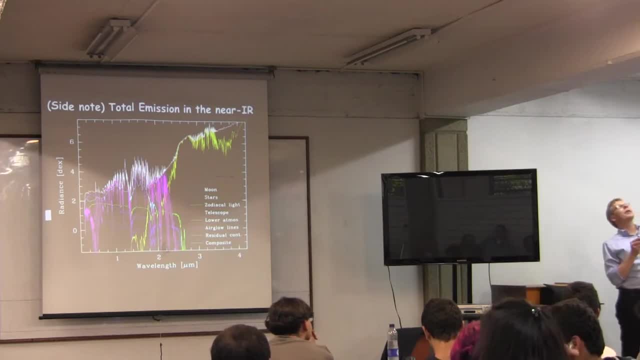 but the atmosphere is in the zero area. so I look at the lamp and I look next to it and I subtract the two, four divided, so I essentially compare a spectrum of atmosphere plus object to another observation of atmosphere only, and that's the simplest way of sky subtraction. 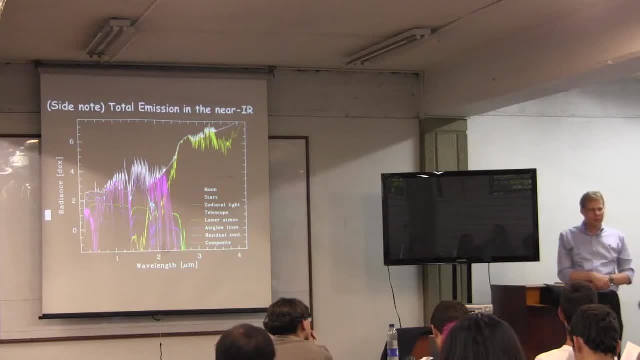 the problem with that is that you can't do it at the same time, you have to do it afterwards. first you integrate there, because the object is usually fainter than the lamp here. you integrate for a long time- half an hour- and then you go to another position on the sky. 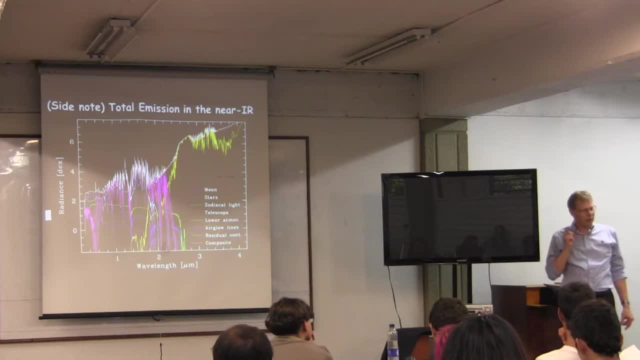 but in this half hour maybe the atmosphere is changed. the problem is, the atmosphere is changed. it's not constant in time. so then you subtract the two. in the ideal case you can subtract out the atmosphere completely, but because it's later during the night, or we said before, 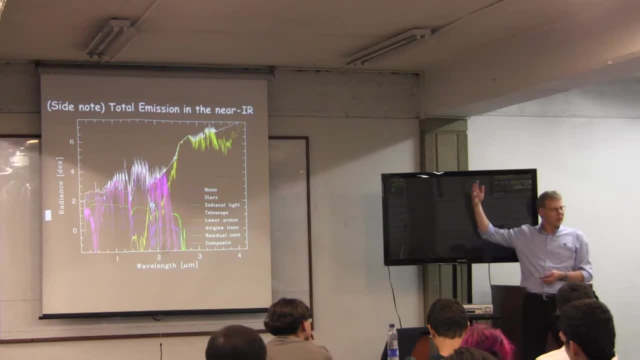 for fluorescent emission. it changes as the ions recombine, so some of the signatures will change with time, and so it's difficult to find the right calibration to figure out. how often do you have to go back and forth between your object and the sky? and yeah, that's the art of observational astronomy. 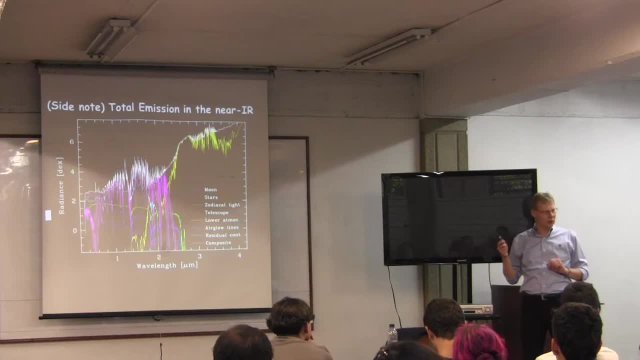 to find out what is the best calibration strategy for what you take. but the simplest thing is go back and forth between the object and the position on the sky which is close to the ocean it's also if you go far away, and far doesn't mean 20 degrees. 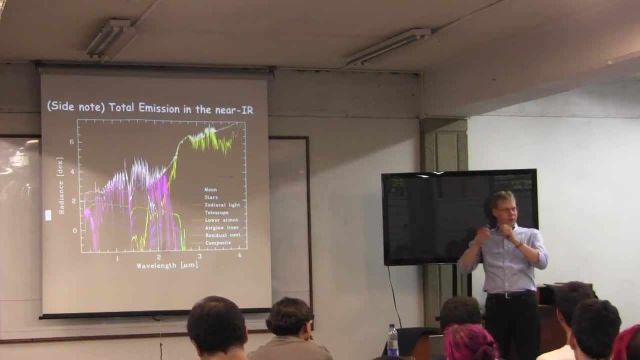 far is already one arc minute. if you go far away, the atmosphere may already be very different from your actual source location, so you want to go only a tiny little bit away. but of course, if you have a big galaxy, that's not working. if you have a galaxy, 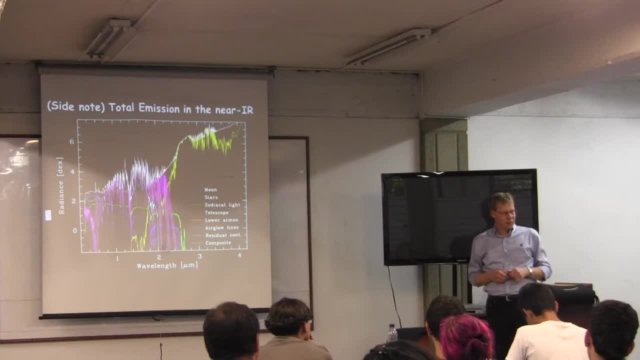 that's 30 arcs of arc minutes and you go only one arc minute away. then you subtract maybe the other parts of the galaxy from the central part of the galaxy, and that's when you subtract all the features of itself. that's not working, so it's challenging. 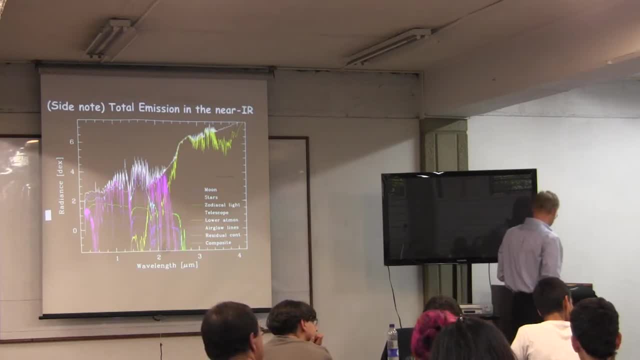 can you use this artificial star, these lasers or all the sources of light that you know? is there no, no for ok, it's a definite no because there are. well, we'll see later when we talk about adaptive optics. there are two ways people produce artificial stars. one is the ray scattering. 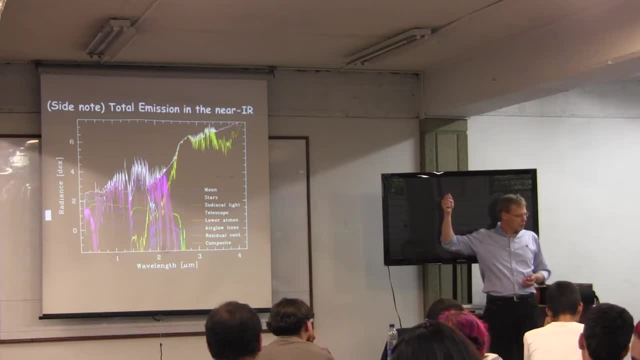 which is only a 10 km height. these are continuum lasers, essentially, but they only give you the information about the lower 10 km of the atmosphere, so they don't show you what's up there higher up. or you can use a, a resonance scattering of of the sodium d line. 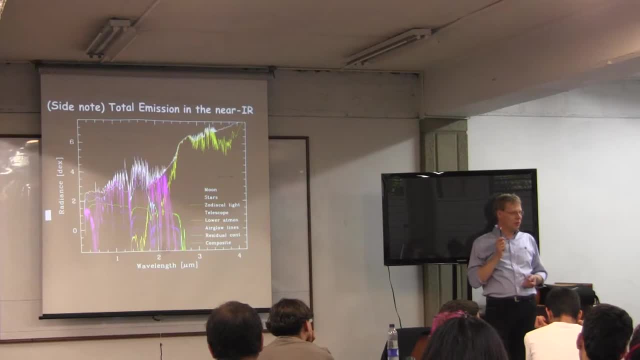 at 90 km height, then the problem is, if you have only monochromatic information, then you can't calibrate your spectra. what you could do, of course, is to send a- well, a bright emitter up there. so if you have a billion dollars and you don't know what to do with it, 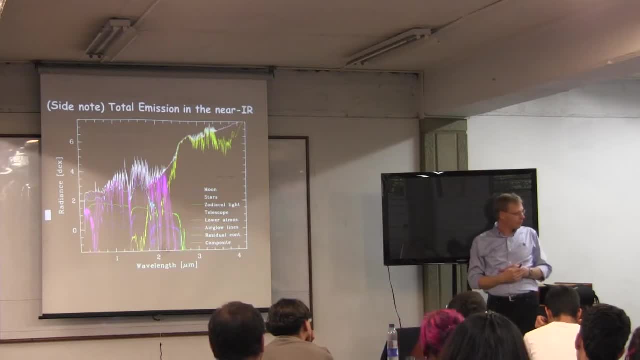 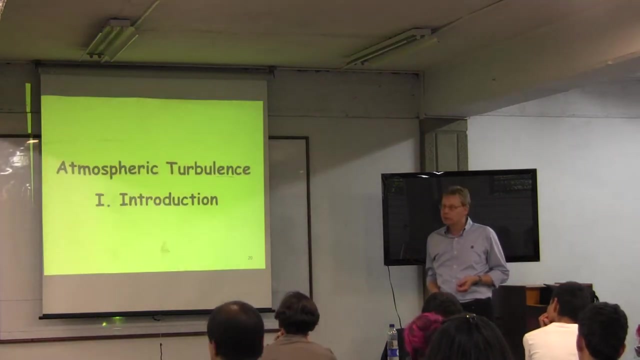 you could create your, your artificial source in orbit, then you would have your the sky full of well traditional, I mean you could. you could use the space station, for example. it's fairly bright, but it's never where you want it to be ok. so I have another question. 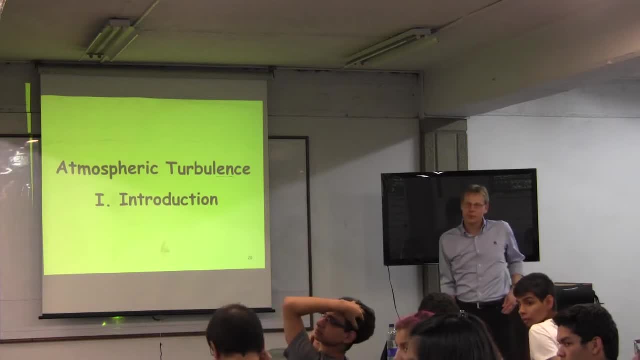 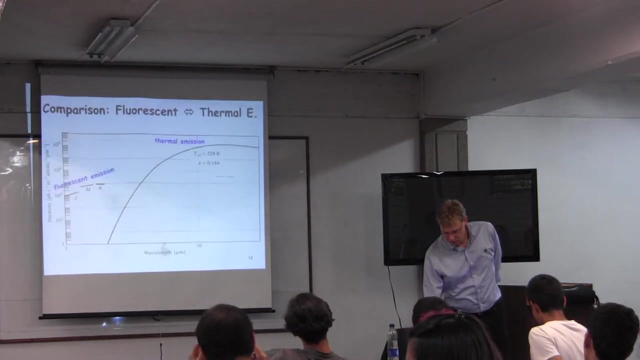 I'm sorry. yes, please, a nice question. you told me that you know there is the relation between atmospheric emission and the dark barrier emission- the two. when you talk about two types of atmospheric emission, there is something called thermal emission and then we have an equation. in this equation there are 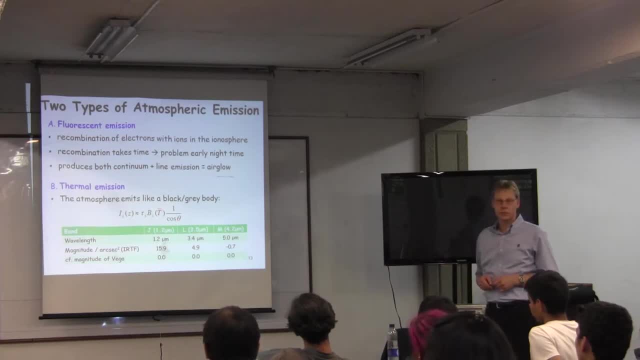 a term, that relation between a dark barrier. so when you start the dark barrier, there are so many things that are different. I don't know, but it's difficult for me. so I want to know the relation or the boundaries between, between the thermal emission and the dark barrier emission. 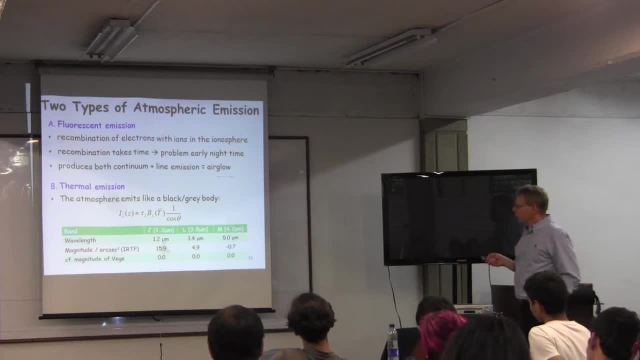 ok, so I'm not sure I understand your question completely. yeah, of course this is a a simplification again, but it it usually works. it's a simplification already, because if we think about the atmosphere as an ocean with different layers, then all of the layers of course we know. 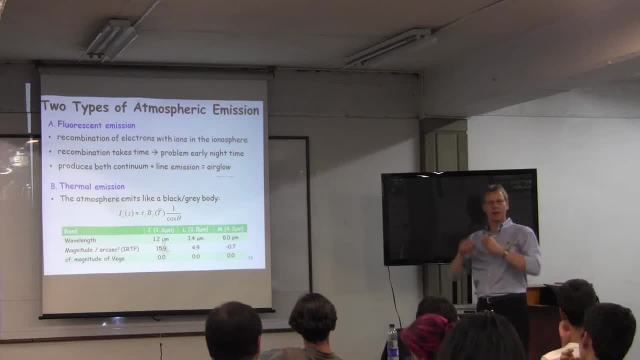 how the temperature will drop, have a different local temperature, so you already integrate, or you already integrate over a couple of different. I mean you could. I mean the nice thing is, if you add black bodies, it still looks like a black body, right? so you might have one. 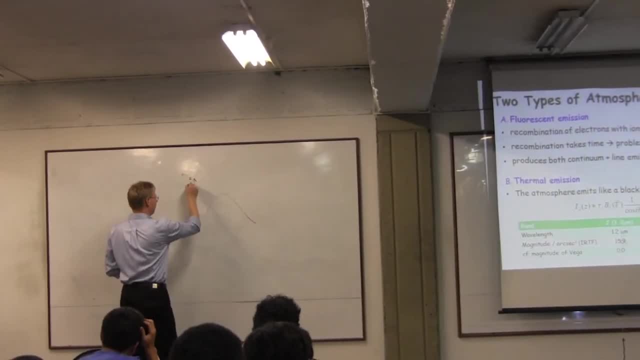 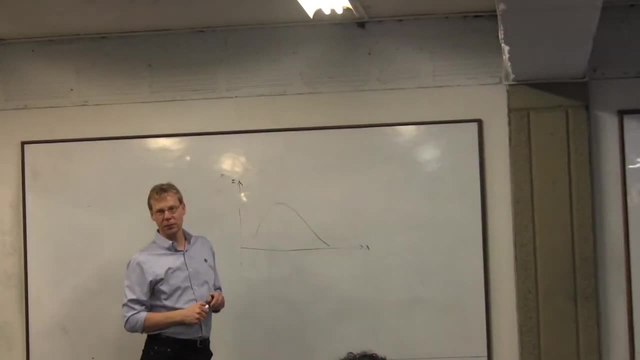 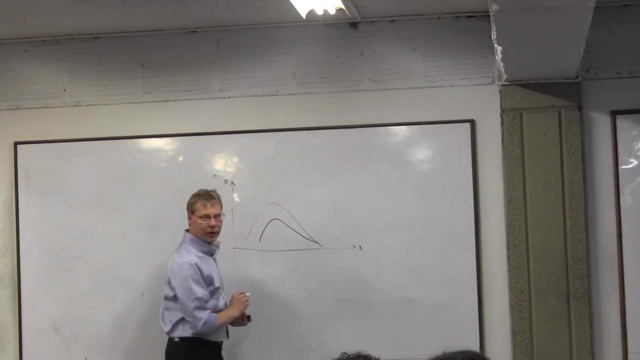 black body. it's basically the density here and the wavelength, so maybe that represents the lower one and it's, it's warmer, and then you have a, a fainter one and an upper layer, and then then this is: this is even higher up than the, the atmosphere. 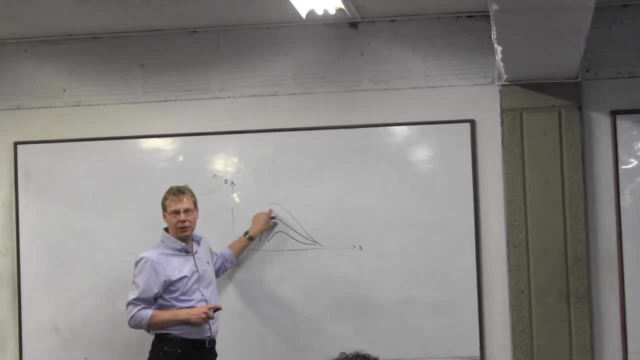 and then you also. they're not all contributing the same amount as in this formula here. you have the opacity there and that depends on the density right, and of course the layer on the on the ground is denser than the one at 50 kilometers higher, so that one 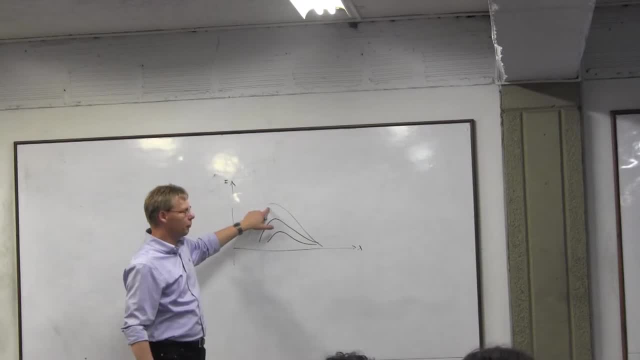 will contribute even more than that, and so in most of the properties are given actually to the layer which is pretty close to the ground, and then we just assume it's a. in reality, of course it's not, because then you have what's not shown. here are all kinds. 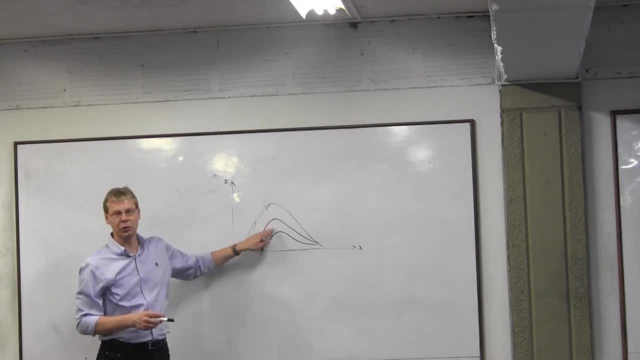 of absorption bands or molecules, right, but this is a higher order effect on top of that. so usually it, it, it works quite surprisingly well. you, you take- I mean you can take your- you go to the observatory, you have 10 degrees Celsius, right. then you assume. 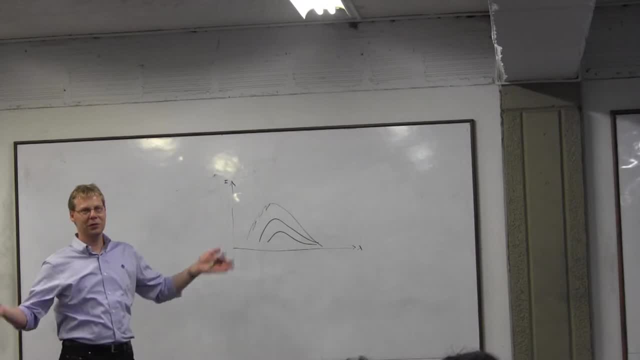 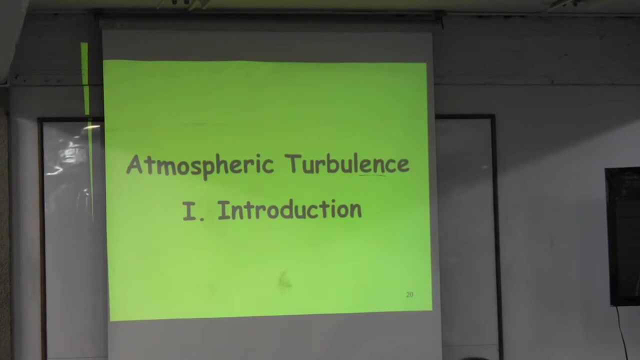 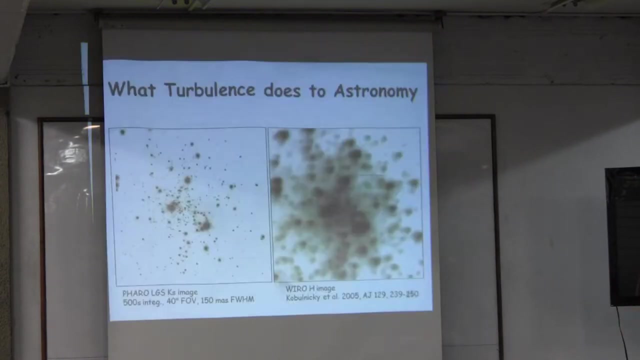 it's a, it's a whatever effective light body of 283 Kelvin, and then you're not so far off. okay, okay, turbulence this is. I realize this is also challenging and it's not my intention that the most challenging part of the lecture is just before. okay, let's see. 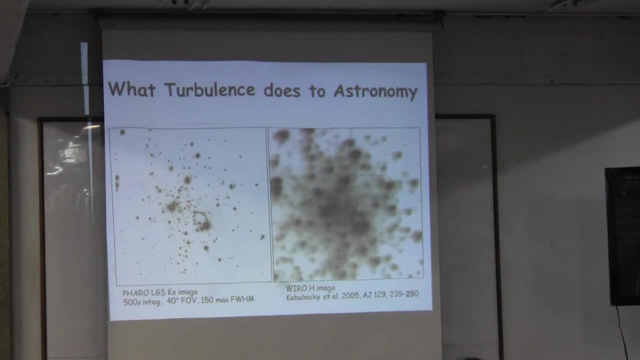 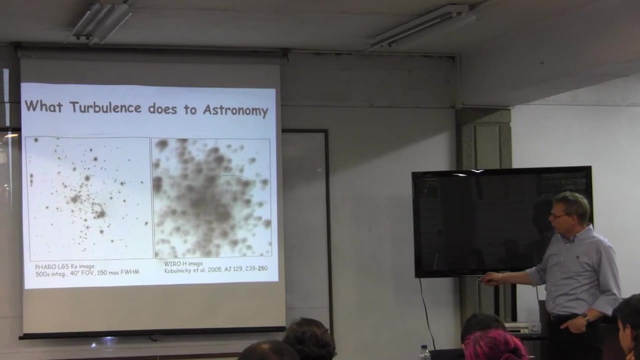 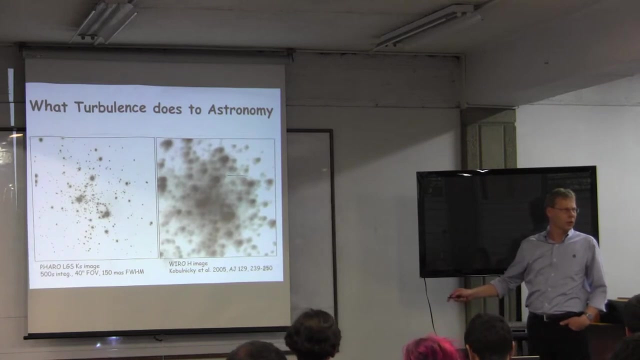 first, why we worry about this. I wouldn't I wouldn't talk about it if it were not important. this is just a comparison of the same star cluster in this case. yeah, this was why we this Wisconsin, I think- observatory, so this is an image taking at 1.6 micrometers. 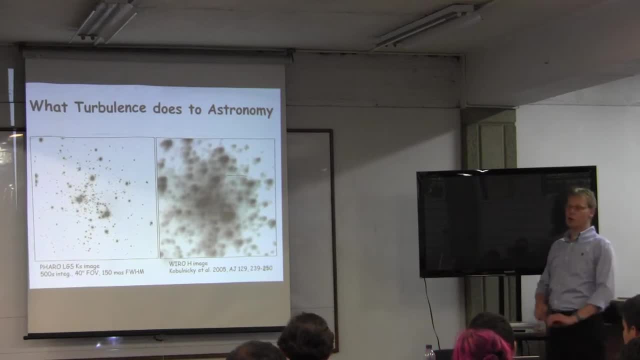 of the star cluster seen, so not correct for atmospheric turbulence. this is what you would get when you point any any, let's say without. on the left one: this is the one taken at similar wavelengths. well, this is the one taken at 2.5, but with an adaptive optics. 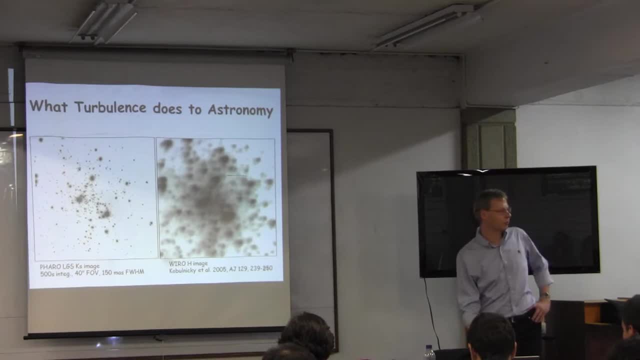 system that corrects for the atmospheric turbulence. same star cluster, same, and there is. there are essentially two fundamental aspects that you gain when you get closer, when you overcome the atmospheric turbulence and see and get a different. so there are, yeah, what, what would be? the two things. 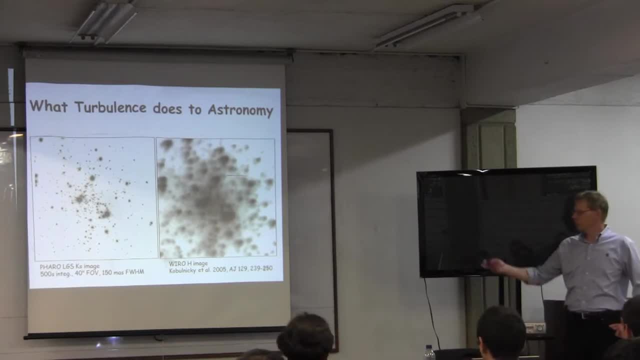 I mean you just look at me. you should be able to tell me what difference, what, what I mean you see some difference and then you ask what? what's the difference? that you need the size, the size of the point. so resolution is one thing, right, I mean. 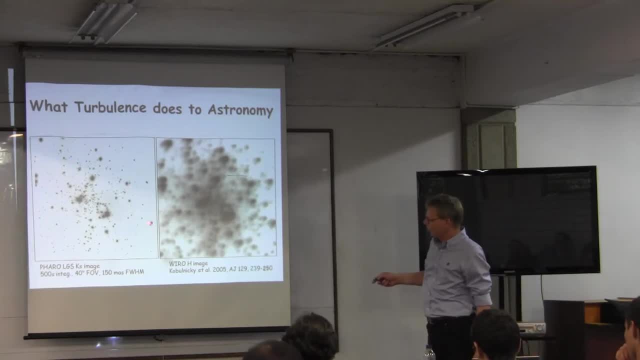 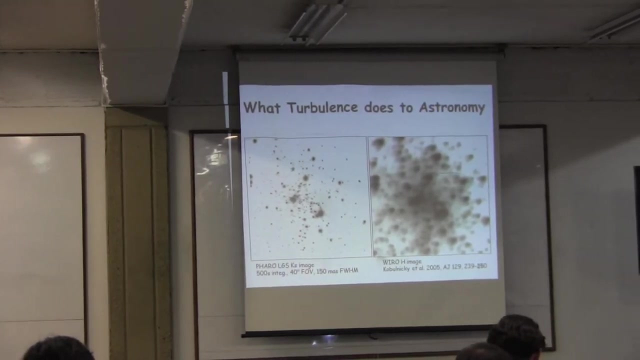 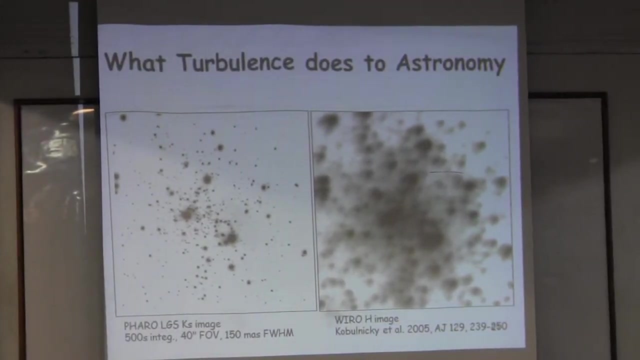 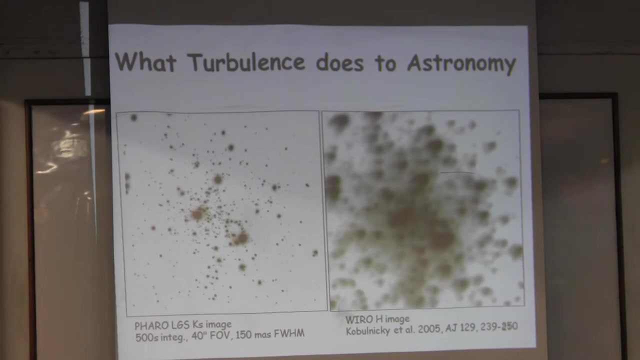 we can, we can, we can look here this one here. I mean you can see two stars, right, so we, we gain resolution, angular resolution or spatial resolution. but there is another effect here, any idea? it's maybe not so obvious in this. okay, I'm helping because can you see that? 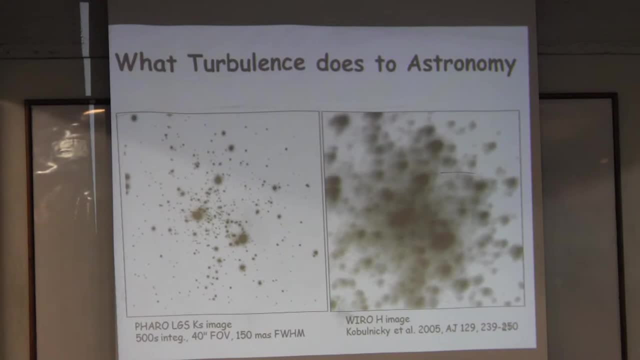 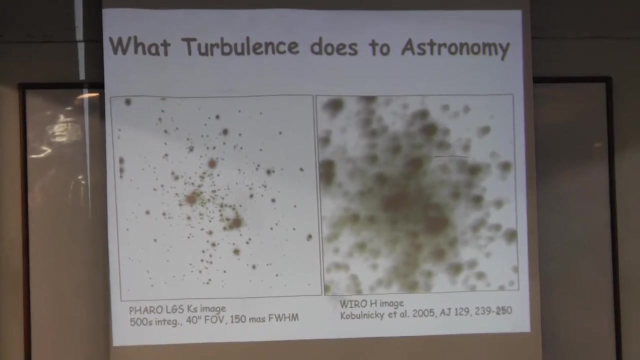 that dot here. yes, okay, there, I invite everyone from the background. okay, so, and there is nothing here. and the point is that if you concentrate the light, then you also have more photons between the same area of your detector or your ccp or your photographic plate, whatever. so the 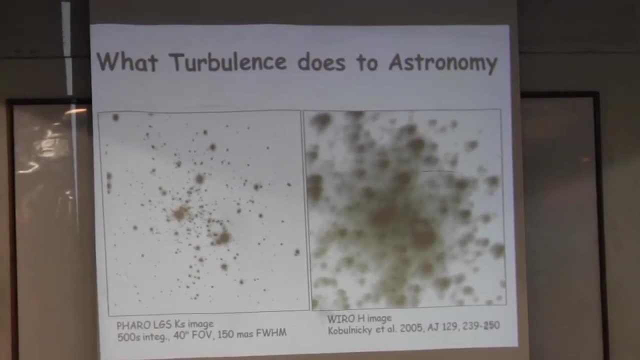 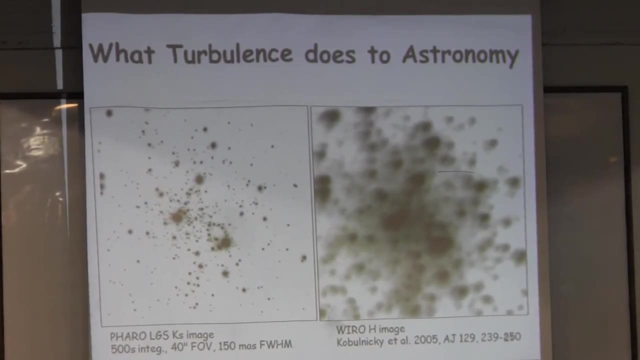 and you gain insensitivity. you also have what we said before: the background, thermal background, fluorescent background, whatever all the background sources we talked about. they are all across. they are all across the image, but they are the same here and here. right there, right there per unit area. 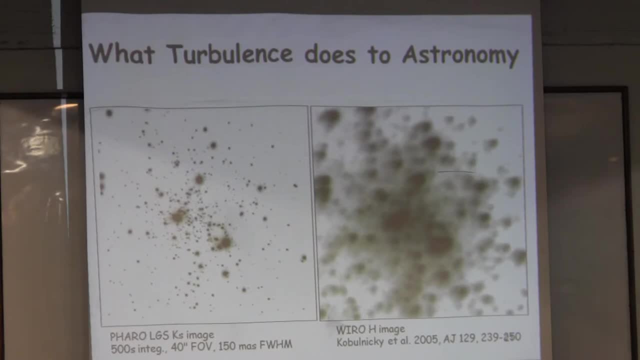 the background covers the whole sky. it doesn't care about whether we have turbulence or not. it's the same strength here and here, for every point, but in this case the information or the light from the source is concentrated in a much smaller area with respect to the surrounding. 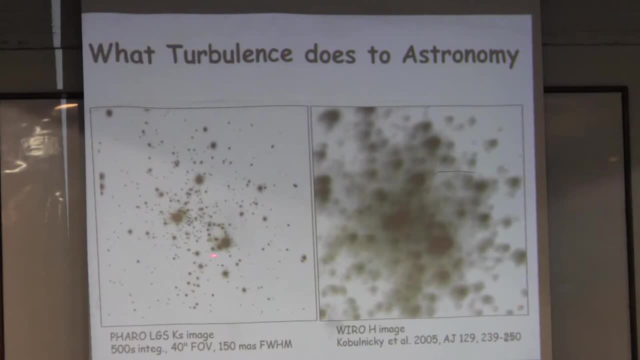 background than in this case, and so here we can see much fainter sources, sources that we hear be beyond the detection. we'll get back to some aspects tomorrow when we talk about signals and noise, but so these are the two main things when you get to the diffractual area. 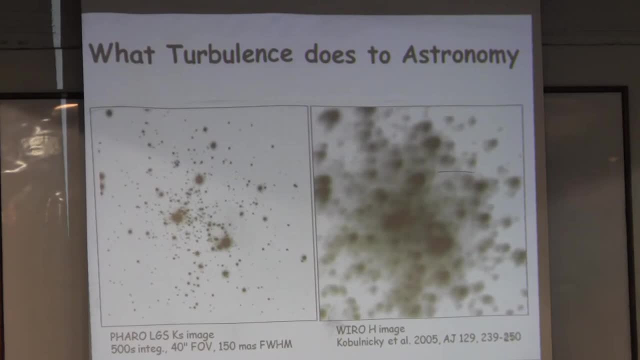 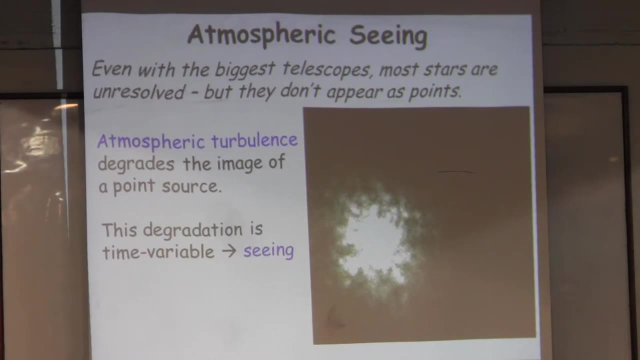 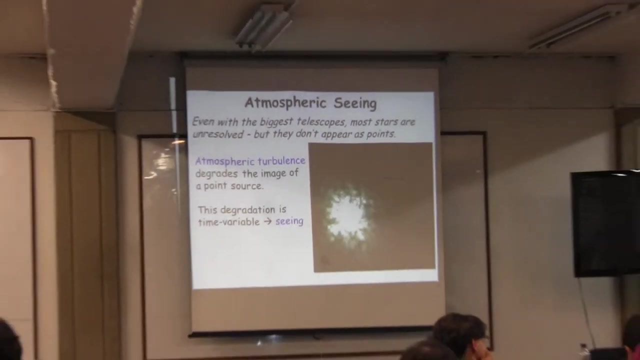 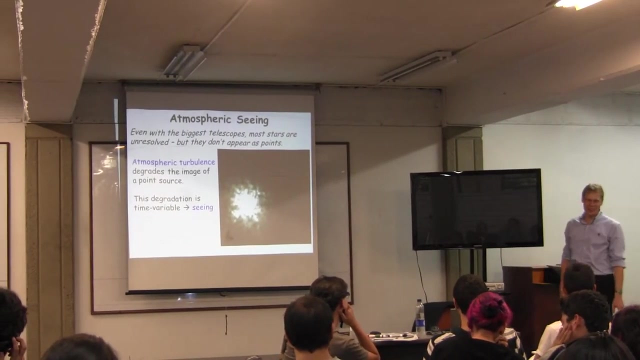 you gain insensitivity and you gain in angular resolution. ok, and there is, yes, it's not exactly the same instrument, it's not exactly the same integration. yeah, yeah, it's, they're similar, they're comparable, but it's not exactly the same instrument. yeah, I mean the 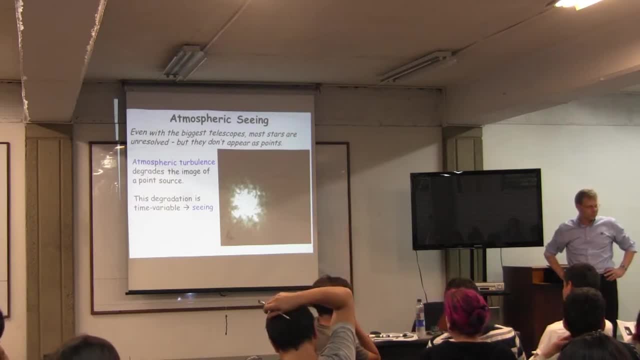 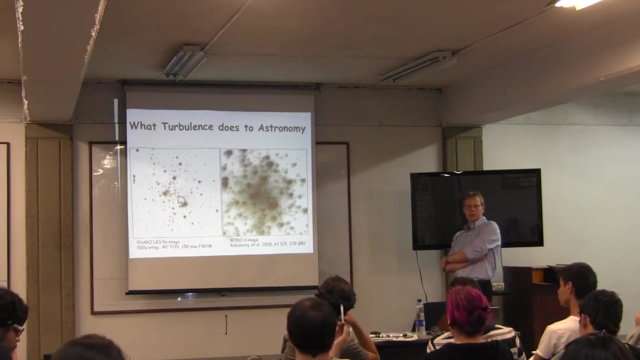 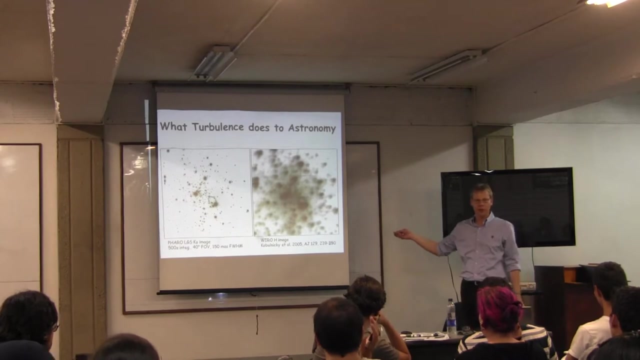 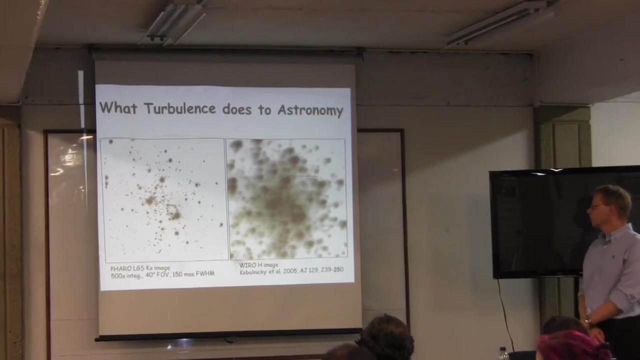 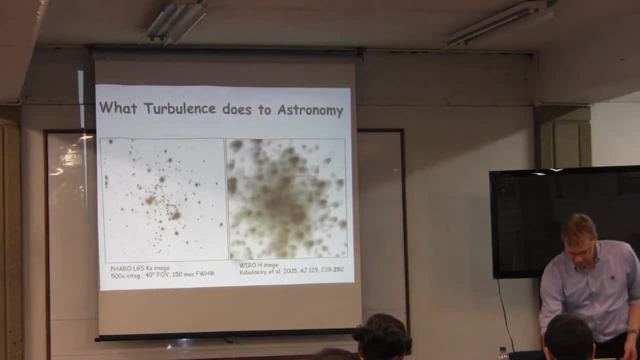 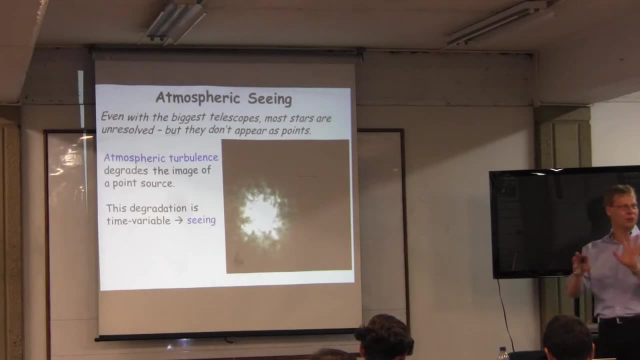 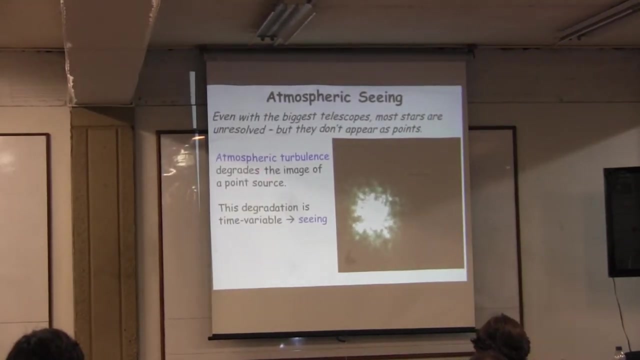 okay. so why is that? and i think if you haven't seen how, on this picture, or what nature does to our ideal points of our surface of the star, you should watch here a movie of short exposures. so so we said the atmosphere in turbulence degrades the image of a point source, but it's. 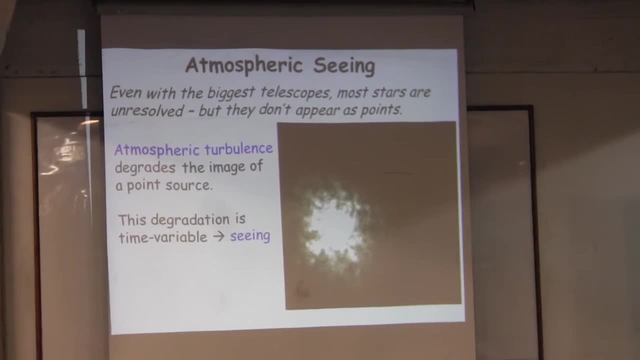 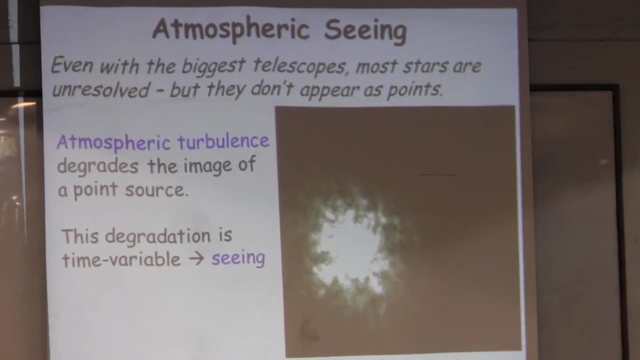 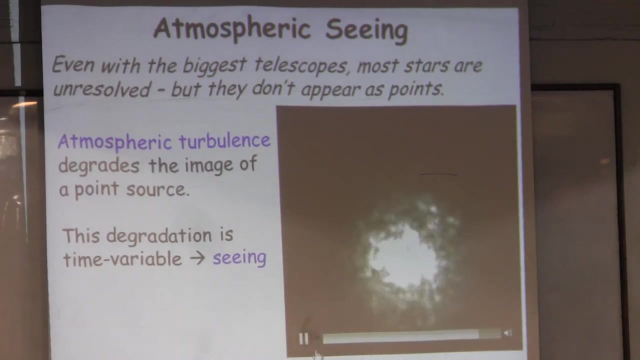 not like constant degradation, like a standing aberration, like you have an arrow in your optics, but it's a very dynamic effect and this is called the c and i'll show you. this is a regular, so this is a typical sequence of observations. i'll replay it a couple of times, if i can. 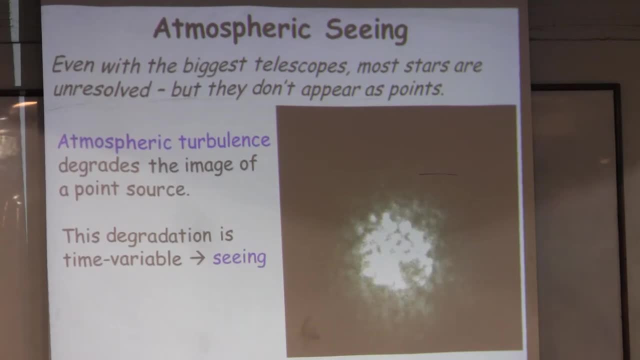 so this is really an image of a single star and it moves around and it has all those structures and this is simply, well, that's what the, the atmosphere does for your, to your image, all right, so it does not stay stable. the central way moves around, the structure of this cloud moves around and, of course, if you now 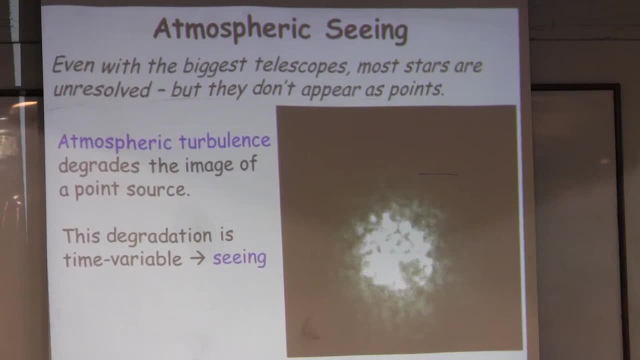 well, would take a long exposure right. as i said, this is a. this is a movie of short exposures. okay, i don't know, maybe this was one second altogether for a bright star, but let's say you, you're integrating for half an hour. of course, then you would get an average of all that. 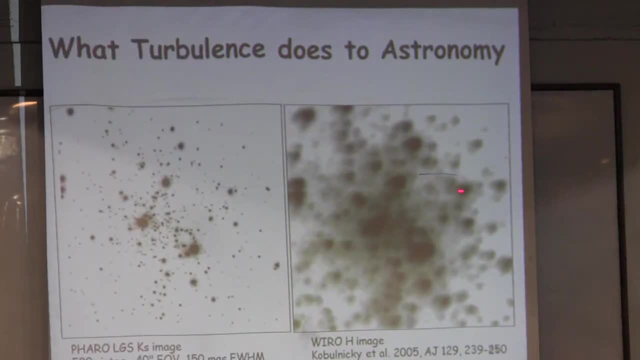 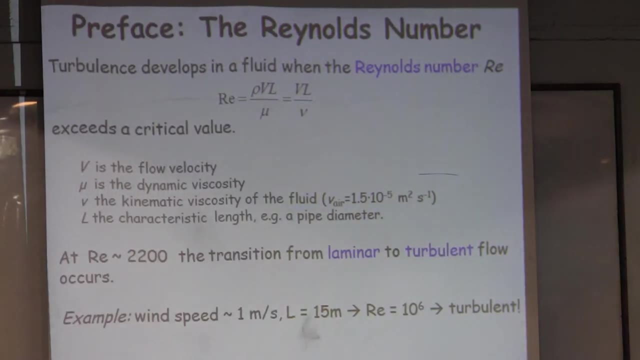 and the average looks like this, something like that: right, all the stars are some some third blocks, okay. so that's why we want to understand the atmosphere. if i want to build something that compensates for that funny part of that. first let's talk about- and yeah, i mean, why is the atmosphere? do we know it actually that it's turbulent? and, yes, we know. 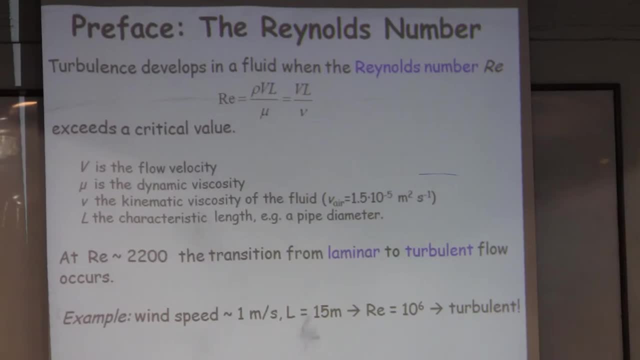 this is a sort of a side note. there is one simple quantity that people who study turbulence know very well: the Reynolds number. and the Reynolds number is defined here as the ratio between density, flow velocity and the characteristic length. now, this is over which we studied that. Imagine you have some water flowing through a pipe, then the characteristic length would be the diameter of the pipe. 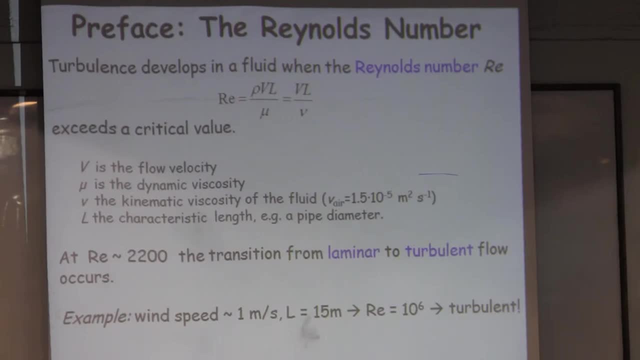 Divided by what's called viscosity. Oil obviously has a higher viscosity than water, And for air it's very small. In other terms, the flow velocity times the characteristic length divided by viscosity. Okay, so there is a sort of a magic number: 2200.. Don't ask me why. 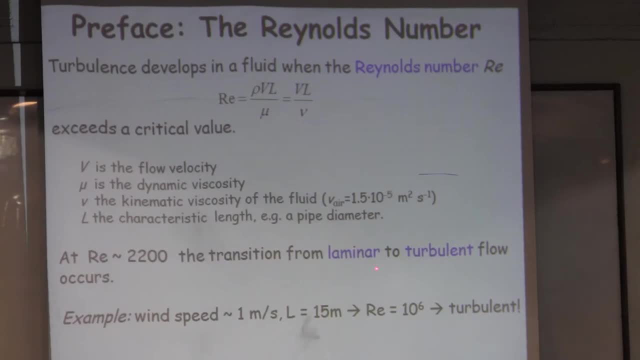 That's sort of the transition point between laminar flows. The laminar flow is what you observe when you're in an airplane And we fly through the air. You fly through the clouds and you see the air streaming across the wings And you better make sure it's laminar. 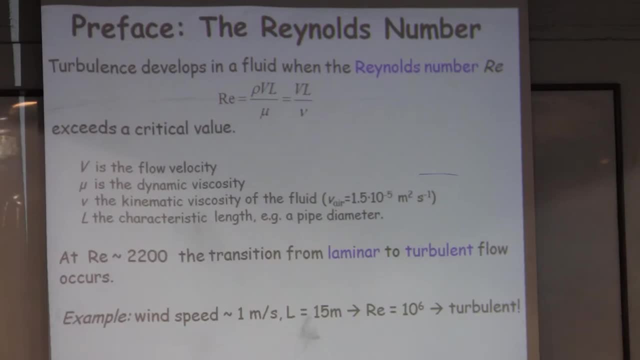 Because as soon as it becomes turbulent you probably have a problem in the plane. So there is the laminar flow across the wing, Or if the Reynolds number is less than its laminar, if it's larger than that, it's turbulent. 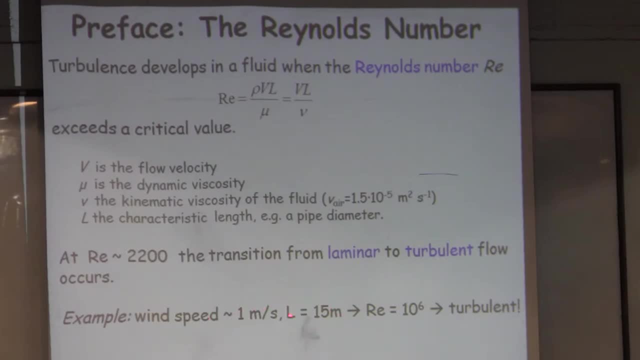 And if it's larger than that it's turbulent. If we include something here for the wind speed- typically an observatory can be larger than that- That only makes it worse. Scale length, of say, 15 meters- we get to that point. 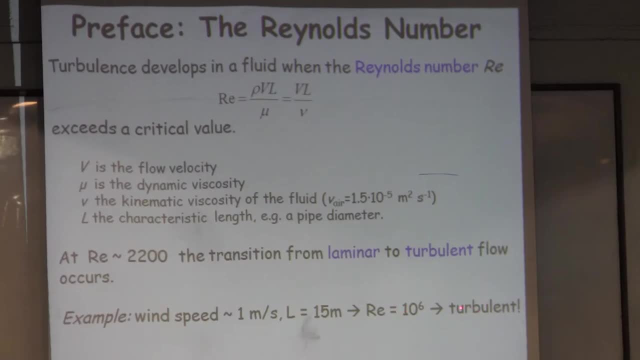 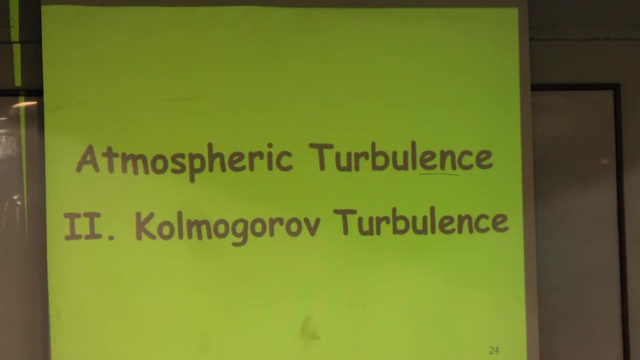 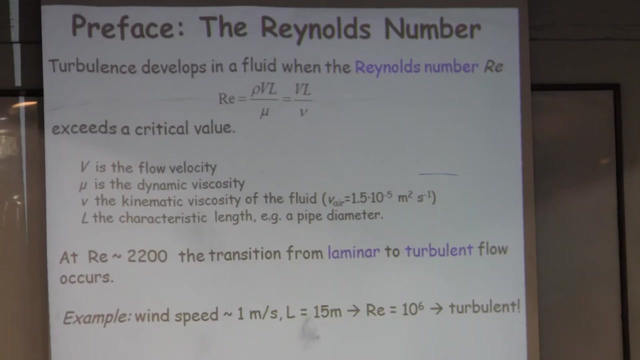 But then the Reynolds number is 10 to the sixth, So in any case it's turbulent, The air above there is turbulent And People have been studying the term. I have a question about the scale length. It's something like the decay of the blocks. 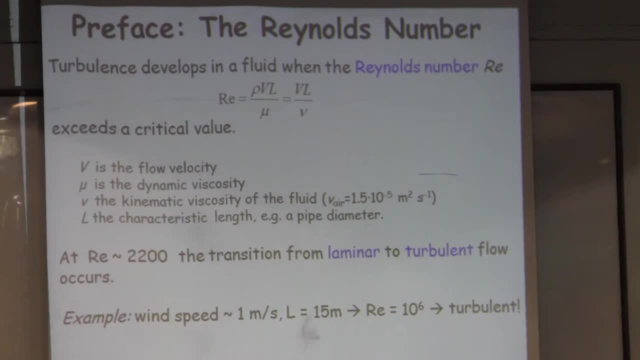 Or is the size of our cells? What is this? This is, Yes, this is ill-defined, But if I have, Let's see if I have a picture of this. This is the width of some lander. I think I have a. 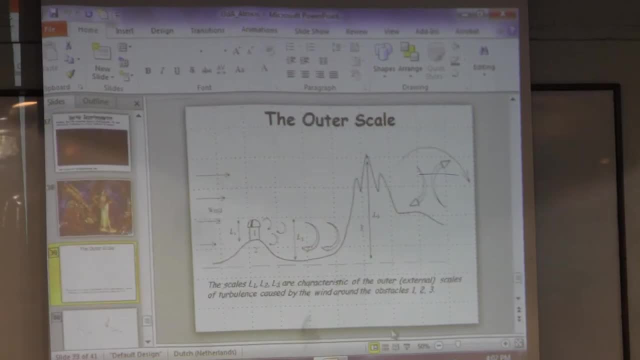 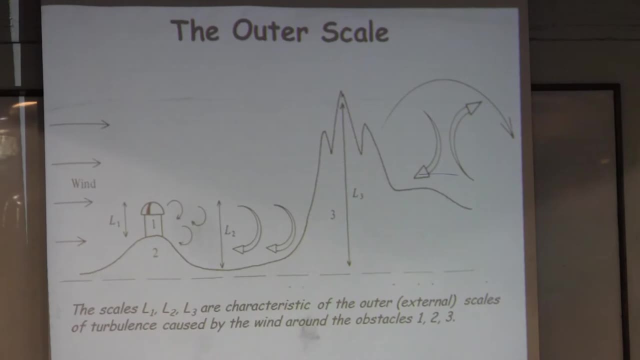 Let me just go back to. This is another approximation: 15 meters. Well, it's not 10 centimeters and it's not a kilometer. So why is it 15 meters? Because if you have an observatory somewhere in the mountain, 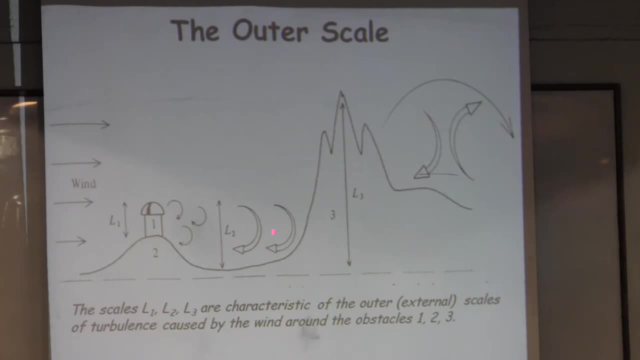 that's the typical length for separation between big objects on the mountain Right. It's the size of your telescope. It may be whatever the size of some trees, Something like that. I realize this is not very well justified, But the main point is with 10 to the sixth. 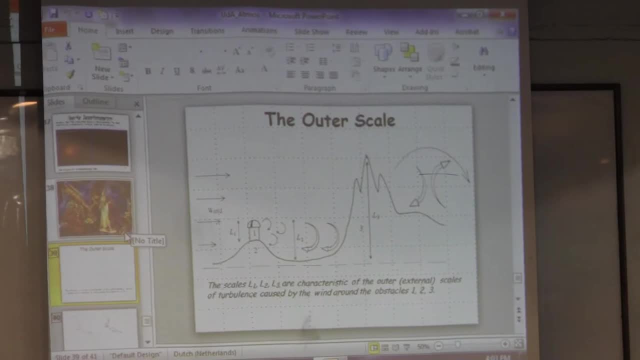 you're so far above the 2,200 Reynolds number, But you can easily use another. If you don't like 15 meters, use 30. But if you have very small values like this one here, you have less duplicate boxes. 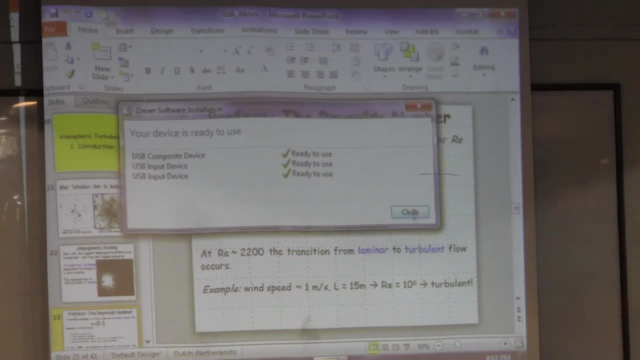 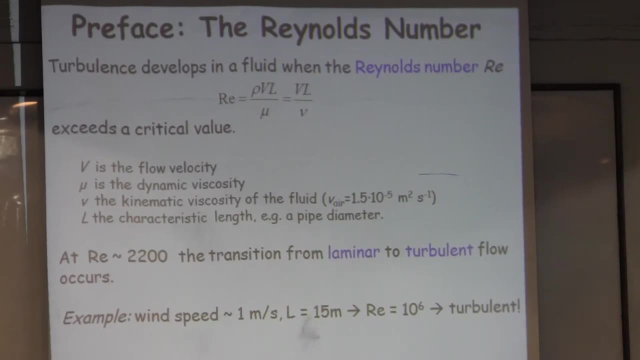 Right, So if you walk, for example, in a desert instead of a mountain, in the mountain top, you have smaller, small values. Yes, That's because in Colombia we have a lot of deserts, Right, Cool. 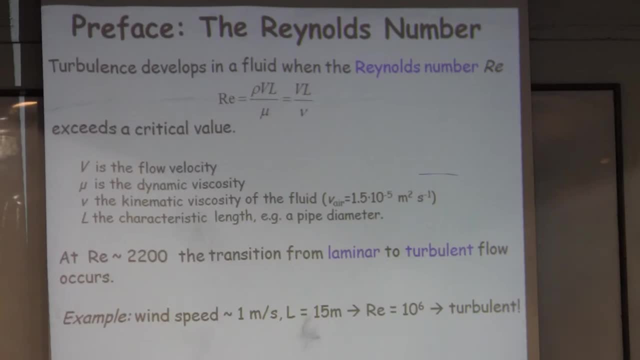 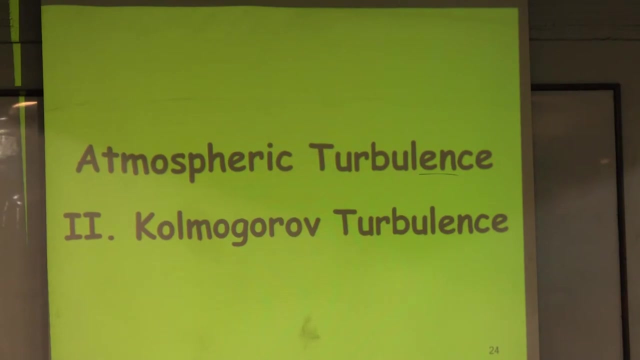 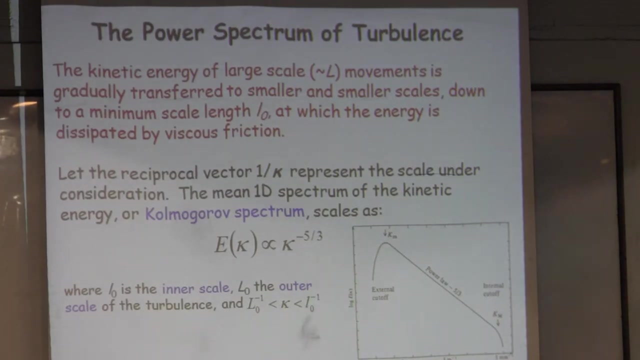 So another point, Yeah, But of course then the problem is that if the wind has no obstruction it may give a lot larger wind speeds, So you always lose, OK. So there was a Russian mathematician who studied the turbulence carefully. 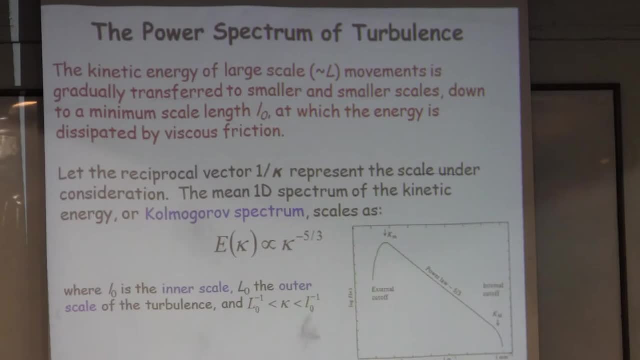 And so we all assume meaning people working on systems that correct the, Assuming always that it's a- We know it's not true, but it's- And what it means is that the kinetic energy of large scale movements is 15 meters, sort of. 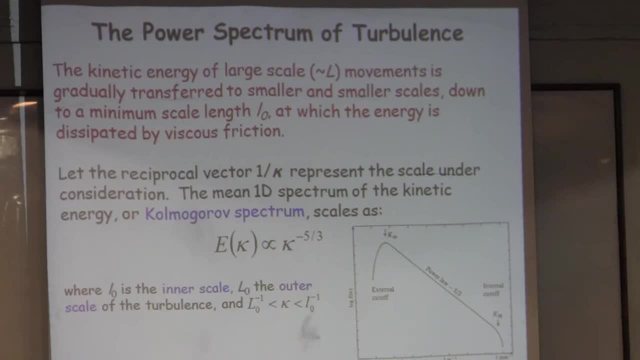 It's then gradually transferred to smaller and smaller scales. It's not like you have big turbulence at 15 meters and that's the only thing you have. That's sort of out of scale, as it's called, And then you have smaller and smaller scale sizes. 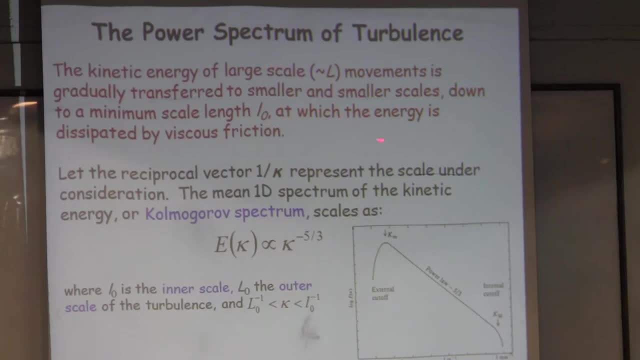 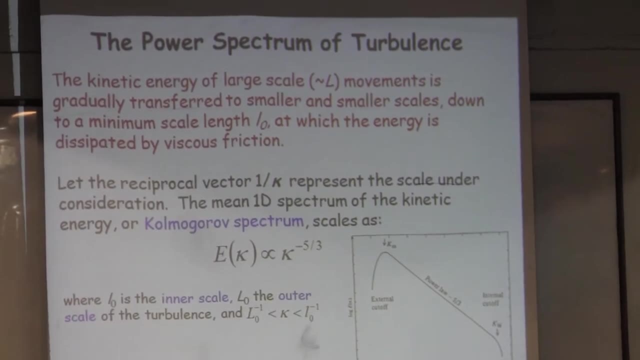 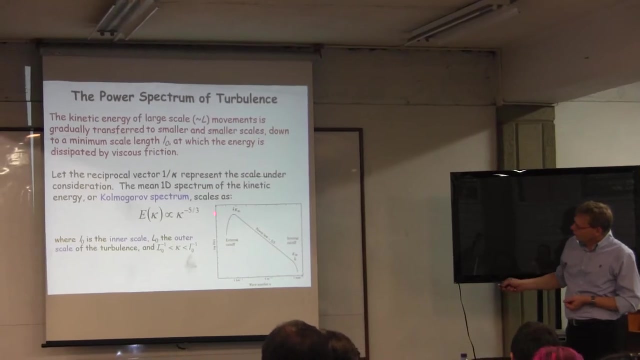 of this turbulence down to minimum scale lengths. And then the minimum means that if it's below that, the energy is going to dissipate into a beat, essentially by OK. So what's shown here is essentially the energy of the spectrum. 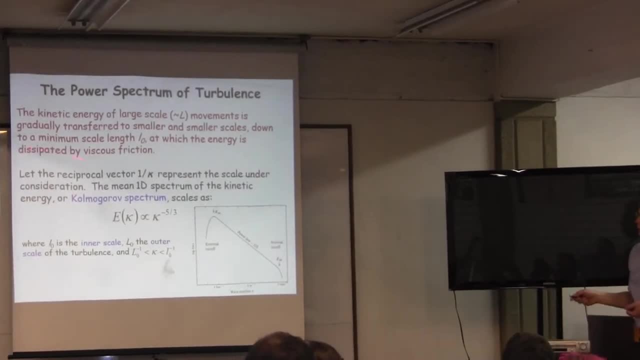 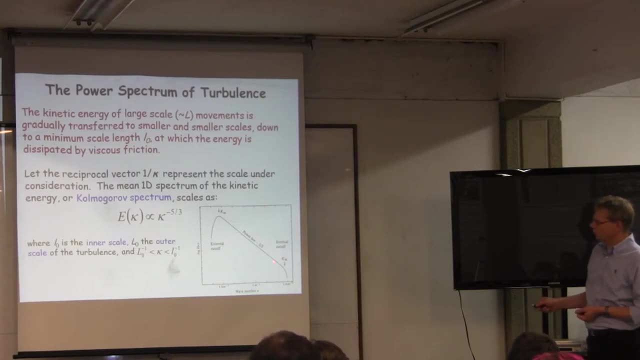 as a function of a quantity of kappa, which is for the inverse of kappa, I assume the vector that represents these scales That's supposed to be. It's hard to give a good explanation, but this is the terminology that we can use. 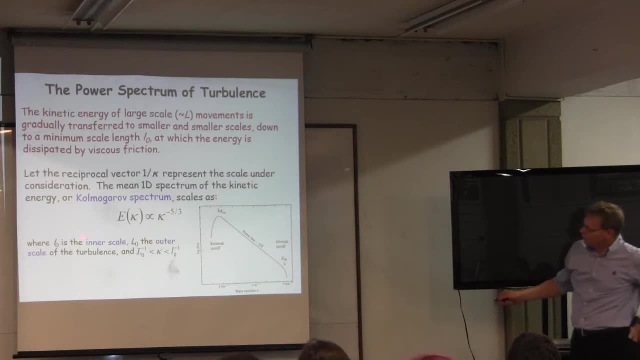 And the main point here is that there are two critical values: the sort of inner scale. here That's the smallest scale, a few centimeters typically. It doesn't go to infinity. We have no turbulence at the micro-meter level. 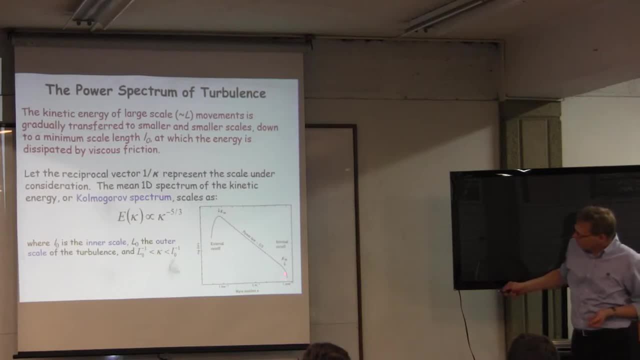 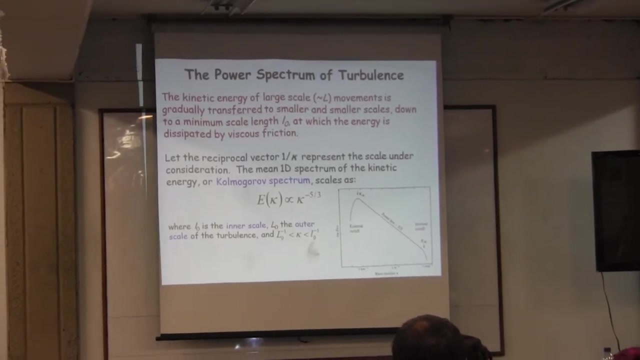 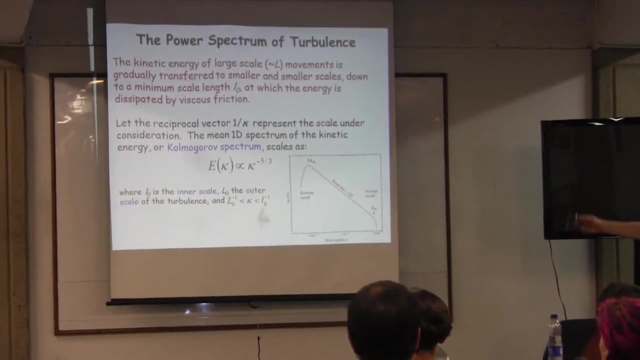 So millimeter here, or inverse millimeter, And then here you have a very large outer scale, And in between here the energy follows the law of. So obviously at the outer scale you have more power than That's it. 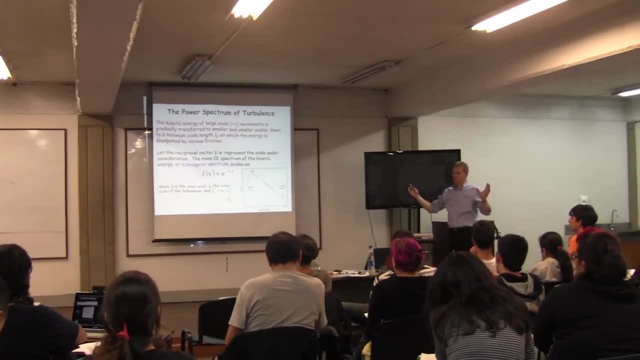 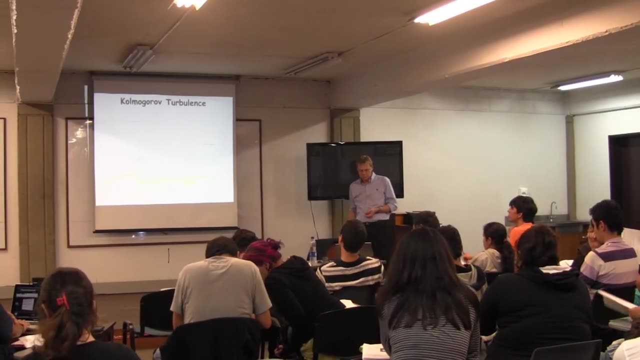 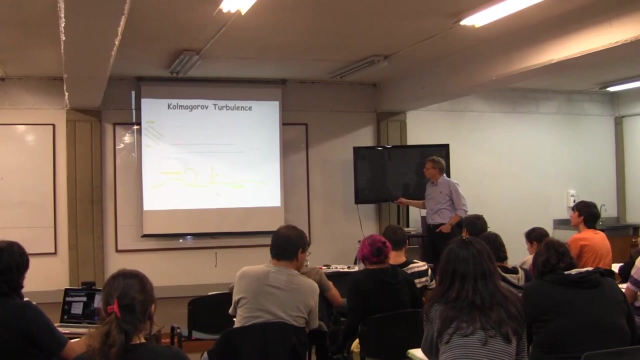 So the turbulence, essentially the turbulence is not random but follows a certain energy or size factor, And this is just illustrated here again. OK, This is our ground, And OK, Now a couple of sources that contribute to the turbulence. 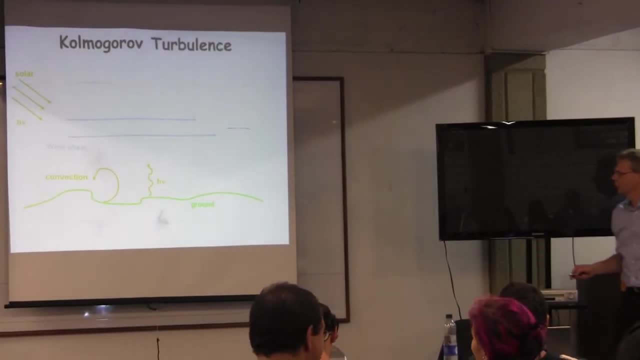 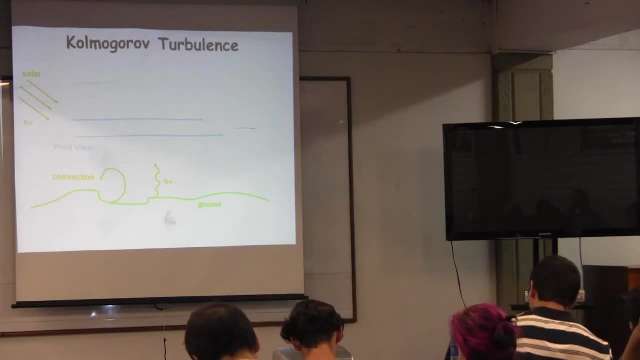 We have winds, lateral winds. We may have convection here. We may have the heat radiation from the ground heating up the air. This is what you see on a hot day from the paved road, But you have, of course, also a strong impact. 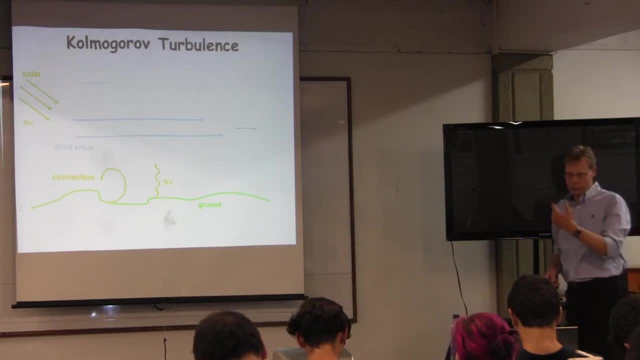 of energy input from the sun, From above, And so this altogether creates some turbulence, Some outer scale. This is the largest one, You know, 50 meters. before we had a process of turbulence, Or this is If we would just take one big block, the outer scale. 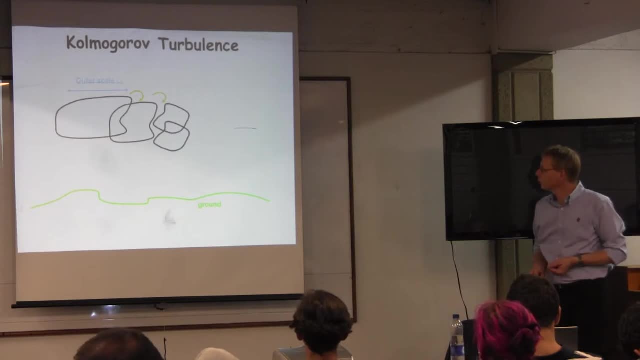 and we follow it in time, it will break out into smaller units, smaller units, smaller units. OK, And this is the turbulence: Oops Down to this minimum inner scale. OK, And that's the simple picture we have of the turbulence. 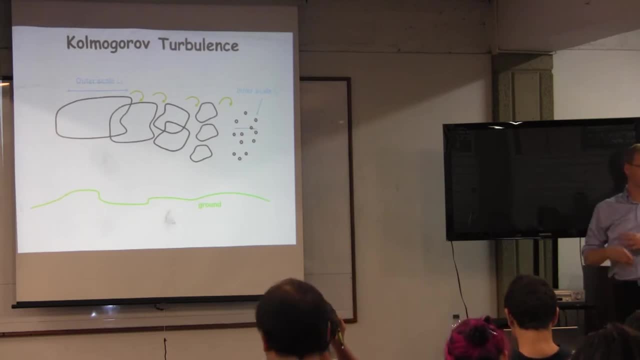 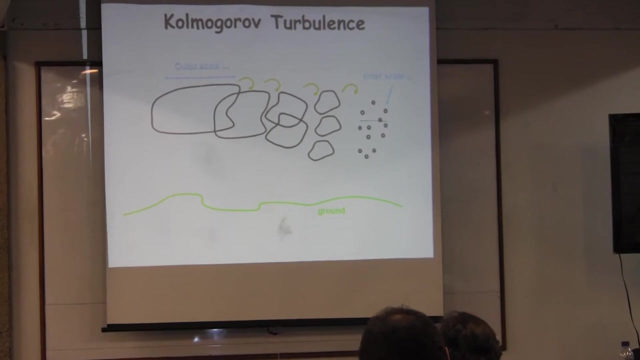 But if we want to correct things we have to find some characteristics. So obviously this already shows- it's a complicated picture- of big areas of turbulence. You have small ones, But at some point you have to simplify it further and So again what the turbulence actually does. 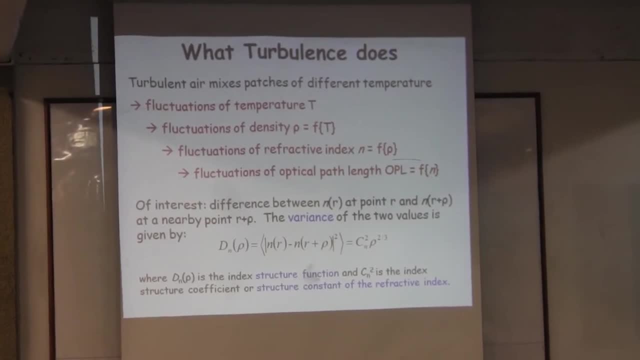 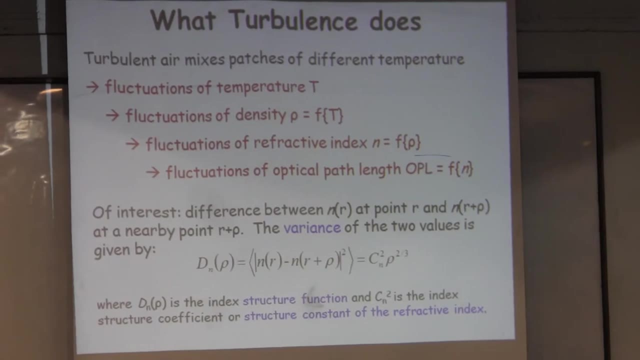 I mean in principle, if the air were either transparent or had a constant refractive index, it wouldn't matter. But what's happening is that our turbulence mixes the air And it mixes patches of different temperatures. Right, It's not talking about many degrees. 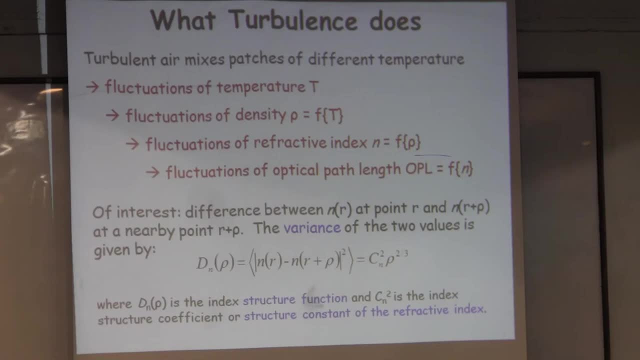 but there are tiny differences between temperatures, between the air here and the air. It's never in perfect equilibrium. So you have fluctuations in the temperature And because of that you have fluctuations in the density, Simply because the density is a function of the temperature. 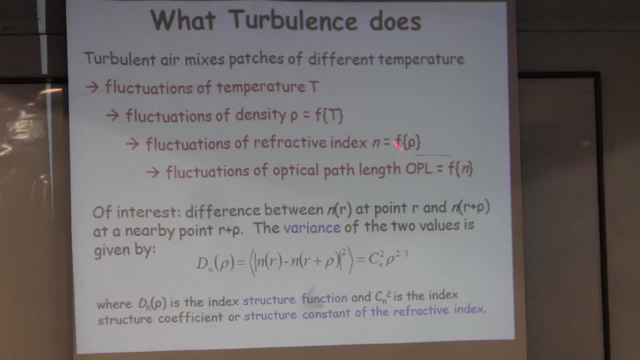 OK, Now, if you have fluctuations in the density, you have fluctuations in the refractive index, because the refractive index is a function of the density. And because you have fluctuations in the refractive index, you also have fluctuations in the optical confidence. 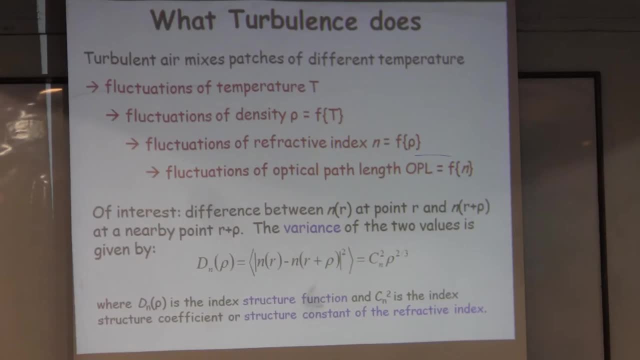 So the light that passes from your distant star through the atmosphere. So obviously this picture we have, this is, you know, a flat wave drop from the object at infinity that goes through the atmosphere, But then that part of the atmosphere has a different optical path length from that part. 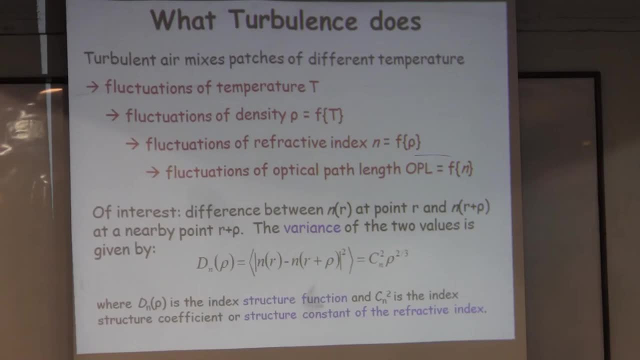 And so your flat wave drop gets distorted, And that's what's giving you these blurred images. And we can, we can look. this is a bit of a map here to make you know about the statistics and the variance, which is, well, yeah, the statistical quantity. 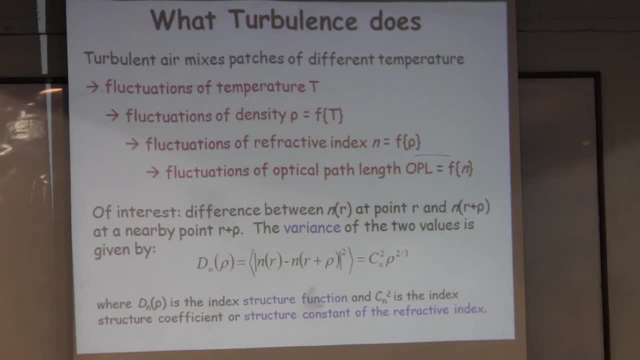 Let's compare the two values. We look at the refractive index at the point of r somewhere, And then there is another, the refractive index at another point, which is offset from r by an amount of rho. So here is one point that's n of r. 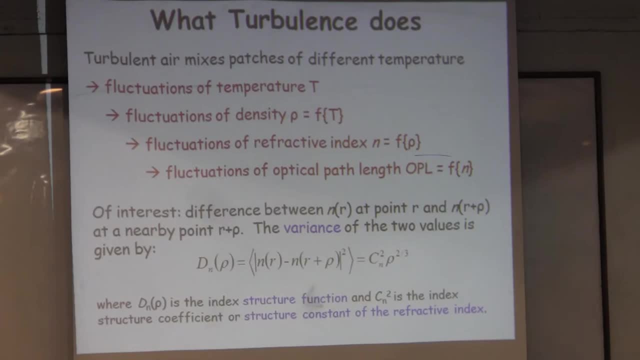 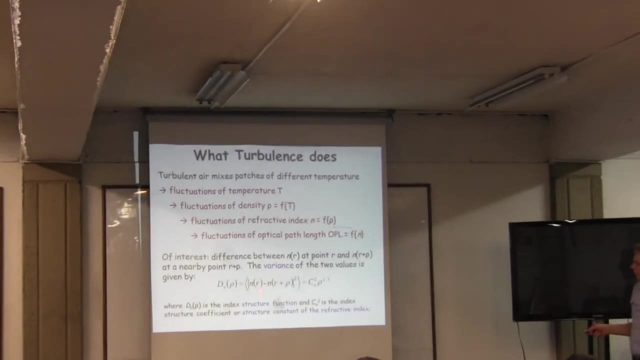 And here is n of r plus rho. Here's the difference between rho And so, and so we compute the variance. Of course we do this for many points. And then we take the. we take the difference in time average. 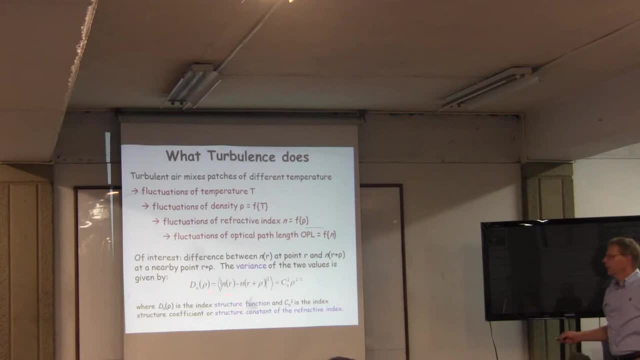 And I mean this can be measured actually. And then this quantity, that's the variance between the density fluctuations- sorry, the refractive index fluctuations is called the structure function of the atmosphere, Or we can also call it the C? n-square problem. 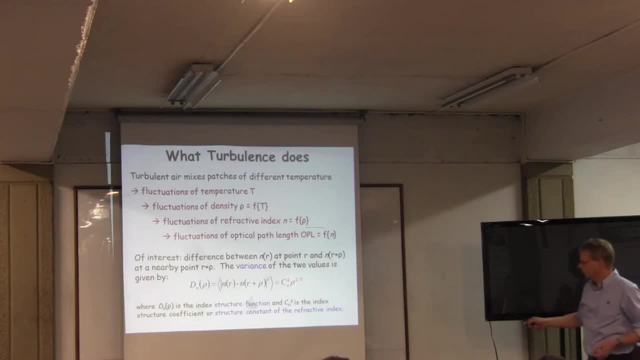 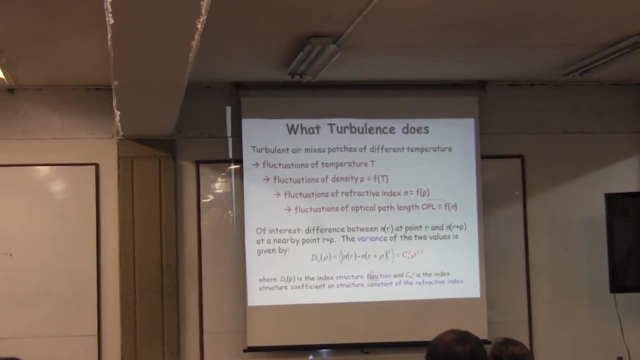 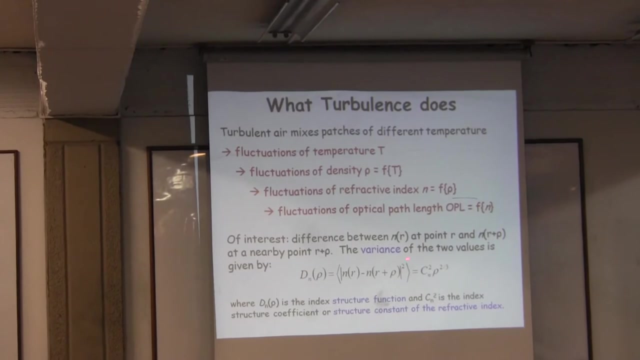 People talk about the C? n-square. That's what's written there- The nicely called the structure constant of the refractive index. Don't worry about this. This is relative to the density here, And the main point is that this quantity here 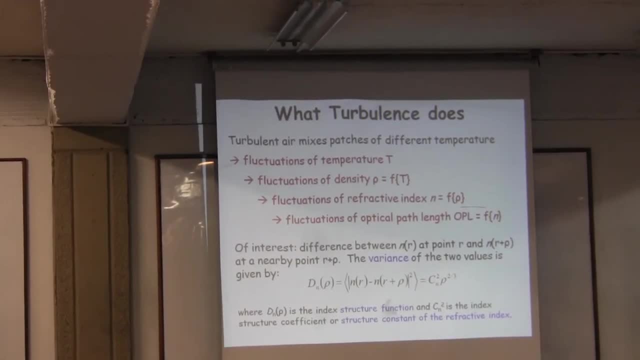 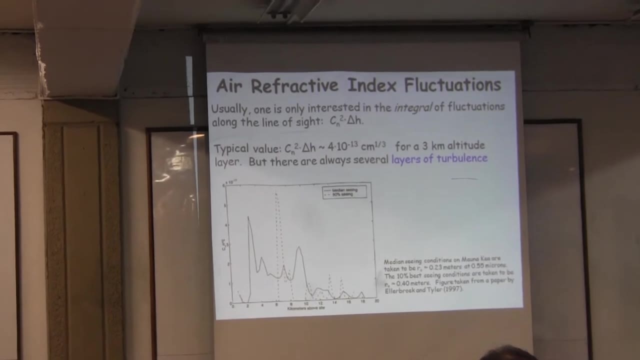 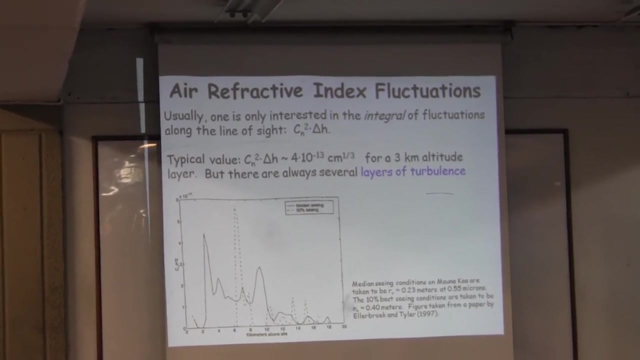 is the C? n-square. That's something that can be measured, And how exactly this can be measured is a. I think it's a topic that's too different, sorry, too difficult for you to just be able to measure. And what I show you here 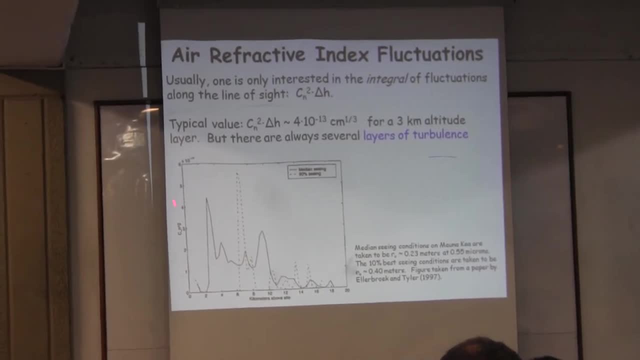 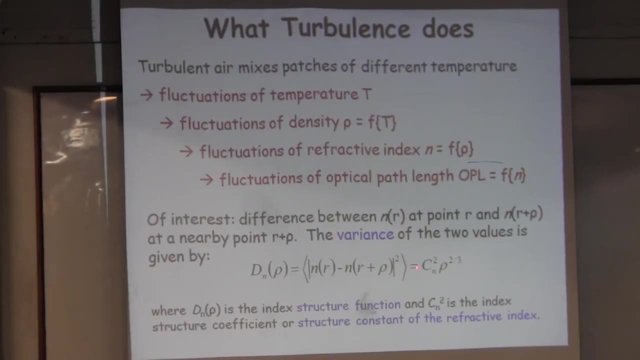 is actually a measurement of this C n-square profile And so again, the mean obviously can match that. if this one is large, relatively large value means the variance is large. That means that between two points separated by a row, 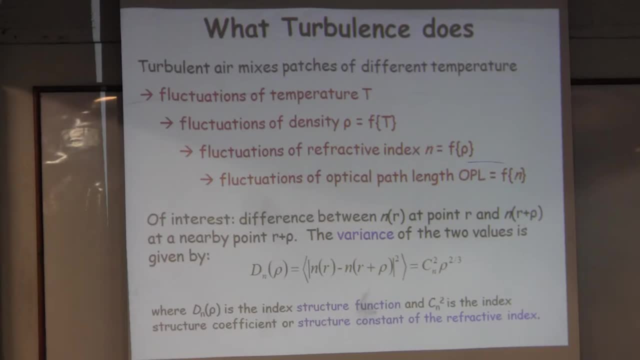 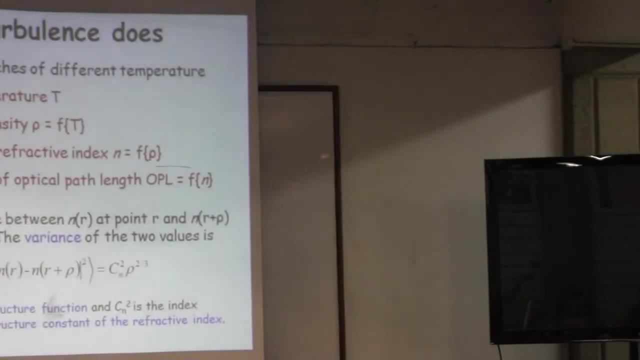 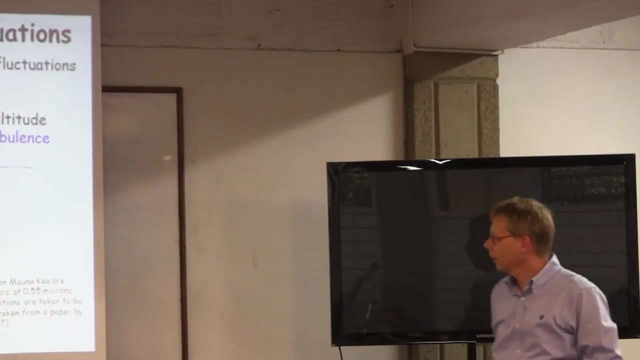 their refractive index differs quite significantly. And if it differs quite significantly, it means it has a very bad effect on your image quality, Right? So you want this to be small, Okay, And I mean usually you don't if you're only worried about the total. 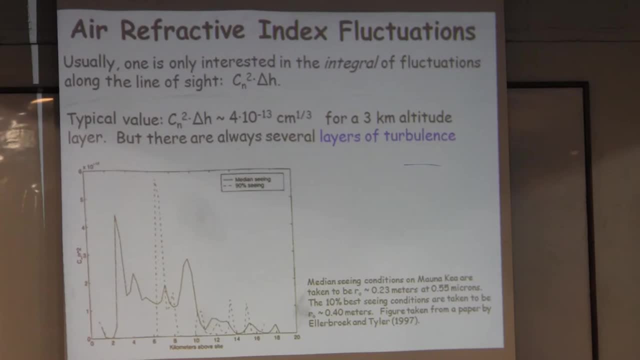 integrated along the line of sight Typical value here. don't worry about that, There will be okay. I think I can say that There will be no test asking about refractive index constant here. This is a. this is a typical subject. 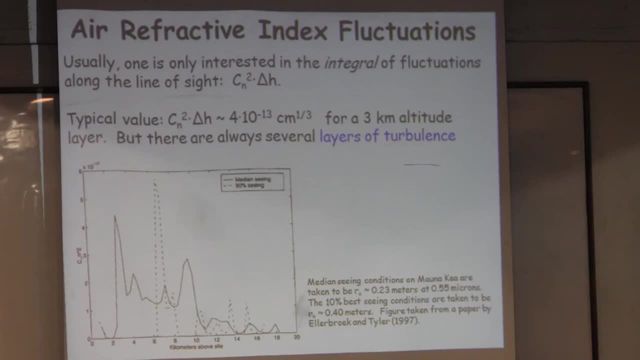 and I don't expect you to get this in this course immediately, But I thought it's useful to show because the measurements show how this structure function varies with height. So on the x-axis here you see the height in kilometers above the sun. 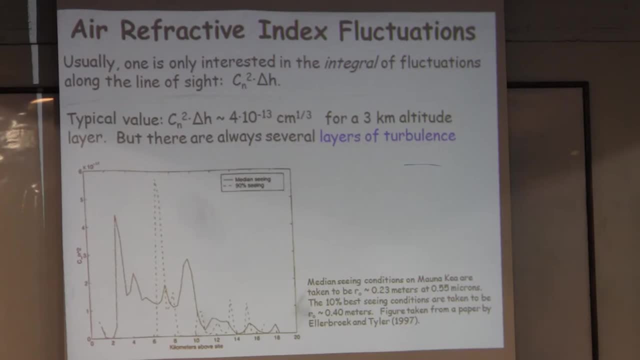 This was actually measured from Mauna Kea, which is one of the prime observatories on this planet, And here is the sea and spirit profile and here is the height of the observatory, And what you see here is that there are some peaks. 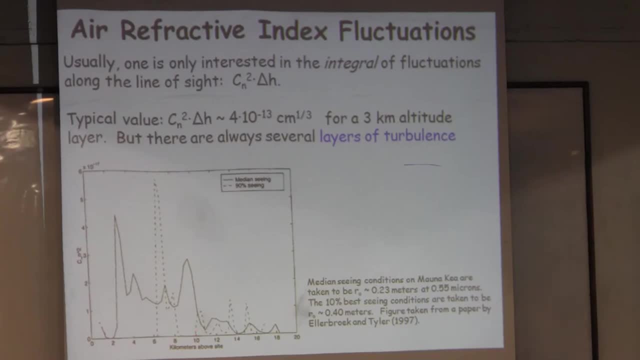 And what it means is that most of the turbulence, like we said before, if this sea and spirit profile is large, that means that the density or the temperature, whatever- is very different between two points And that means that it has a very bad effect. 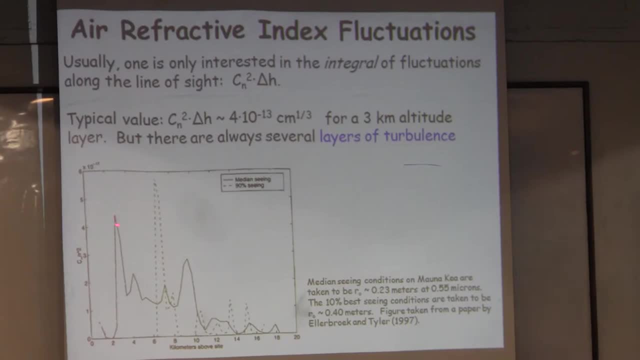 on your image quality. So if this is high here, that means that a lot of the sea, a lot of the image marine will be produced at this point, some three kilometers above ground. And then there's another one at high layers. 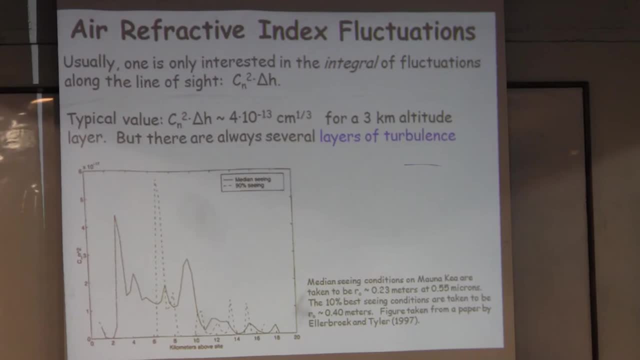 let's say nine kilometers with respect to the risk. So actually if you could compensate for those two, you would already improve your image quite a bit. And that also changes with season, So it's not like your turbulence is always created with the same layer of the atmosphere. 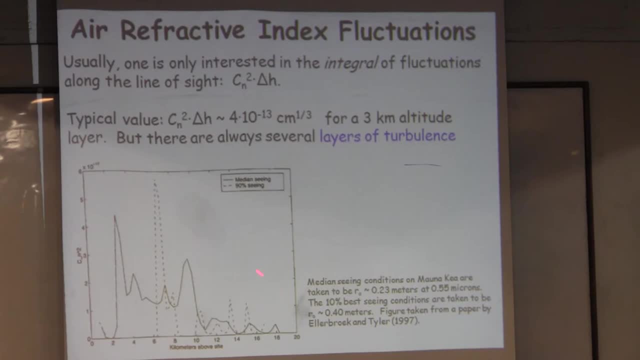 So for the same observatory it varies from day to day. So if you take only the nights with the very best sea, you can see that this one is completely gone. So apparently there must be some condition in the atmosphere where, on average, 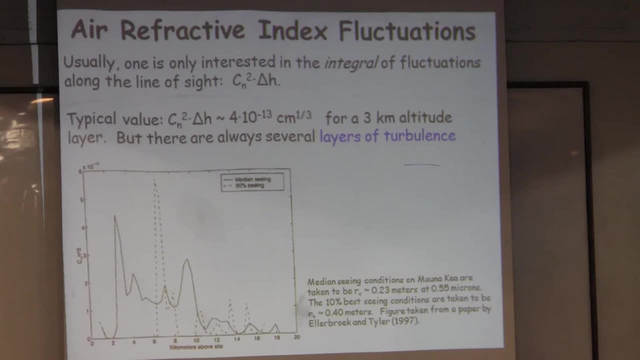 you have some winds at low altitude that you can't see, But if you take the best nights on Mauna Kea, these components are completely gone. so you only have some very strong component at seven kilometers away. Maybe some airplane just came by. 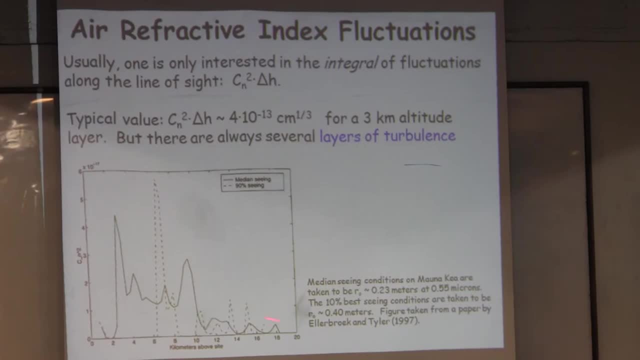 and added some turbulence. I don't know, But it's very dynamic, it's changing all the time and you need to compensate for all that. So the main point I need to take away from this slide is that turbulence is not constant in every layer. 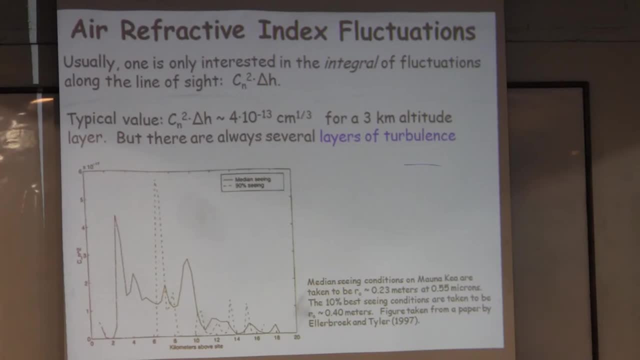 It's usually some very specific layers that contribute most of the sea, And the very dominant one in all observatories usually is the ground level. So that's one of the reasons why people try to build a dome around to shield it from the wind. 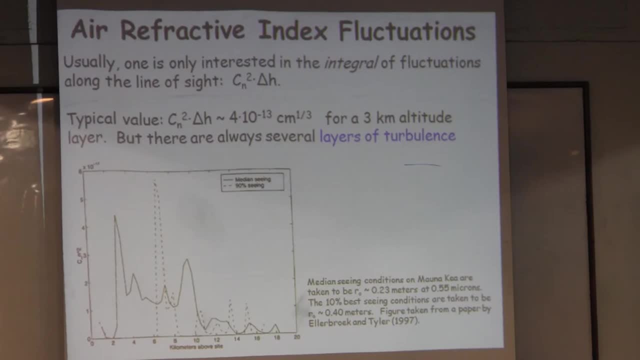 or to put it actually up on some, I mean many of this Back to the 15 meters. many of these scale lengths are mostly at the ground level. So if you build your big telescope at the top of a tower, that's 30 meters up. 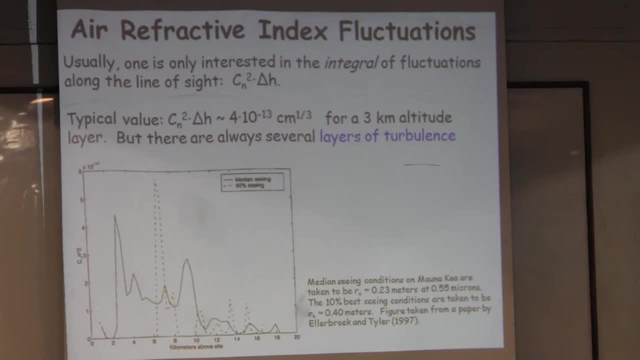 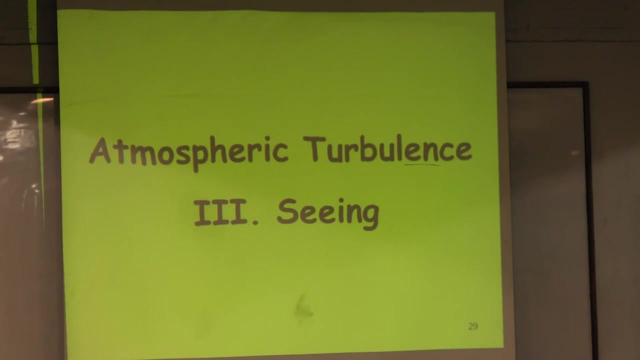 the sea will already be much better. And yeah, of course that's expensive. This telescope weighs a couple hundred or thousand tons. Maybe the tower is bigger, Okay, but it's turbulence occurs at some distant, a distinct altitude, and it's changing with time. 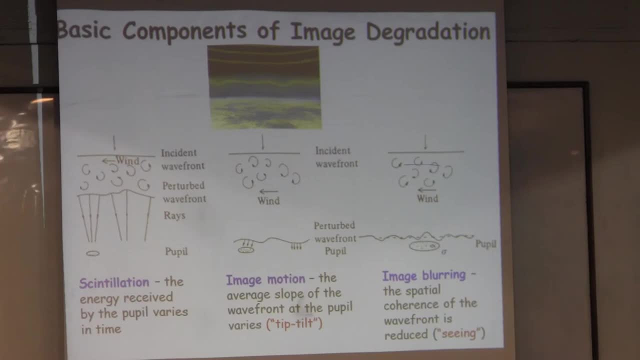 Okay, now from turbulence. we've seen these effects before, So this should not depart from that part. One effect we've seen in this little movie event that I showed you before: You saw the clouds, the blob moving around. That's called the image motion. 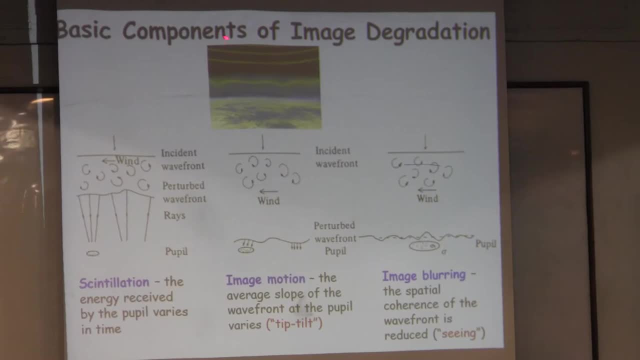 And well, one way to look at this is to say we have an object high up there, We have an almost parallel wavefront coming through to the atmosphere And then it goes through the layers of the atmosphere and it gets distorted. So the ideal flat wavefront would give an ideal point source. 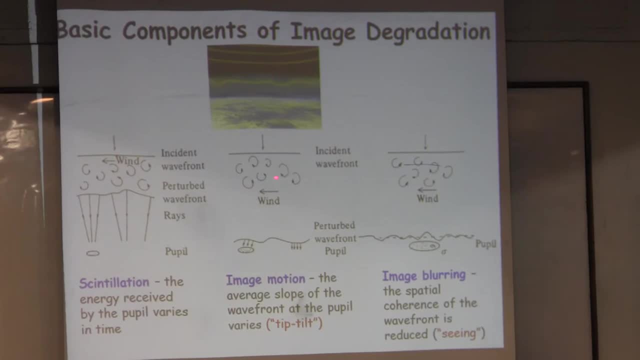 But now that we have a distorted wavefront, we will see the blurring of the image, Now that image motion is essentially due to flat parts of this distorted wavefront. So if let's say we would look through that part of the wavefront, 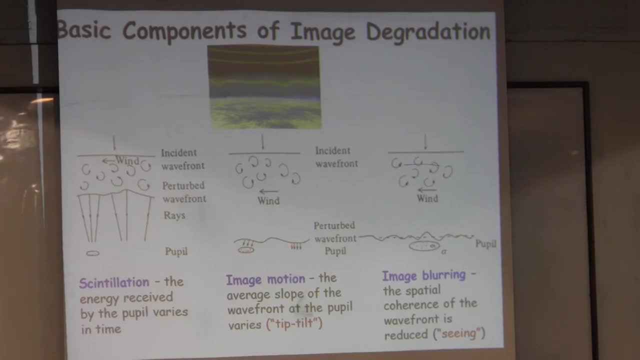 then we would see the speck at the cloud here. If the wavefront, say, moves by and the angle or the inclination is a little different, it would move everything just by a small angle And that means it moves the source around. 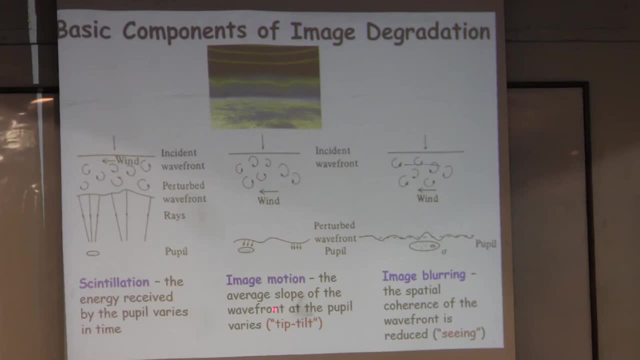 And that's what's called the tip-tilt motion, And this is also important because many telescopes, especially the smaller ones, are equipped with a tip-tilt system. In fact, my pocket camera has an image stabilizer which essentially does the same. 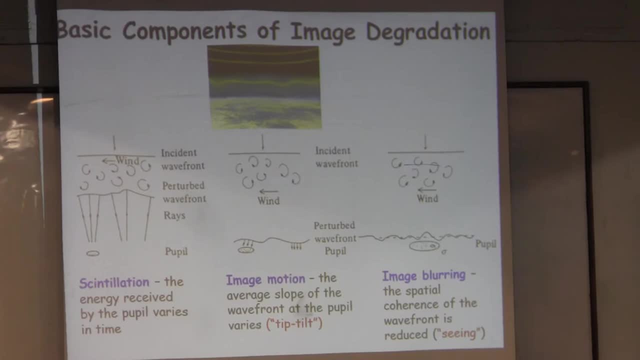 only that it offers, in that sense, like whatever Canon pocket camera is not supposed to correct for the atmospheric distortion which is me shaking while I'm taking photos, But it's essentially the same principle: It tries to stabilize the image because there is this fundamental. 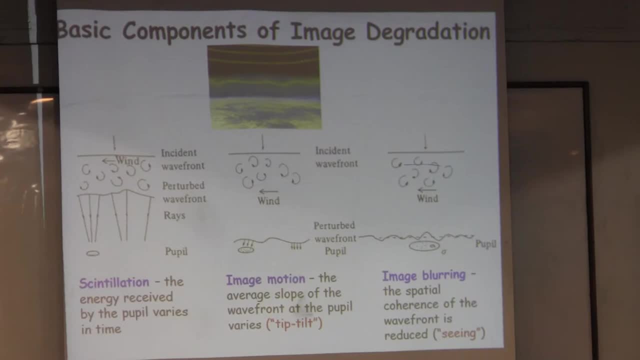 component that moves the image around, and simply by tilting and tipping, in this case, parts of the wavefront, in another case, whatever. And then there is the image blurring, which is simply due to the fact that, because there are many turbulent cells, 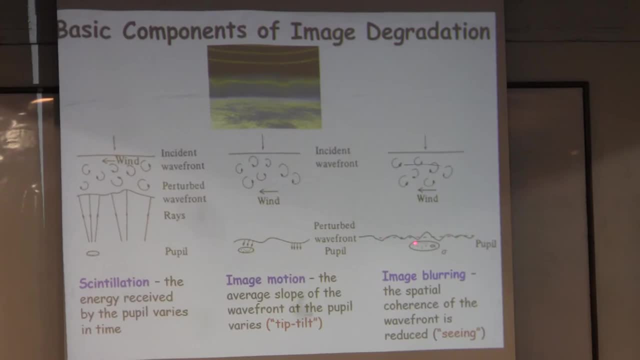 the light comes at different angles. And there is the third fact that if some of the more of the light is concentrated- and in this case, here I mean, imagine you have a telescope here- The telescope would only take, would have that size. 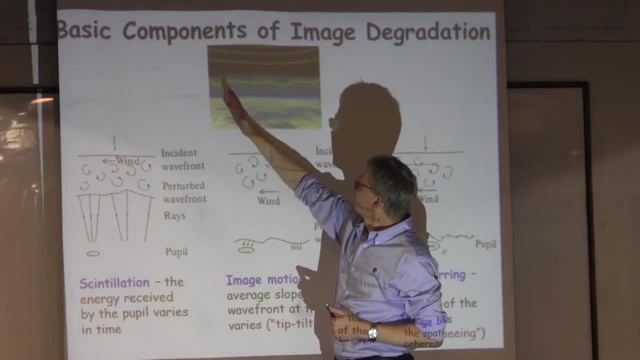 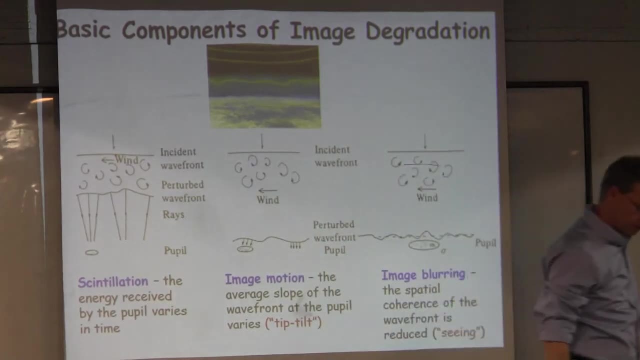 So it would only see that part of the the wavefront. But the grid is moving this way, so the gradient will change all the time. And when the gradient changes we have the image motion, we have the image blurring with time. 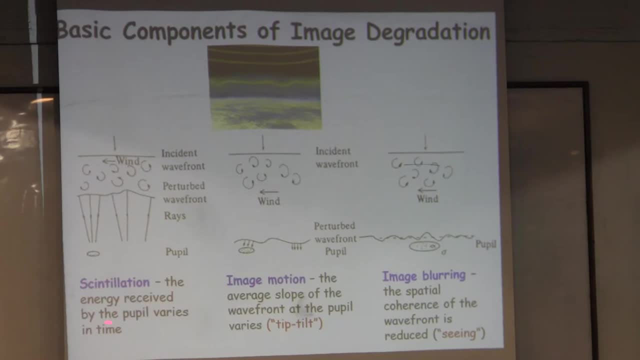 and then there's also an effect called scintillation, simply meaning that, of course, if you have more rays coming being focused here, then this one appears brighter, and then here again it's. This is sort of an effect. 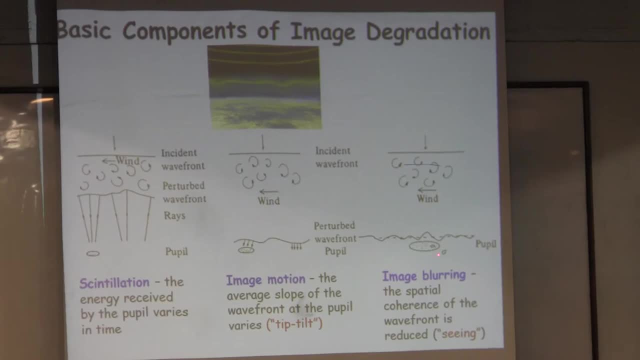 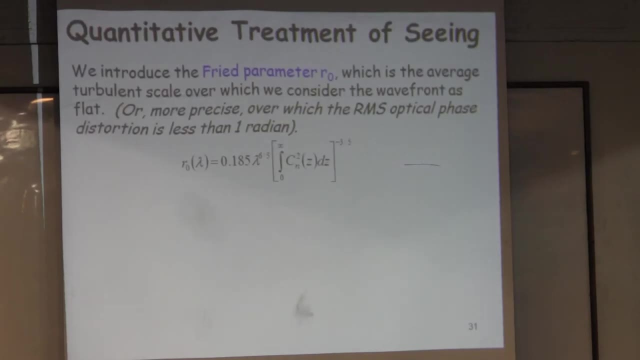 you should not worry too much. it's scintillation, But image motion and image blurring is something that will force us, it will disperse. Why scintillation is not as important, since it's a variation in the primacy of sources. 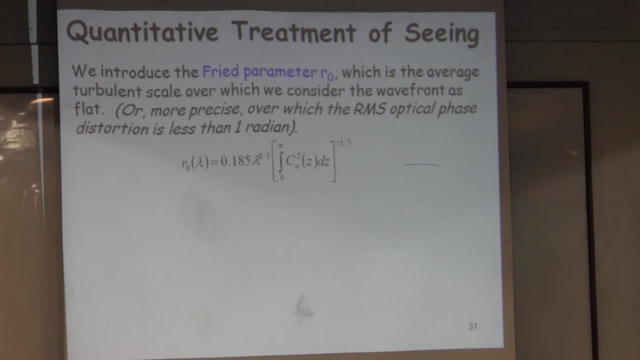 Yes, In the end you take a long exposure and you can't reach up, So every Okay. so so there is a free parameter that I will introduce. It's named after an optician Fried, And that will take a while. 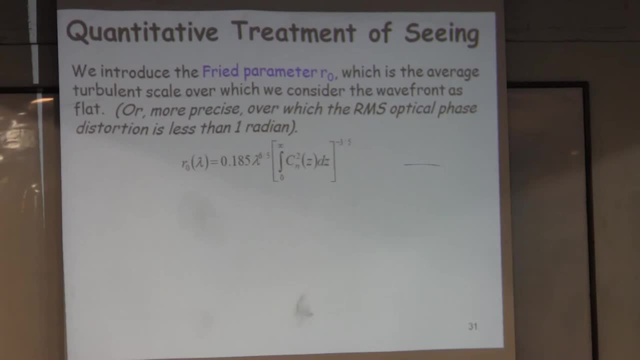 until you appreciate what it means and then it actually can be used. So the R0, this free parameter often called R0, that's the turbulence scale over which we consider the waveform as flat. Okay, so if I go back one, 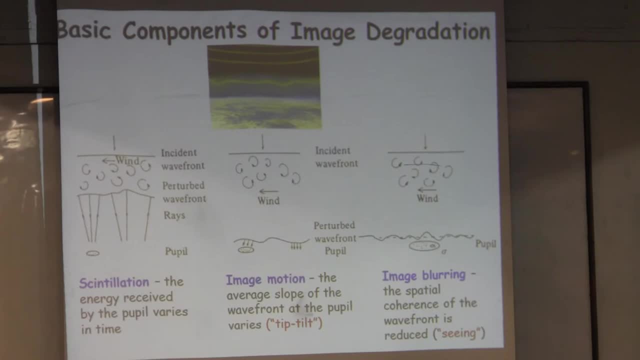 oops, one slide, Okay, so before. okay, if I had a flat waveform here from a star at infinity above the atmosphere, R0 would be huge, right, It would be almost high. Now it goes through the atmosphere. 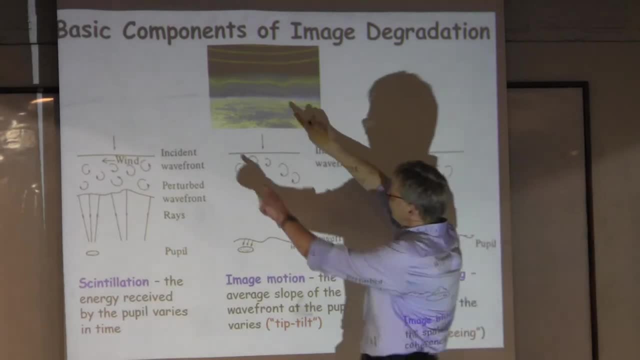 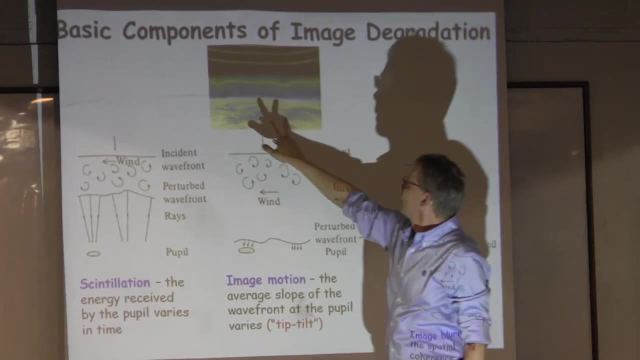 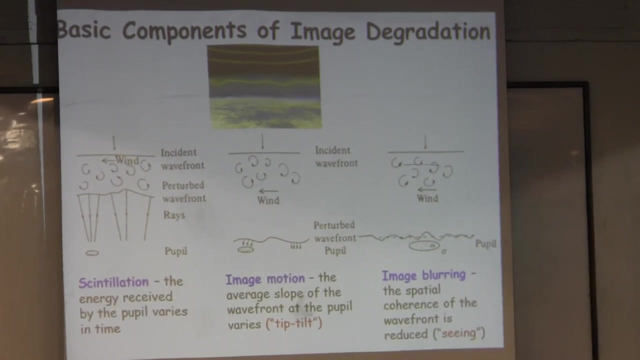 and I can see that. first, maybe this part of the waveform is pretty flat. It certainly isn't flat here, So I could maybe say: well, this size is? I consider the waveform flat, or more precisely, we want to quantify it. 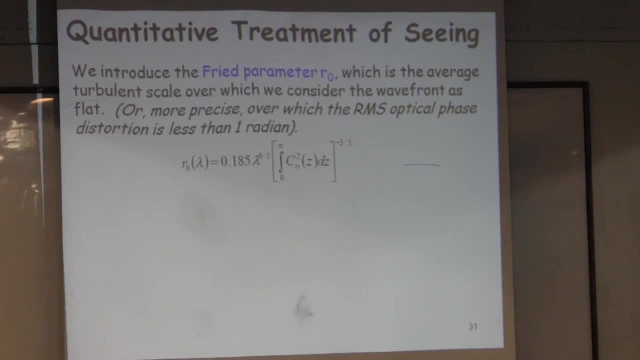 We said, the waveform is distorted, so there is a phase shift between different parts of the waveform. Some parts of the waveform are simply ahead of phase or delayed because of this different optical path length through the atmosphere And if that waveform error is less than one radian. 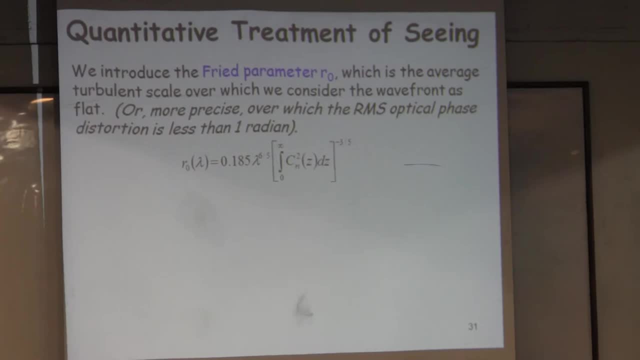 meaning one radian is 60, 70 degrees or something, meaning that one wave is shifted by 60 degrees in phase with respect to the other. that's not that much, Of course. it has to be much less than one wavelength. 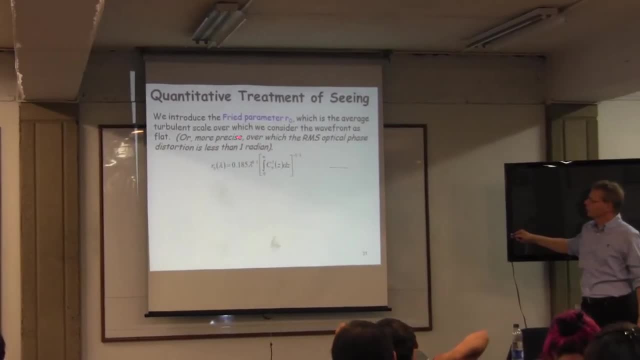 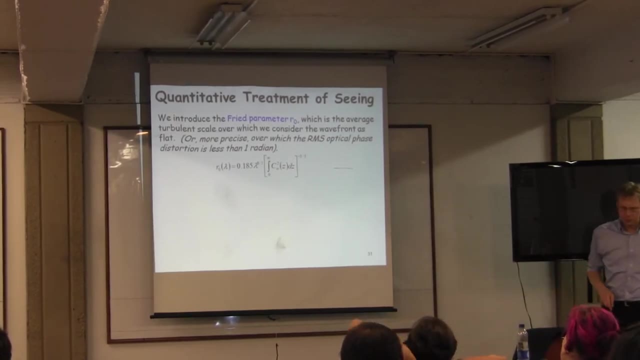 but if it's less than one radian, then we consider the waveform still as flat and that defines then our parameter here. Analogically, you could calculate this parameter here from: I'll show you some more inspiring pictures in a few minutes. 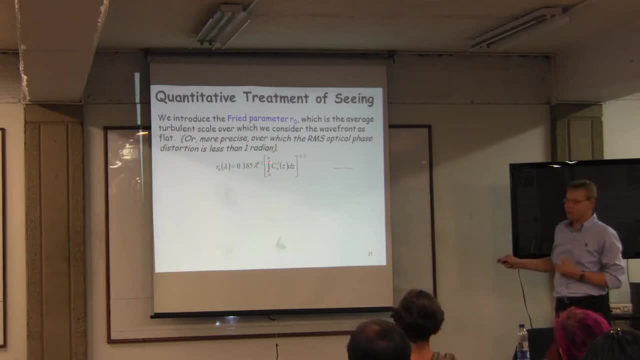 But you can. I think it's better to start with the definition up front. you can actually calculate it very precisely if you would have this structure constant of the atmosphere that we used before, and then if you plug in here the right numbers, then you can calculate. 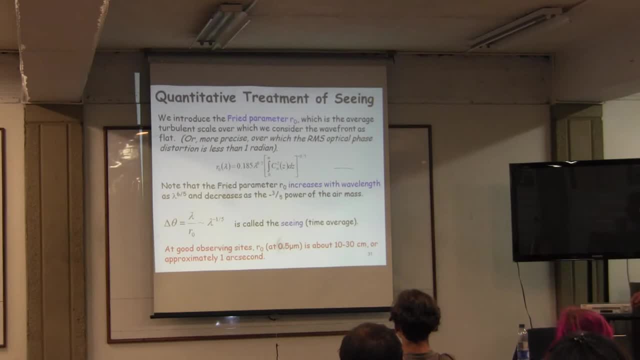 what are not this: What is important to take away from this formula is that this parameter, the value increases with wavelengths, as you can see here, are not proportional to lambda, to the sixth-fifth power, And it also decreases as the minor three-fifth power. 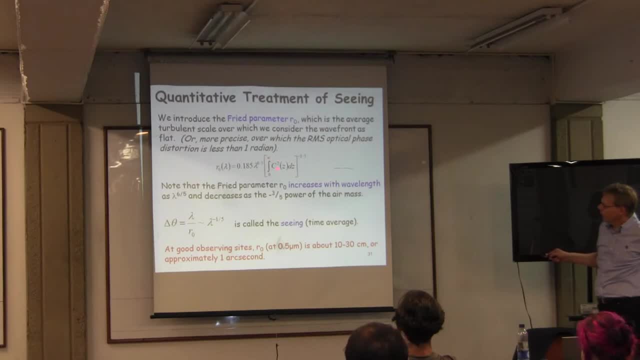 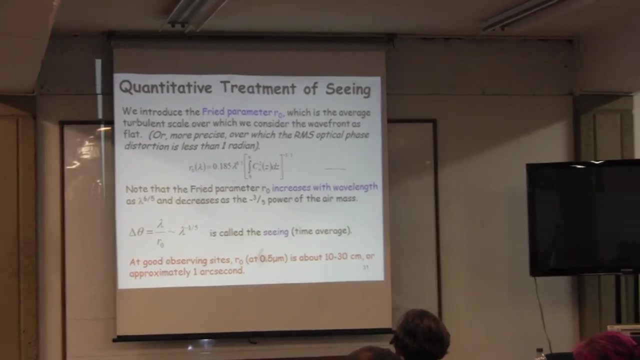 of the air mass, because this one depends. if you draw a couple of slides back, you can see that this one depends on the air mass. Okay, so what does it mean actually? it decreases with wavelengths and decreases with air mass. 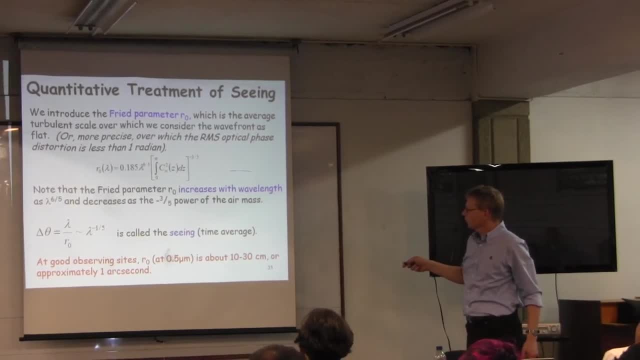 Well, if you okay, it decreases with the minus power, so it increases. An easier way would be to say it increases with air mass, right, Sorry? So okay, that means that this free parameter shows us the size of this chi. 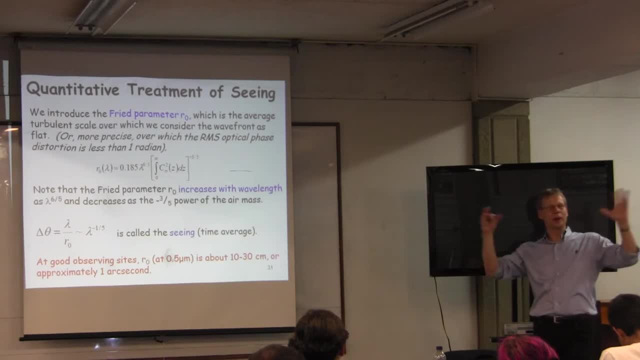 that gives us a flat waveform. Ideally we would like to have the whole chi be flat. So ideally R0 should be very small. Ideally R0 should be very big. Yeah, If R is big, you can consider all the way from to be flat. 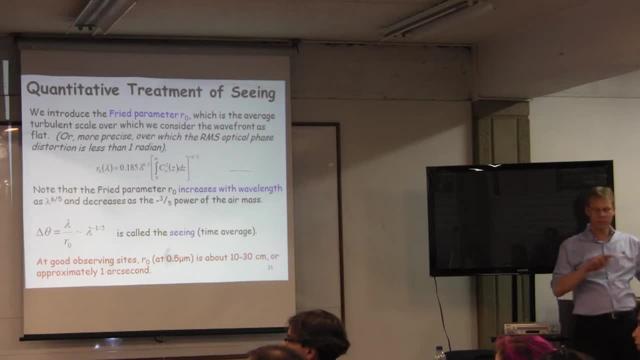 at large scales, right. If it's small, then you only have patches that are flat. So R0 to be large. Yeah, I mean to give a typical scale axis. at optical wavelengths it's typically 20, 30 centimeters. 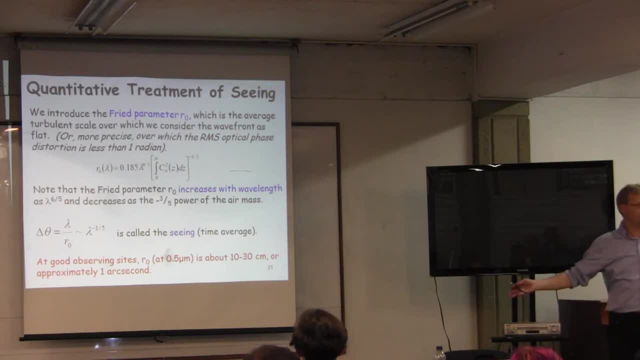 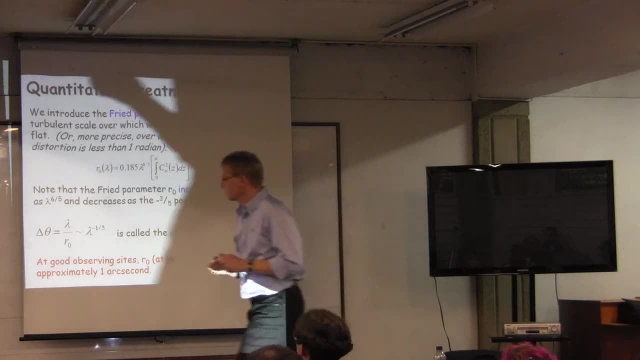 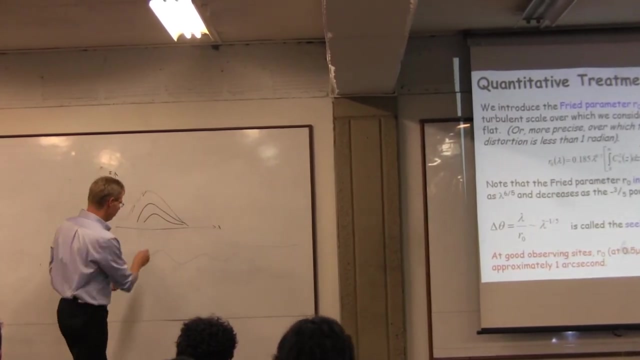 And that shows the whole problem. If you have a big telescope, a telescope that's bigger than 30 centimeters, right, let's say: this is your waveform, Right, It should be. this is what it should be, and it's flat from here to here. 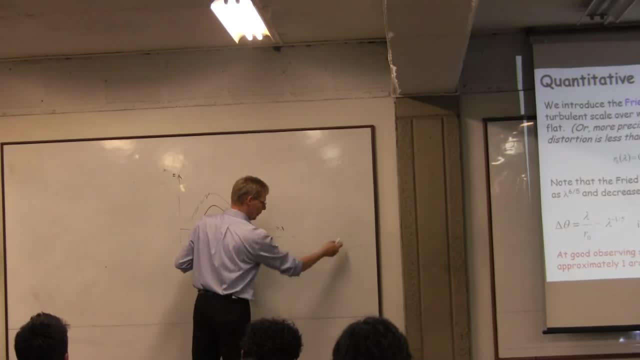 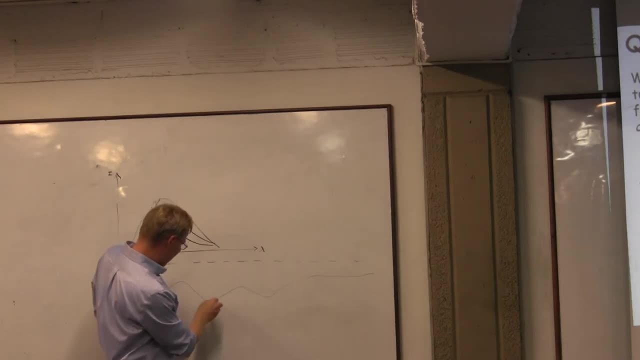 So R0 is big right, It's the whole distance. In this case, I could say, well, it's approximately flat from here to here, and it's approximately flat from here to here, and it's approximately flat from here to here. 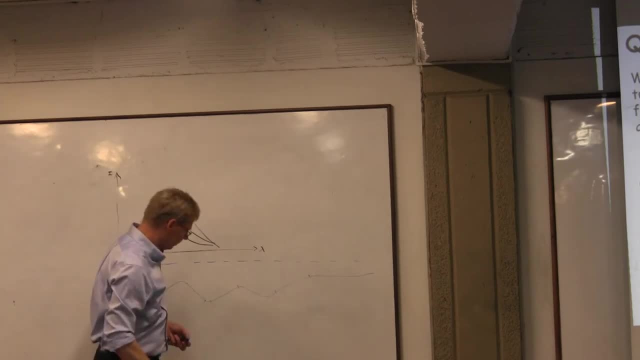 Okay, But not the whole way. Now my telescope, let's say, is big. This is my telescope again. And this is where the problem starts, Because if this were the, let's say, okay, this is the ideal waveform. 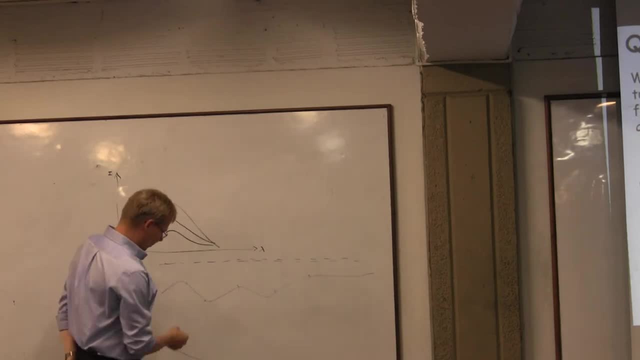 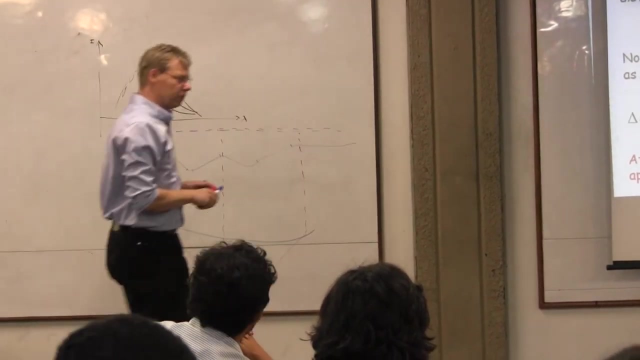 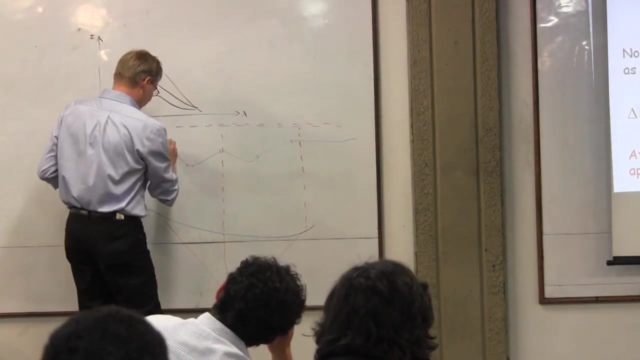 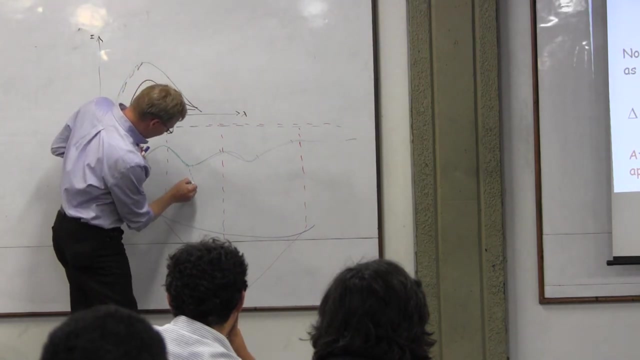 Okay, And my telescope optics would then, okay, focus the light into one spot. Okay, This is the ideal, the ideal case. And now, now, this is the, the terminal waveform, And, okay, the light from here actually is the mirror there. 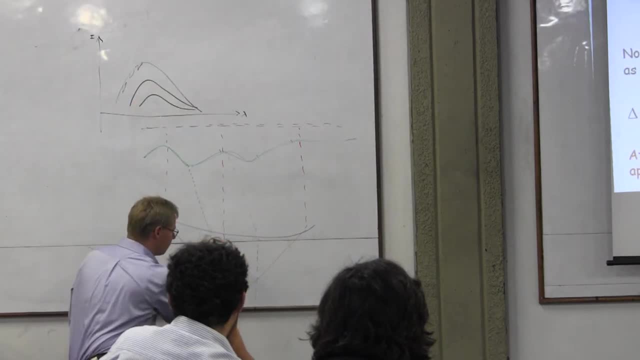 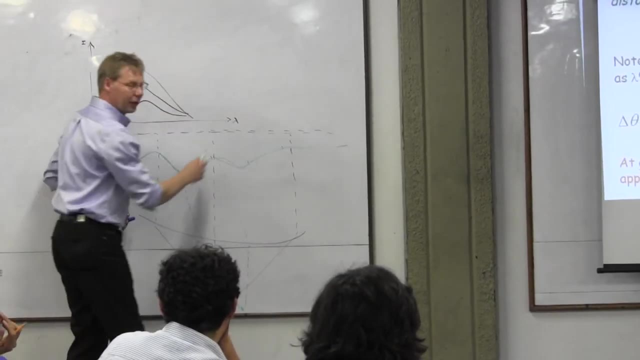 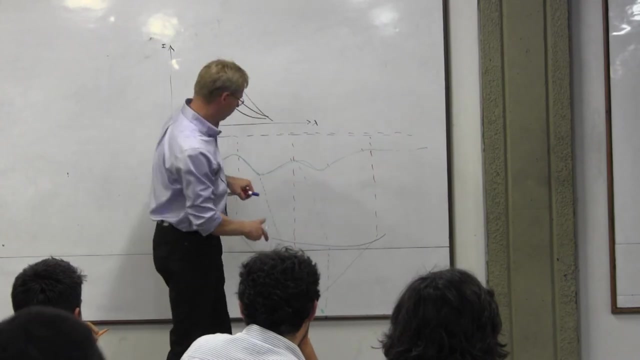 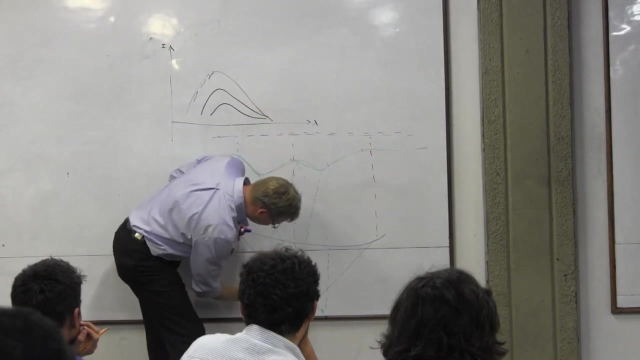 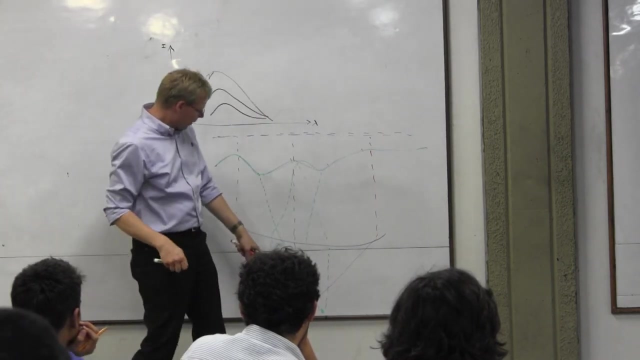 And it will make an image here Now. unfortunately, my telescope mirror is bigger than R0,, meaning that the light from that part above the telescope will actually travel this way, Yeah, And be focused here. So in the end I have. 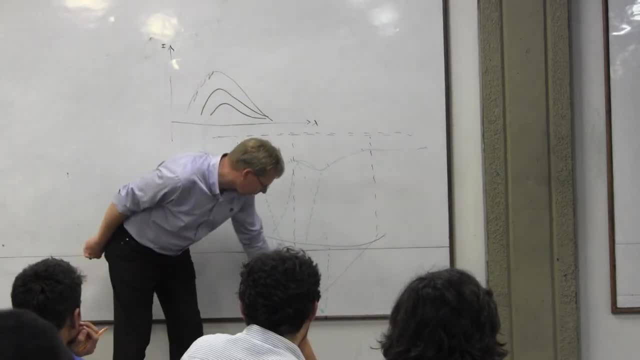 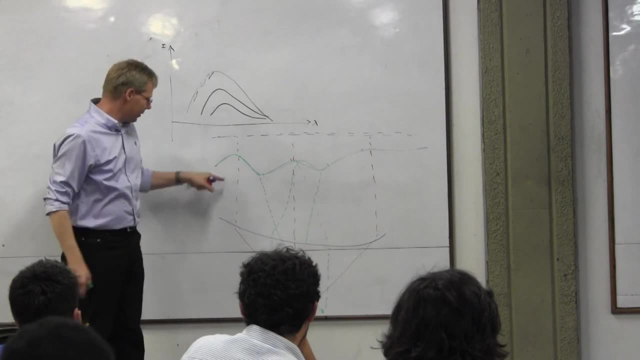 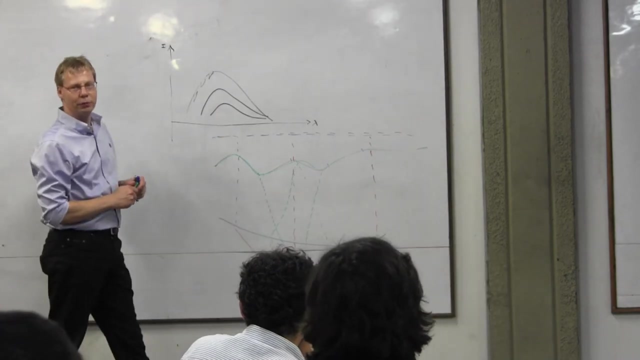 in principle. I have a couple of images from my star- One here, one here- and continue that And unfortunately this thing is also moving In time. So these things are moving around And this is what you saw in the movie before. 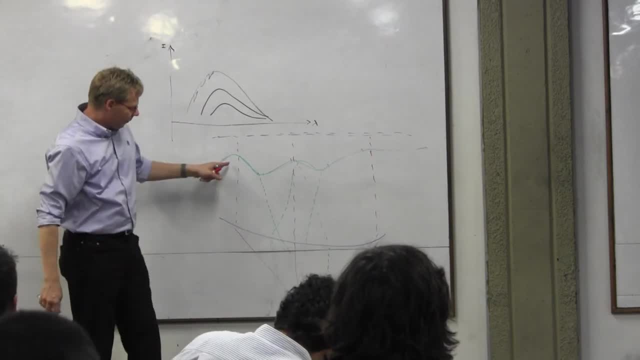 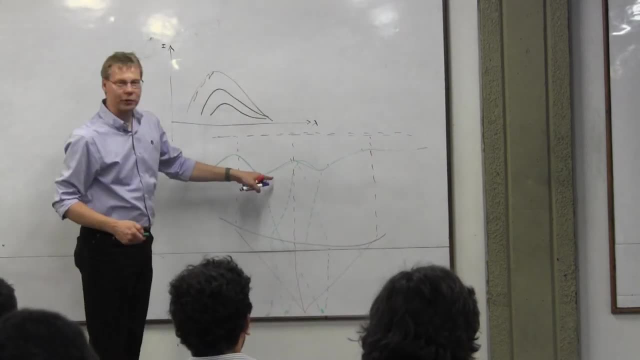 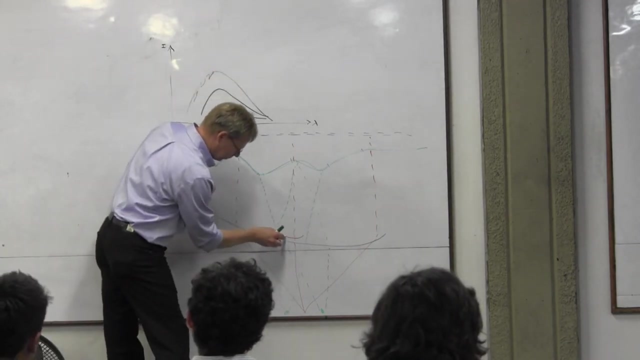 Right, So there's constant motion. And now if you, if you had a telescope- now this was our big telescope- If you had a telescope that were smaller than R0, so if you had a telescope that had only only that size. 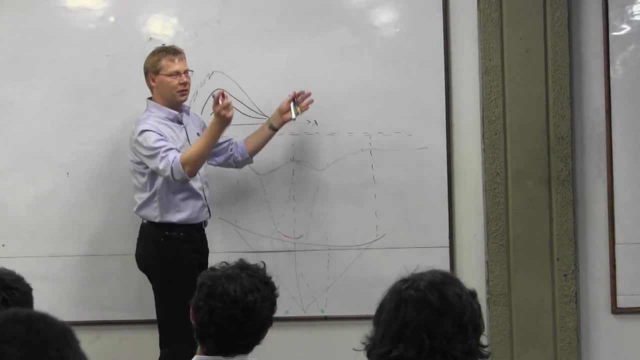 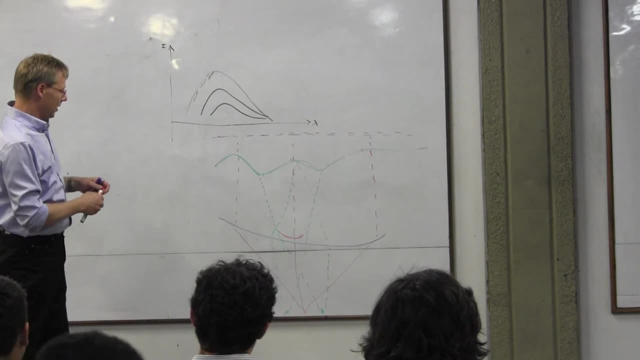 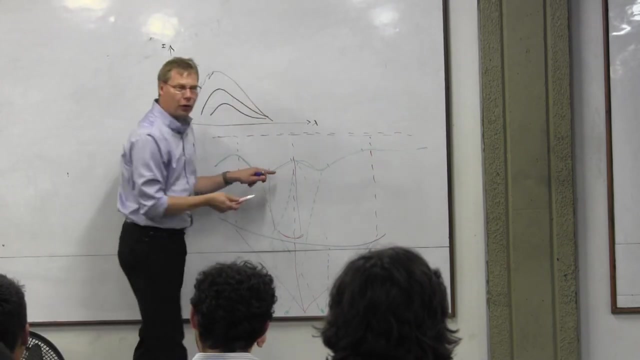 right If you put back your telescope or whatever, maybe inches or so. Yeah, Raphael's telescope, Sorry, Raphael's telescope. Yeah, Yeah, Okay, That that telescope would only see that part and not know that about much about turbulence. 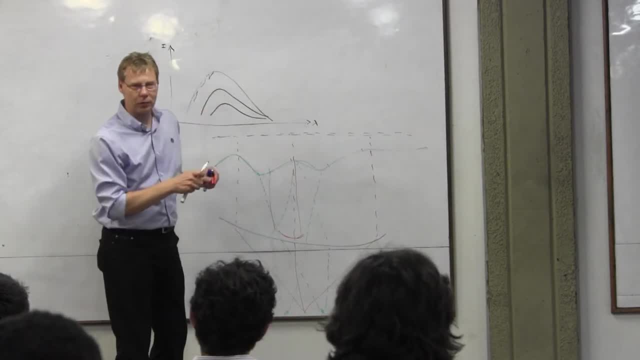 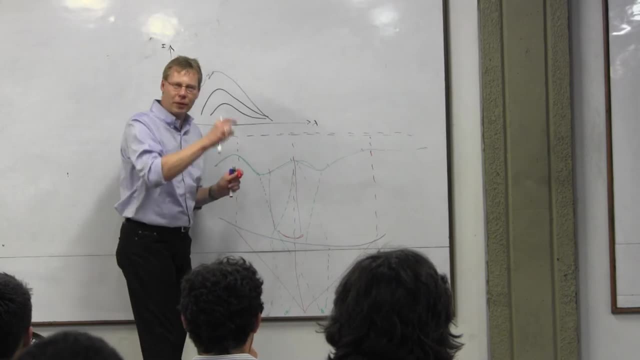 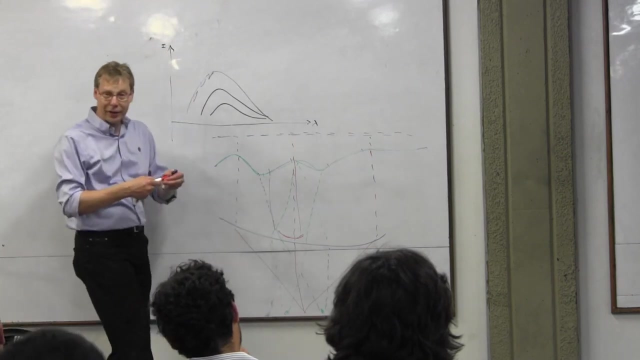 It would what the only effect? because you only have that one R0, one free above your telescope. you would only see a sharp image, but moving around, And that would be the simple Tilt-Tilt component. So, in principle, if Raphael could, 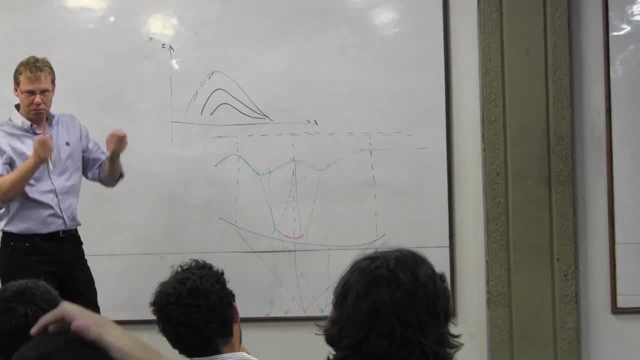 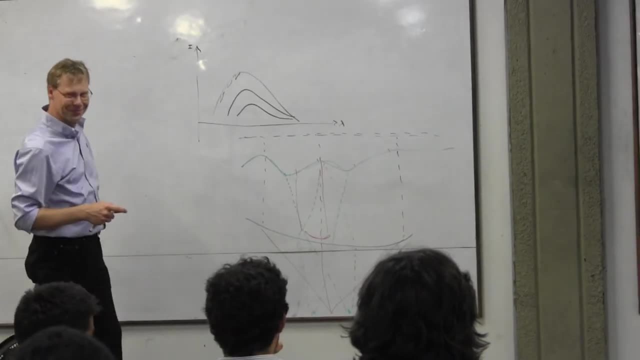 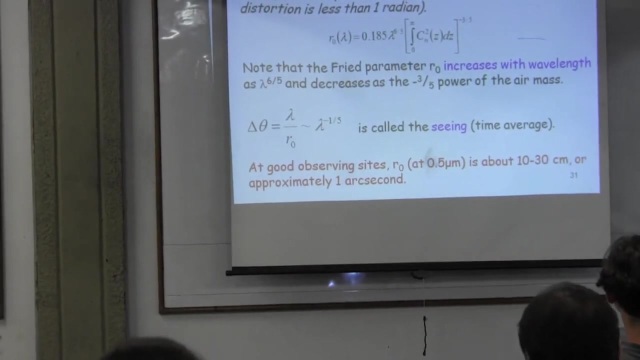 could follow the sky and move the telescope very quickly- so a millisecond scale- then he would still get a sharp image. So what He's only going to make it Right? That would be the same frequency of the of the truth. 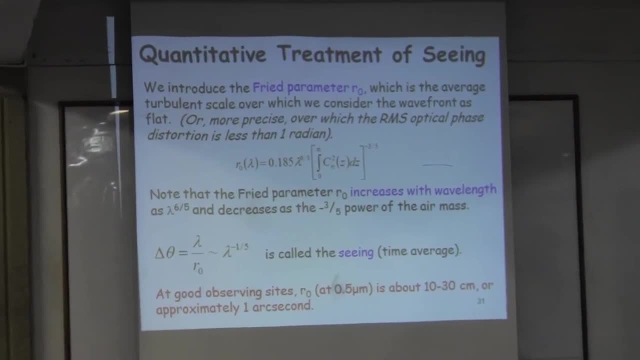 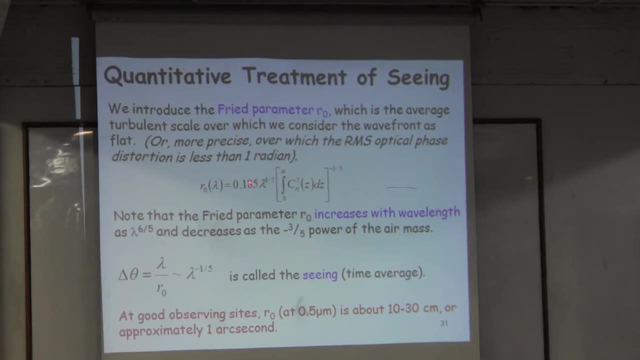 Yeah, Okay. So so what? this means? we want the R0 to be large, The larger the better. And we say: we see that it scales with wavelength. That means that if you go to longer wavelength it increases, And that is simply. 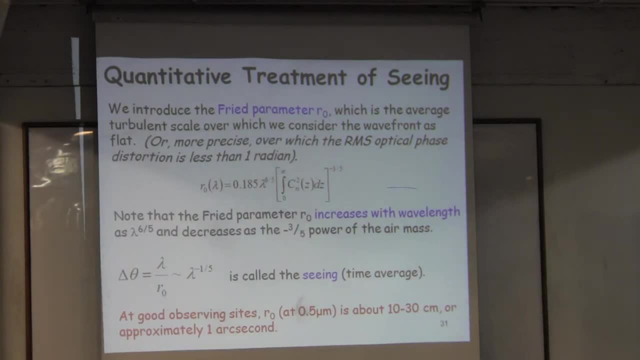 that? how shall I say that In simple words, longer wavelengths are more tolerant to wavefront errors, Although we see that all the time. I mean if you, if you polish it, you, you, ultraviolet telescope and go, I mean. 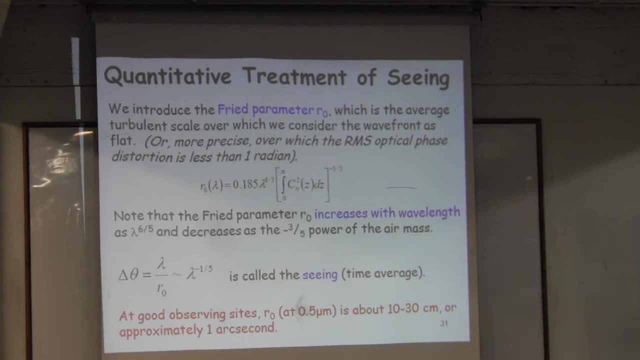 if you, if you polish it, you and go. I mean, look at the radio telescope, right, It doesn't matter if you walk around across it. James Bond has done it in movies. It's still a telescope. If they wouldn't have allowed. 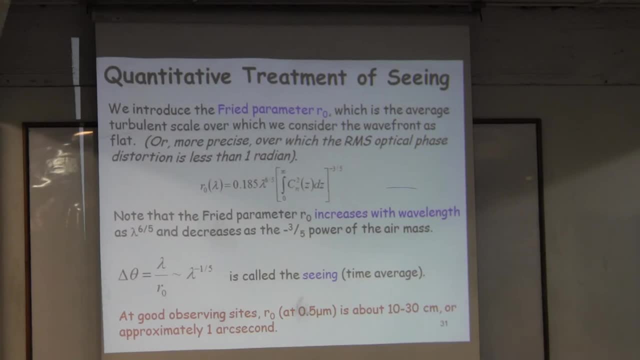 James Bond to walk on an optical telescope, because the, the, the footprints, destroy the image quality, And that's simply because the deflections and it's not in the telescope area or in the atmosphere if they're small compared to the wavelengths. 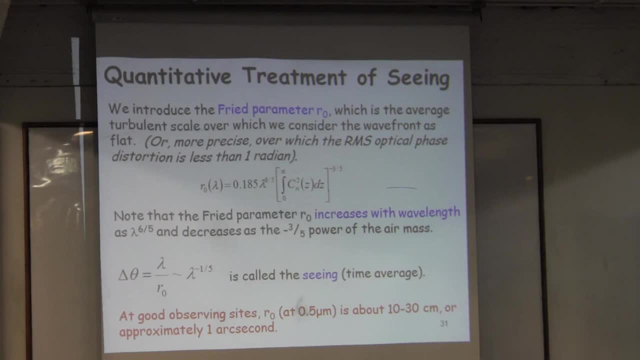 they don't matter, Right, And? and this is seen in this formula, You know, this is seen in this formula here: If, if you go to longer wavelengths, the effective scale over which the wave, the wave forms, can be considered flat, 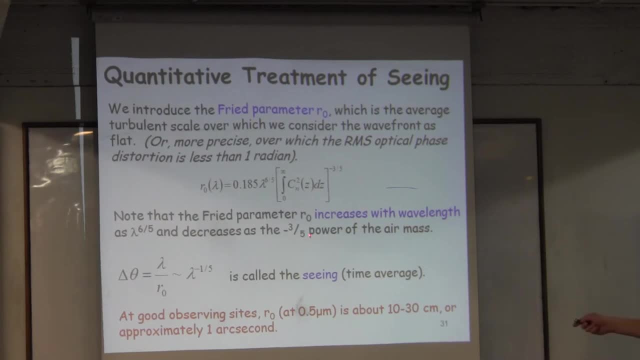 is just bigger. At the same time, if you look through more atmosphere, you get more turbulence, And so it gets worse if you look at higher wavelengths. Okay, So we, we have this formula here that that are not depends on the wavelengths. 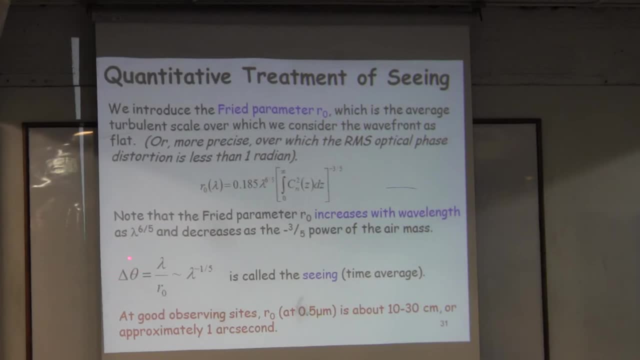 as to the six bit power, And we can determine then a parameter. This is really important. It's called c And that's simply sort of the size, the angular size, Right, We can well, if you, if you think back. 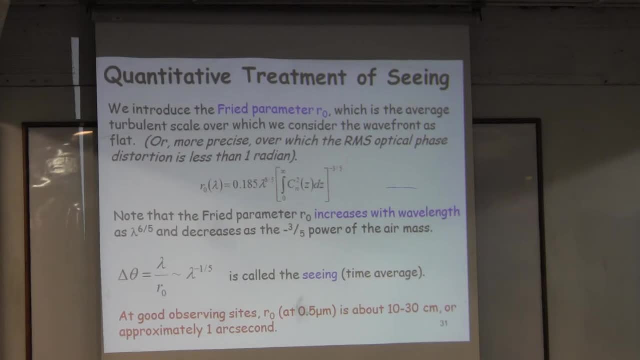 of the comparison of those two pictures, you could just fit, say, a Gaussian profile to to any of the stars in the in the c limited dimensions in the turbulent image and you get an angular size. So so, so so. 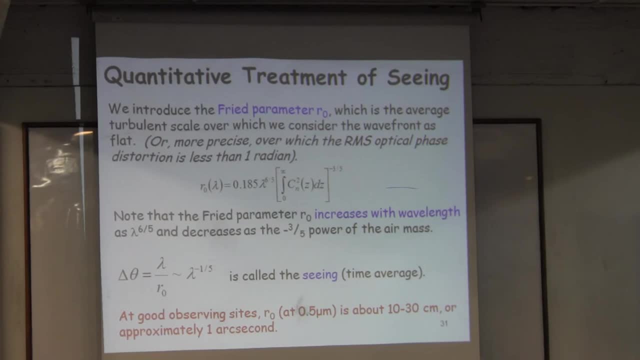 that is really so. so that is actually one thing that is given to you coming to you. so so I can visualize. in any iba camera i can see there are two abge Maximum. Maximum: the temperature, the lambda divided by lambda to the 6 fifths of your left, with lambda to the minus 5 fifths. 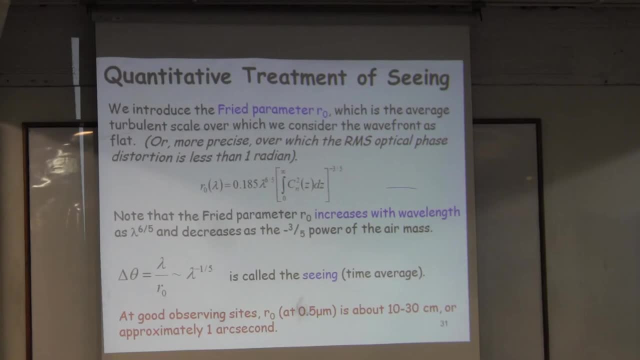 and that means that the scene- sort of the angular size of your scene, your blurred image of the star, will actually get better with longer wavelengths. so the worst scene is an optical wavelength in near infrared. the images get increasingly better with the wavelengths, so if you can then figure out what you have, say 10, 20, 30 centimeters of optical wavelength. 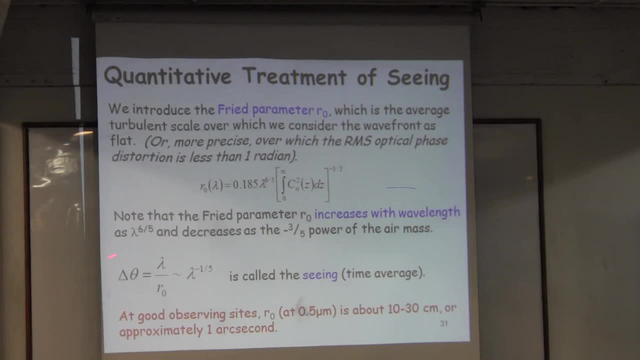 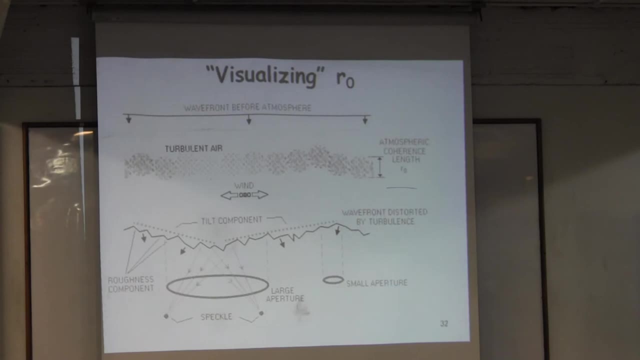 then this increases quite a bit. and then you, according to the scaling model, your scene gets better with the infrared. and here's another graph that may be a bit more sophisticated than what I'm drawing here, but it's essentially the same. so you have the wavefront here, flat wavefront, and then you have the turbulent here. 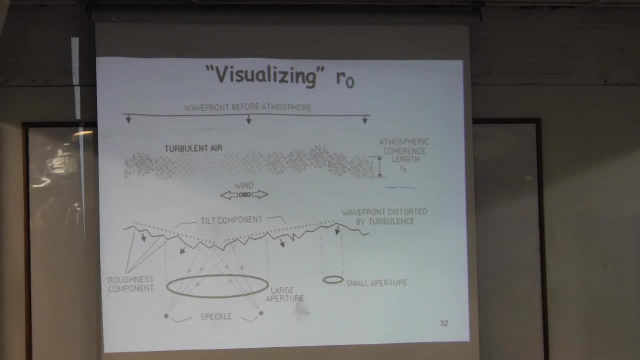 and here maybe some wind, and then you have, of course, structure in this wavefront and I think, again, a simple model to approximate the structure is to say that there is a zero-order component, which is only the, which is the tilt of the wavefront. 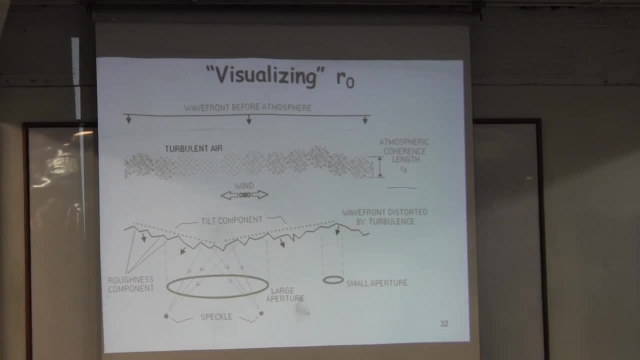 this is the tilt component that gives you the tip-toe of the image motion in the small telescope. of course it's also there in the large telescope, but it's much more. it gets less important there. but then there is also some fine structure. 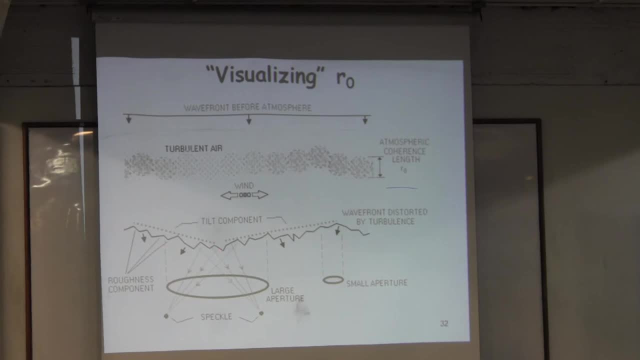 even for the tilted components, the roughness here and that will, if you look at it, you'll see that there is a zero-order component, which is the tilt of the wavefront, and that will give you many different speckles that will work. 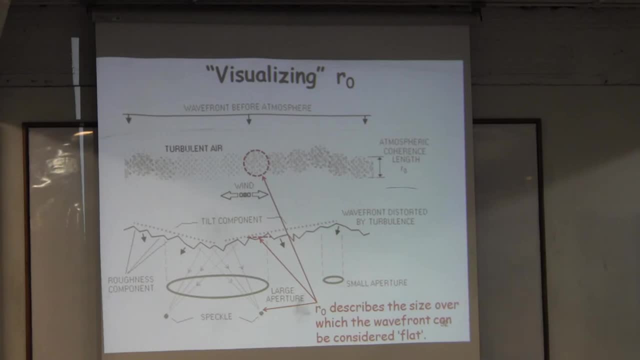 so R0 essentially describes an average size. of course you can't go there and look at the atmosphere and say, oh, I can measure it with a ruler and it's 43.7 centimeters. it's a statistical quantity essentially. you have a wavefront that looks like that. 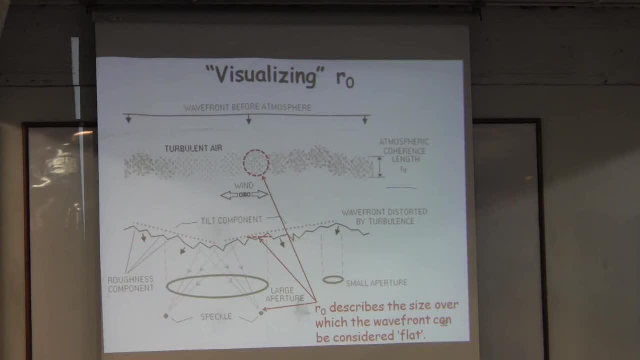 and then remember the definition was: what's the average size and scale over which we consider the wavefront error? less than one radian or any equivalent definition, so we always end up with a number that's sort of approximating a good quality wavefront. 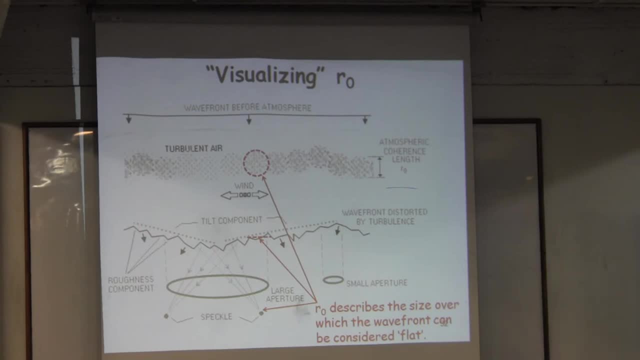 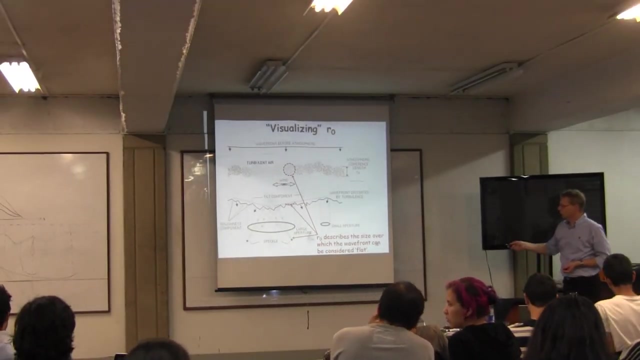 of course it does not have a really physical representation there, but it means that typically, on size scales of a few tenths of centimeters, this is the scale. if you make it larger than that, if you make your telescope larger than that, then you get blurred images. you suffer from this. 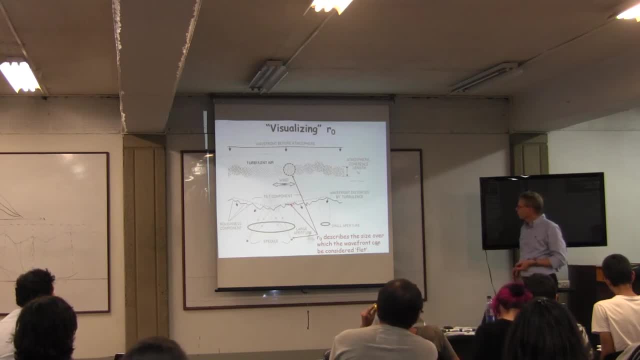 and then, as I said before, each of those are knots, like here. you have two images of the star here and those images are both speckles and each of these are knots and that's a bit simplified picture but produces a speckle. 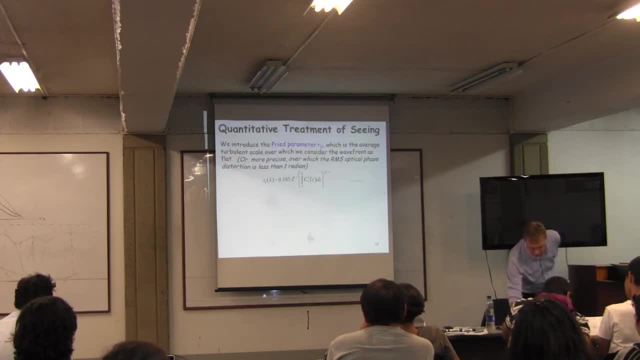 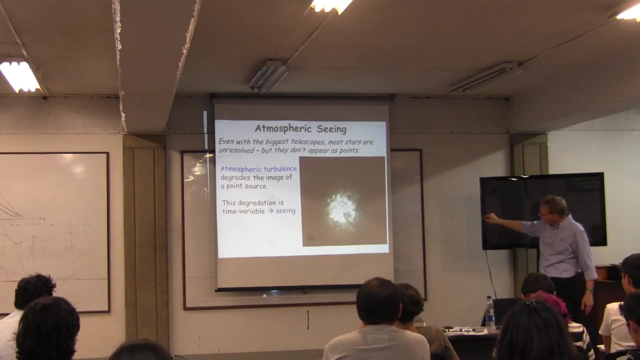 so actually you can see that I should replay the movie because I think it's really best seen there. if you look here, so you see the tip-tilt motions of the cloud, but you see also mid-spawn scar. these are not sunspawns. 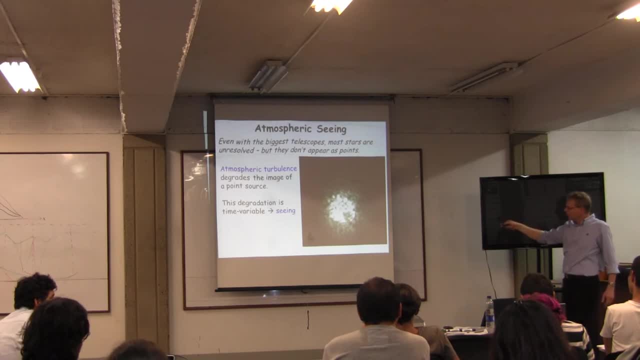 these are sunspawns on the star. remember, the star is not resolved. it should be just a point here. but the fact that you see here many points means that you have many speckles here and in this simple picture, again simplified, you could actually say: well, if this is an optical image. 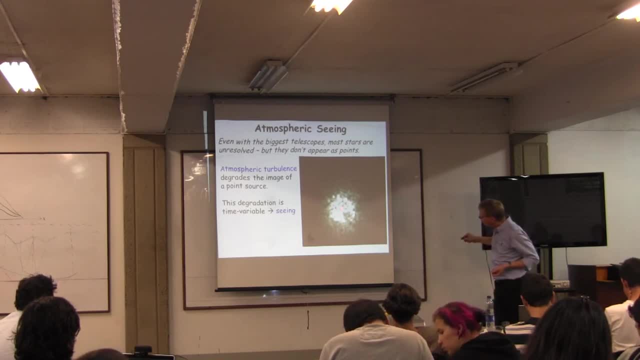 and our knot is 10 centimeters and I have at least 1,, 2,, 3,, 4,, 5, whatever, 6,, 7,, 8,, 10, so I must have had at least a 1-meter telescope. 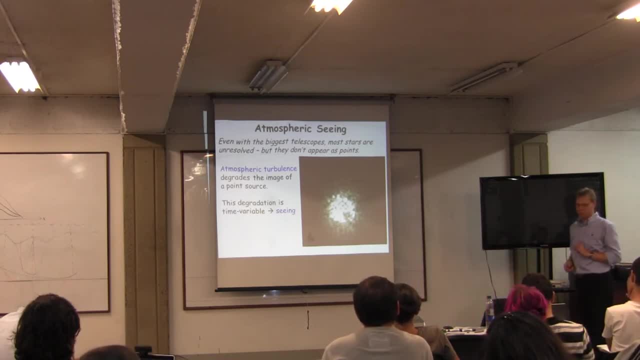 because across your 1-meter aperture you have 10 different speckles, each one corresponding to one more knot, and maybe our knot is 10 centimeters. but that also shows you how complicated it gets now if you build a 14-meter telescope, for example. the atmosphere is still the same, but then you have 400 R knots across your aperture and all of them give you some image of the star and you need to correct for that. so it also means that the most suitable size of the telescope depends on the head you are observing. 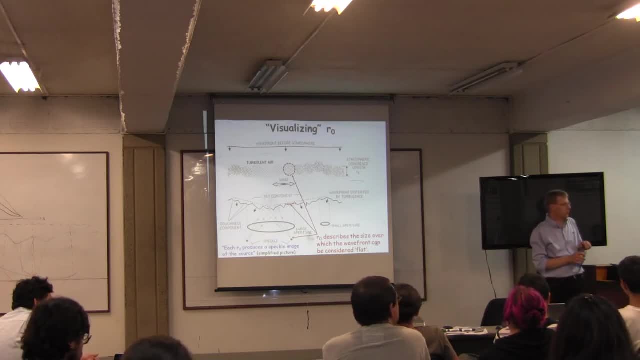 I mean, if you have a very large telescope, you have to be very high where R0 is also very large, and if you go down, for example, here we have this problem. we need to decide which is the best size of our telescope if we are working in our desert. 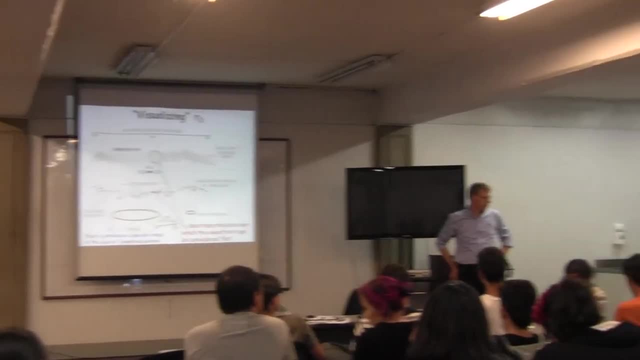 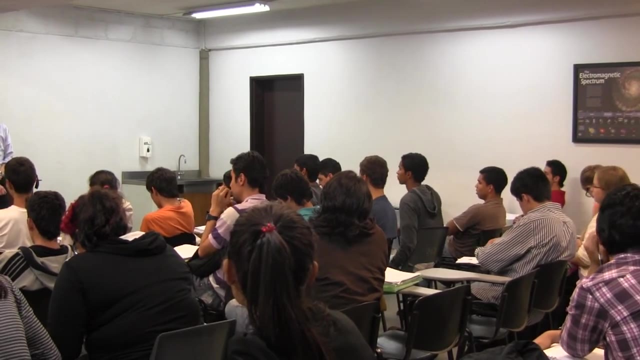 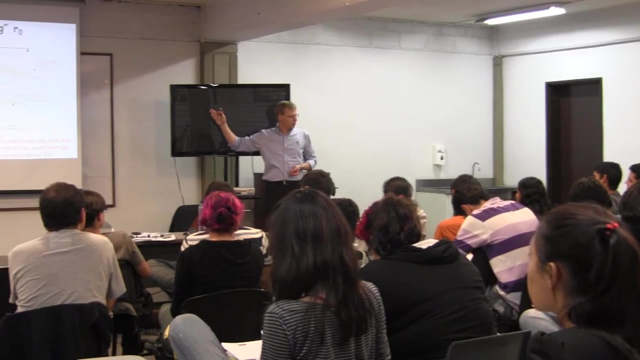 which is at 600 meters. so we need to calculate the average R0 and see which is the best, exactly, exactly. I mean, from those considerations, it's best to be on the highest mountain top. the only problem is- and that's also I mean it's- a practical problem. 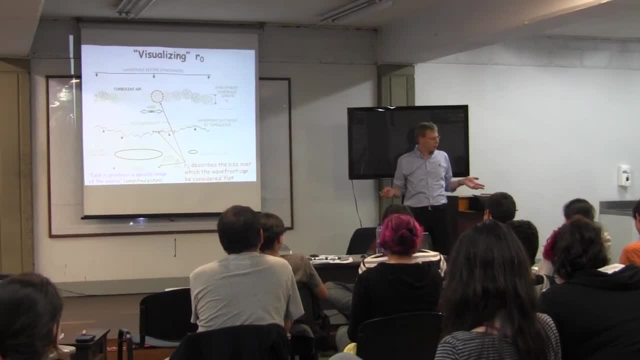 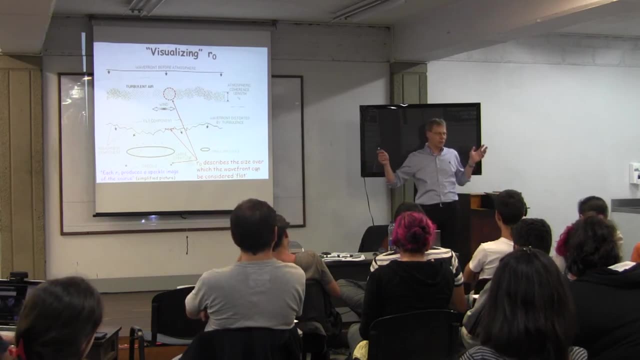 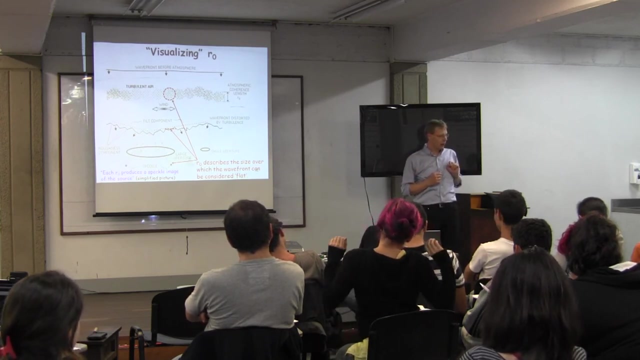 that also ESO, for example, has considered. it gets very expensive if you go up high, if you build it on 2500 meters. I mean, these big things, these are challenging projects. you need many brilliant minds to solve problems and there are no brilliant minds. 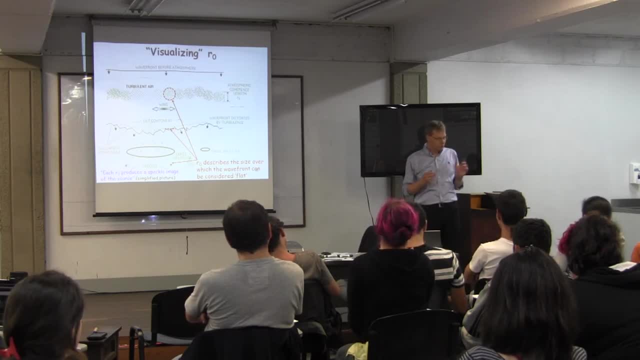 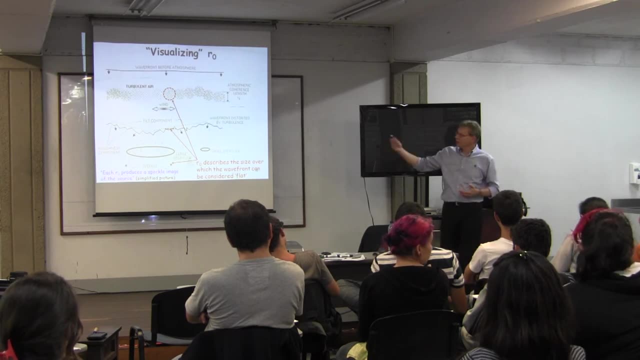 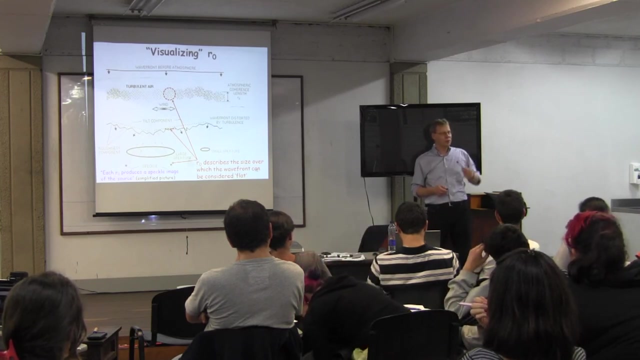 that 5000 meters don't take. you simply can't work there, and that is. you have to then trade on the advantage of better performance, with the fact that it doesn't help you that you have a telescope that in principle would work if all these problems would be fixed. 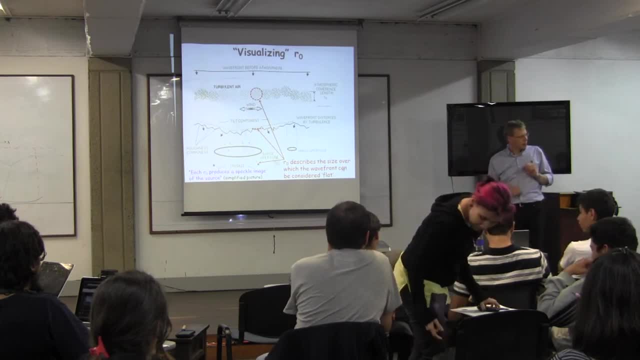 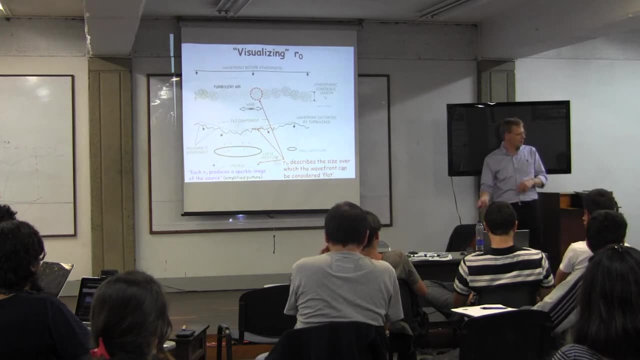 and no one can fix them. so that would mean that if you have to sample everything and test at lower altitude and ship it and the maintenance is still a problem, there's always a trade-off between between performance and practicality. same as for the South Pole. ok. 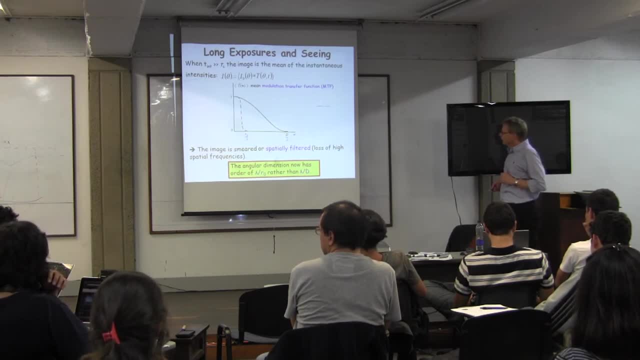 so ok, so what will happen for the long exposure is that, in terms of mathematics- and this is relevant because we can use it- we have better images by image processing. let's say we have, we don't know, we don't need to understand really what this is. 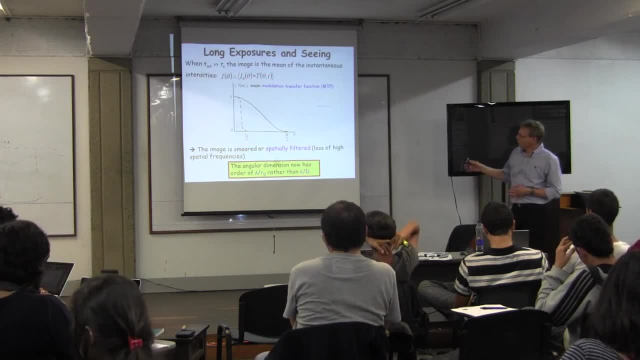 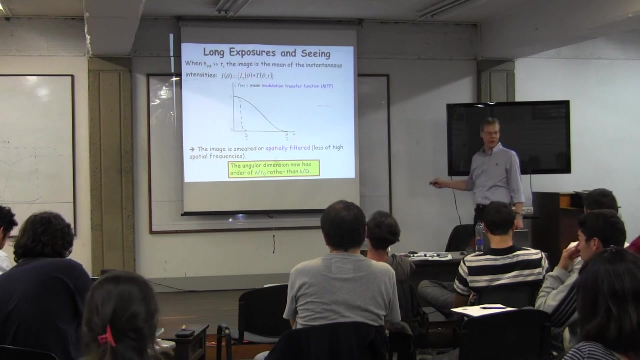 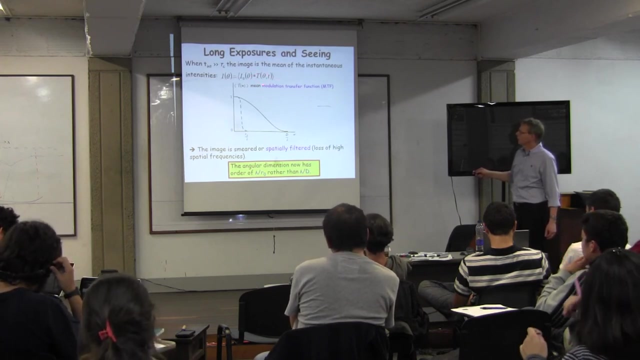 but all we need to know is a simple picture. to describe a scene limited in long exposure is to say, well, we have an intrinsic intensity distribution of the source. this could be again, this could be a delta function and we convolve it with in this case. 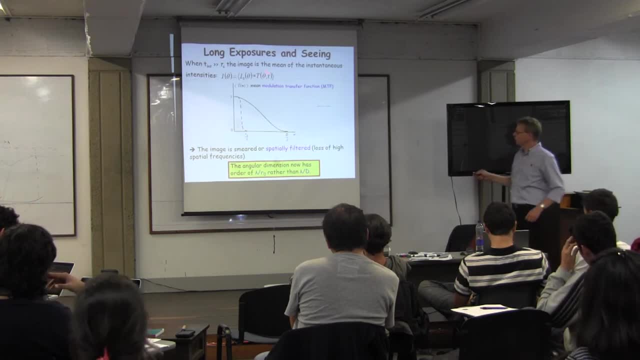 this is the transmission function of the system, which includes the scene component, and what we see then is the convolution of those components. what what this transmission function here does- so that's just the mathematical term- describes the scene, but in a very simple way. what it means for the image essentially is: 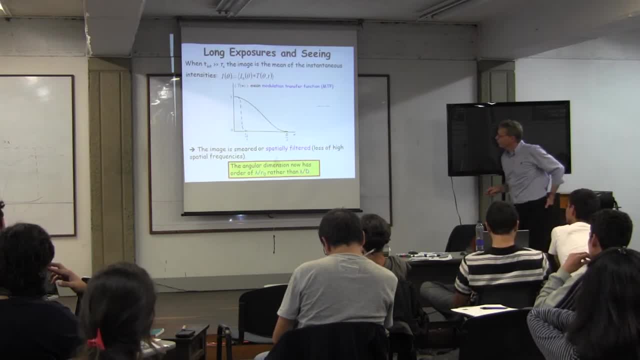 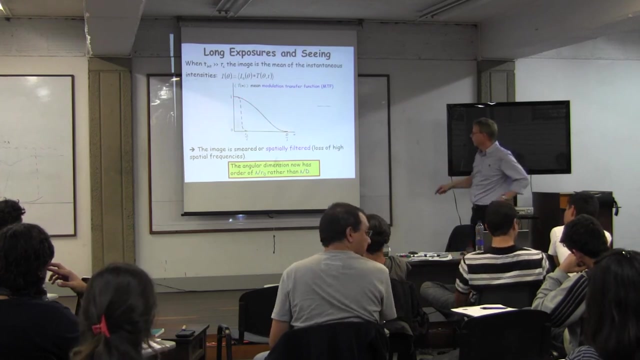 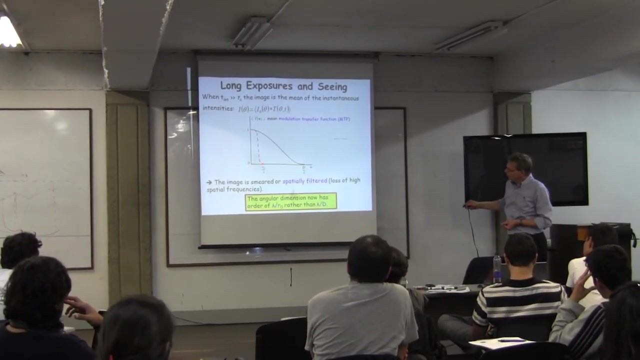 we show here that as a modulation transfer function and we'll get back to that tomorrow. the main thing is that you would have an image as a modulation transfer function, like a solid line, if you were diffractually limited and if you had a scene. this resolution. 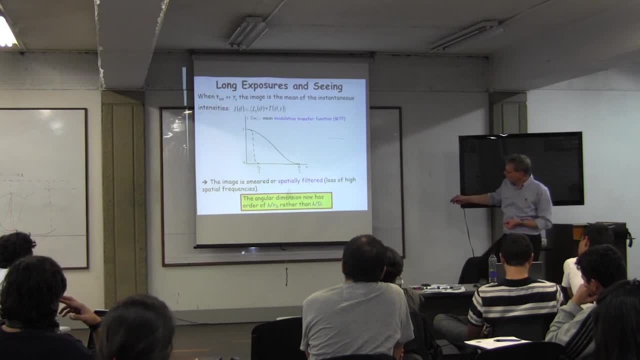 the size of your image would be smaller, would be larger, meaning that the image is mirrored, meaning that it's spatially filtered. so essentially, you have a loss of high spatial frequencies. I mean, what's this what we'll get? I realize this is maybe a bit out of context. 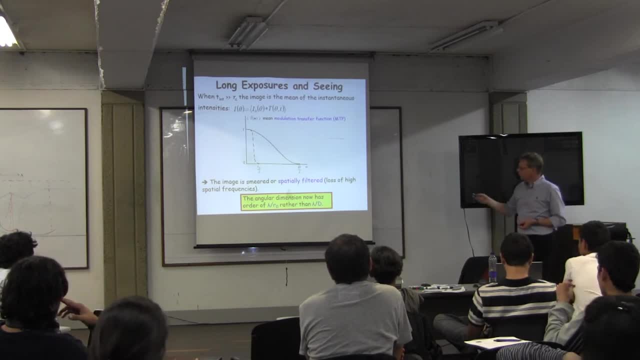 it will hopefully become clear tomorrow in the next lecture and we'll not ask about this then tomorrow in the test. but it's important for to keep it in record because the angular resolution with the scene is then back to a resolution of lambda with length over the street parameter. 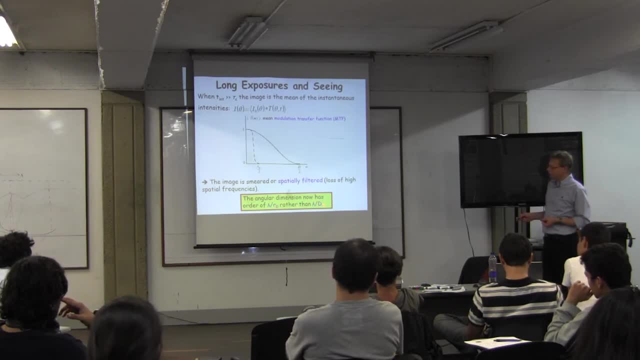 rather than what you could achieve if you had a diffractually limited telescope. that resolution would be lambda over the street, and so lots of high spatial frequencies mean simply that, let's say, you have a very close binary star, so you have a very tiny distance in between. 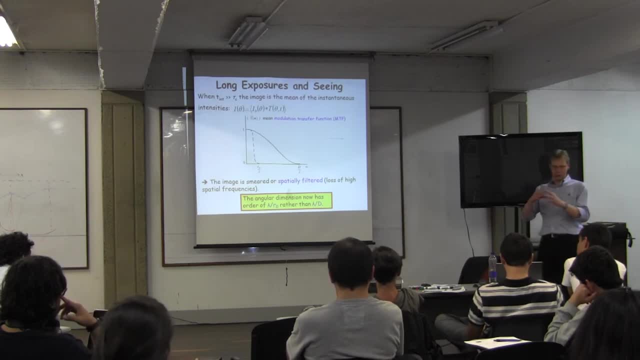 a small distance means high spatial frequencies and this would be lost, meaning you cannot separate them. so, in simple terms, we lose high spatial frequencies and the resolution is degraded in the long exposures from lambda over b to lambda over r0 to r0 over the street parameter. 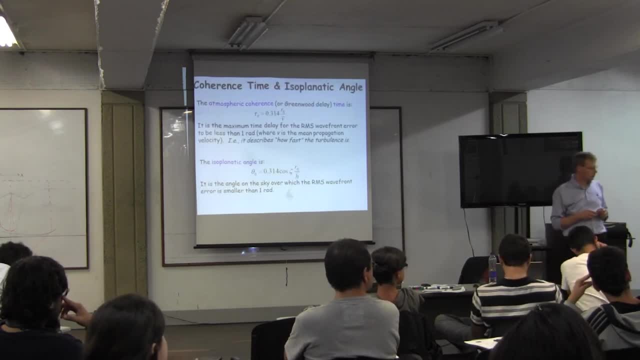 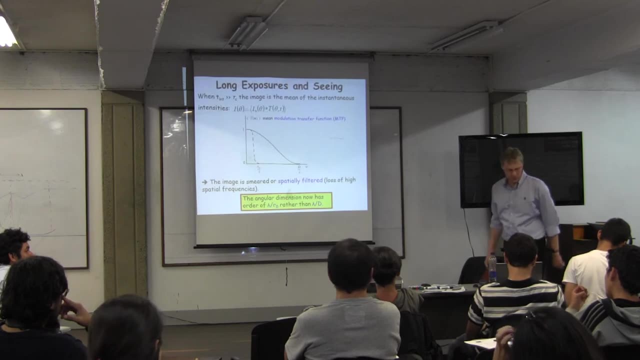 so it means that having a telescope, a 100 meter telescope, will be the same as having a 30 centimeter telescope. do not if you do not, correct for the scene. the resolution is given by lambda over r0. r0 is the property of the atmosphere. it does not care what size telescope you put behind it. so, yes, the 100 meter telescope will not give you a better resolution than Raphael's telescope. if you don't correct for the scene. well, it will still collect more photons, so you will still have brighter images. 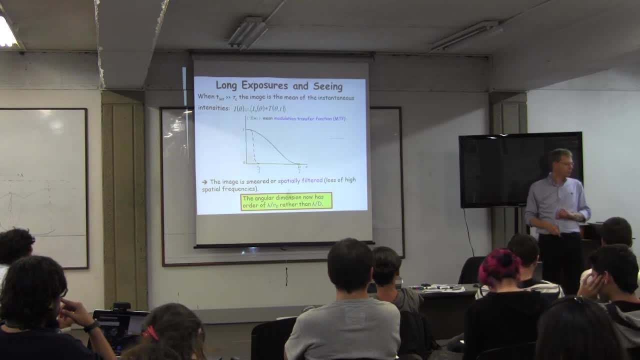 but they have the same blurred structure as the small telescope and this is the reason why all the big telescope projects in larger than 8 meters essentially include adaptive optics and that's why you also saw the chart, see the fire. there were some people you were looking for. 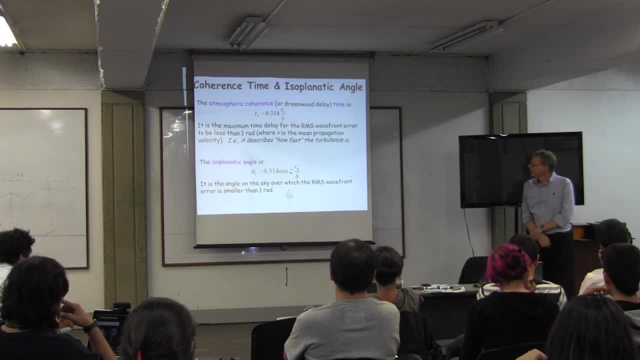 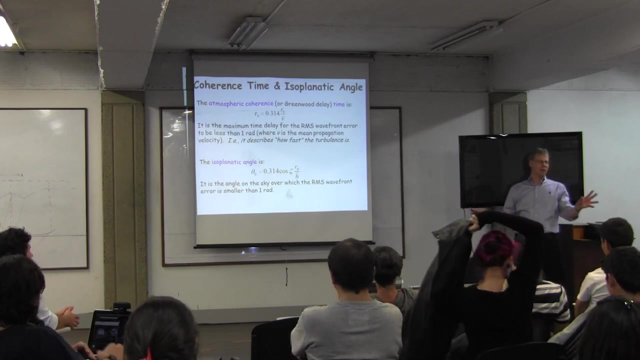 yeah, ok, there is one. there are two more aspects, one that we should consider, namely that that's also important when we when we adaptive optics, when we discuss it later. so let's say there is a technique that measures the wavefront, corrects it, fine. but the problem is: 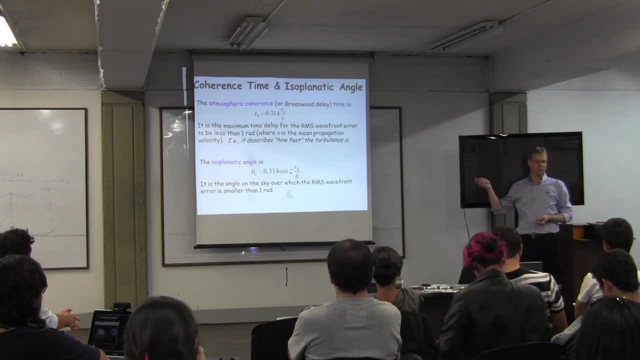 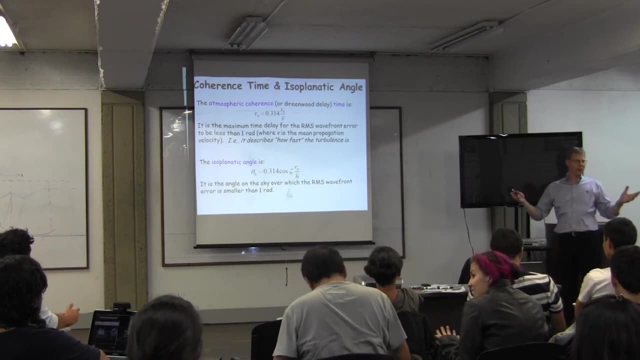 that the atmosphere is changing in terms of the turbulence. it's not standing, so it changes, and it changes on timescales of a few tenths or tenths of seconds, and you can actually calculate it. this is called the atmospheric coherence time. so this is essentially time over which. 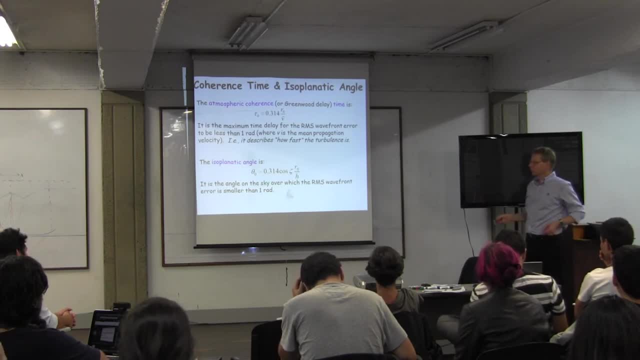 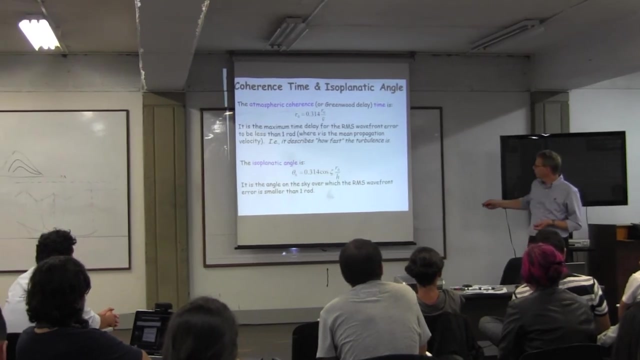 the image quality would stay constant, but the time over which there is not much change in the structure of our wavefront. more quantitative, where the wavefront does not change again by more than one radian. so this coherence time describes how fast the turbulence is any system. 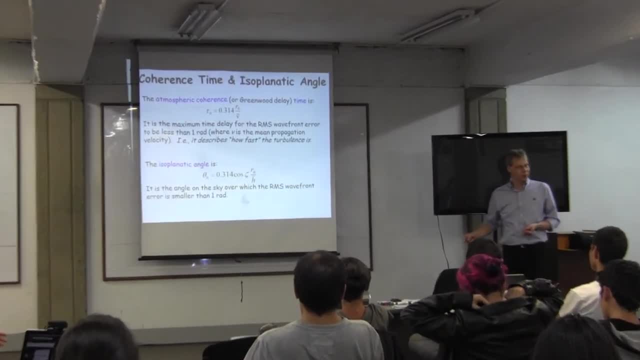 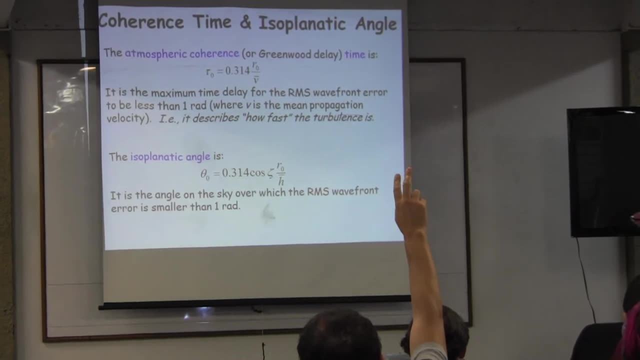 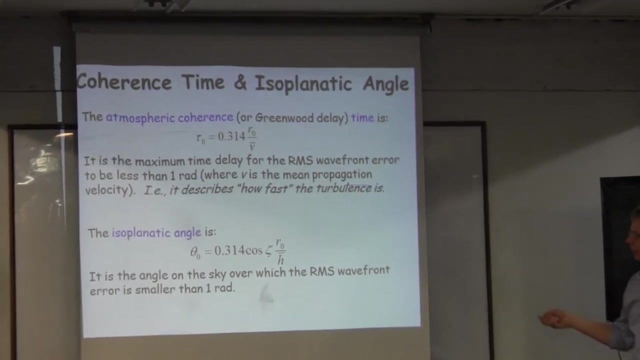 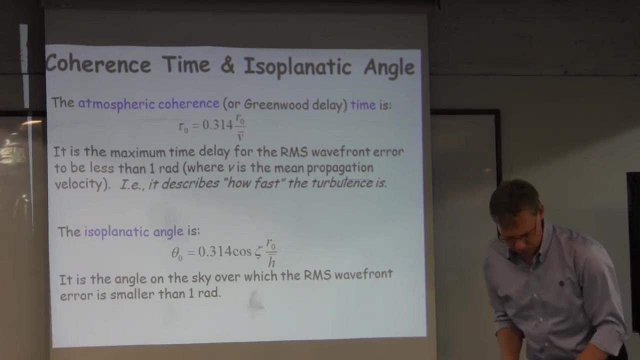 you build to come correct for this turbulence of course has to be faster than that. and the other thing is the sort of the angle, and that's a very nasty thing because let's say in the ideal plane of the wavefront, let's say the ideal case. 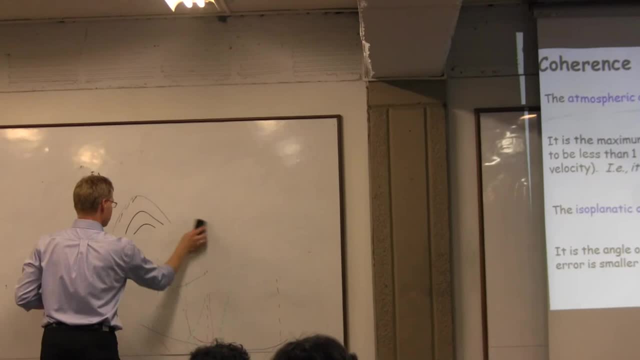 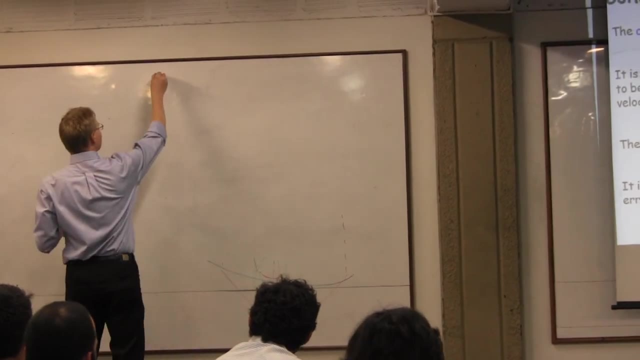 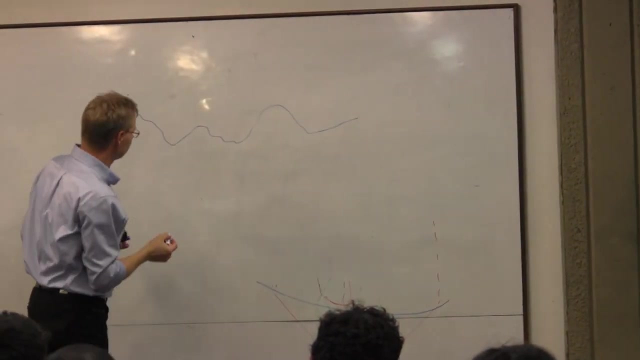 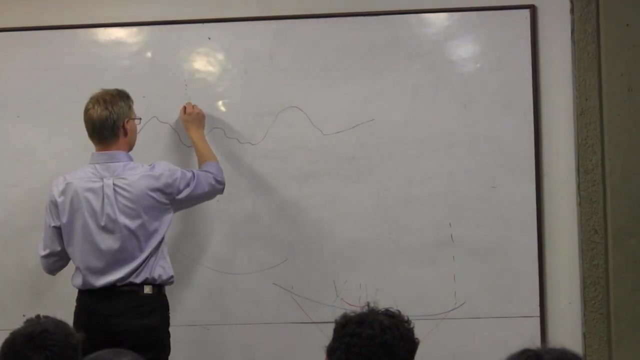 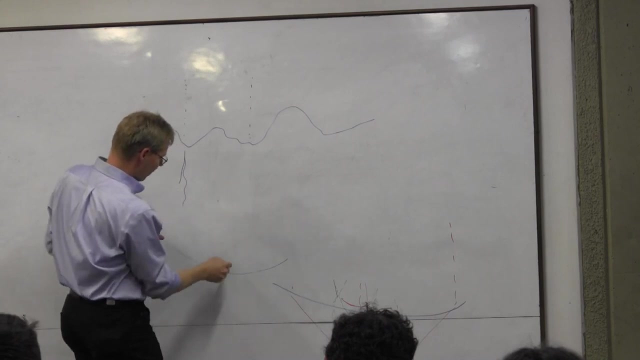 here is that we have the. okay, our star is at infinity here and we have the turbulent wavefront and we have the telescope here. so if it's at infinity, we have parallel light coming in here and we let's say, okay, it doesn't matter. but let's say 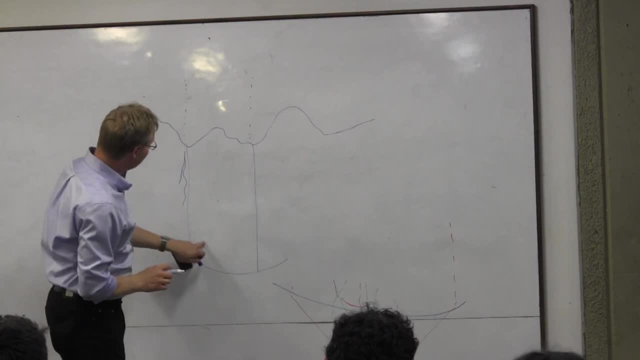 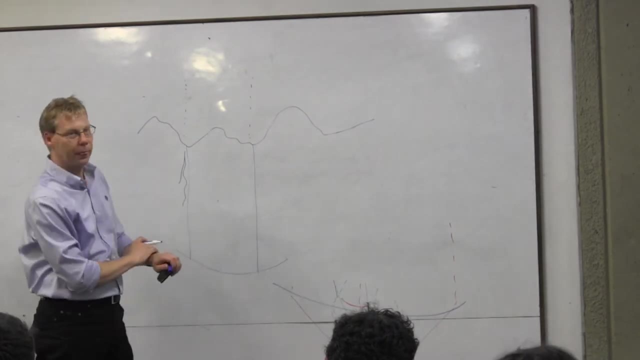 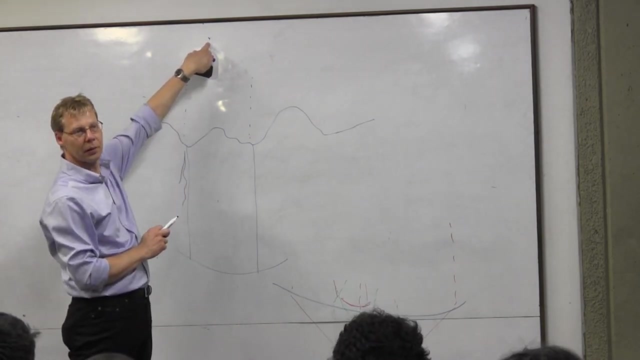 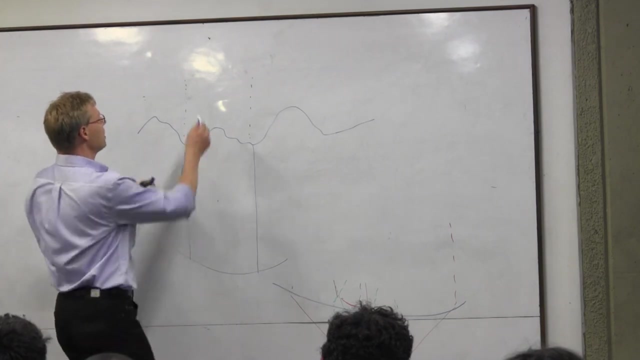 we have here above our telescope. we can measure that. don't worry how we do this, but we measure this level and we can correct it, and then we get a great image of what we want to look at other objects as well. right could be, could be some. 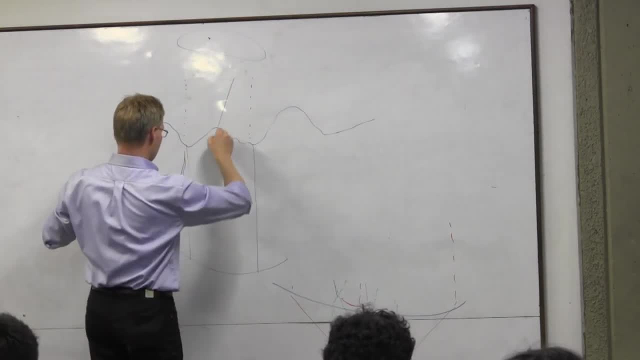 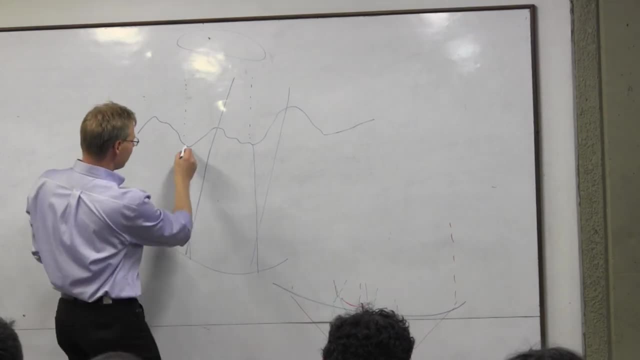 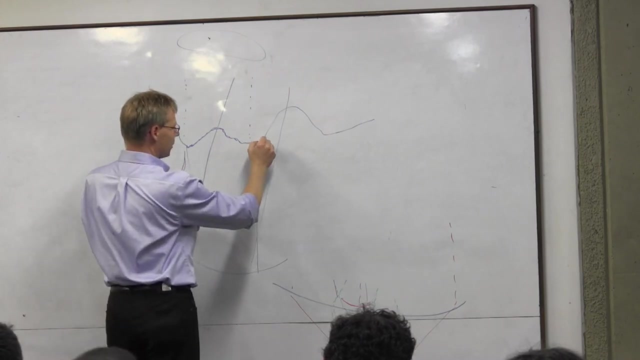 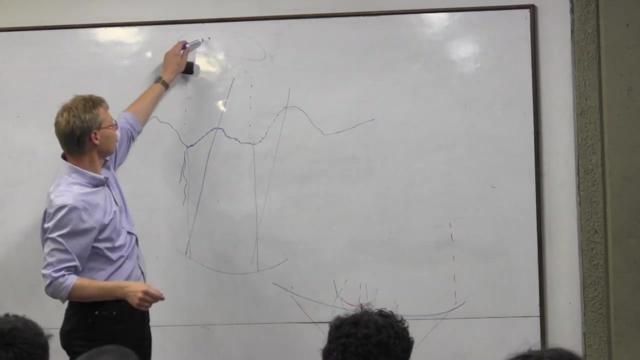 galaxy. here the problem is, if I look at that part of the galaxy, I would have to look in this direction right now. I measured this part here of the wavefront so I will not correct for that, obviously, if I measure my wavefront using a star here. 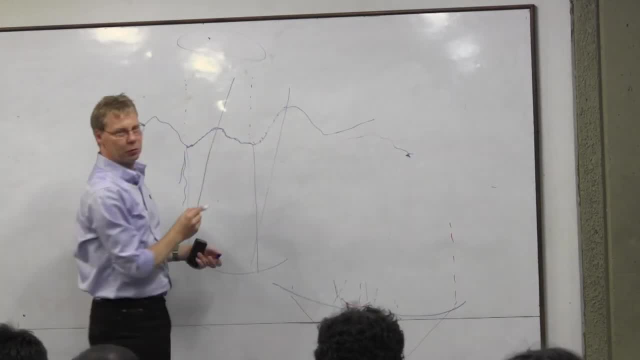 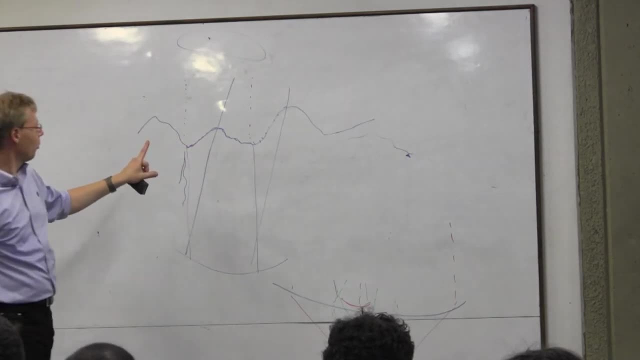 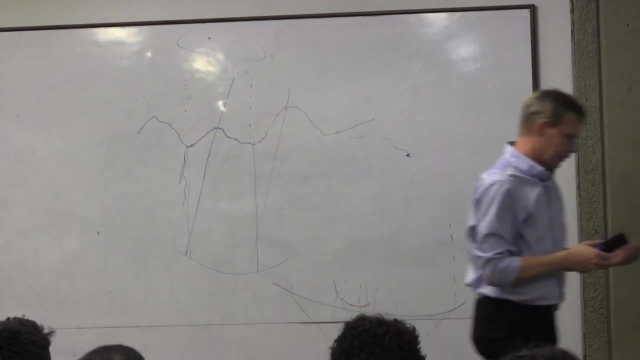 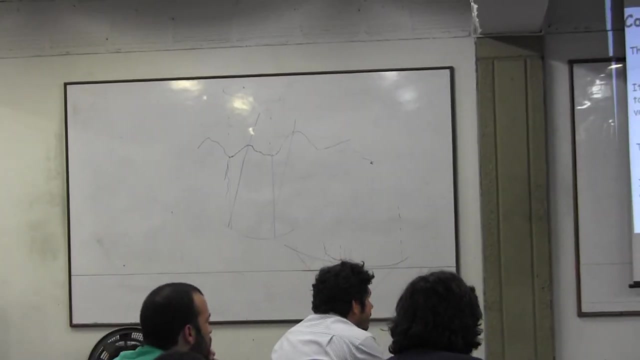 and look at an object here close to the horizon. whatever the atmosphere does here has nothing to do with what I measure here. so all these systems that correct the atmospheric turbulence by this parameter here, the isoscelenetic angle, and again we see the, the. yeah. 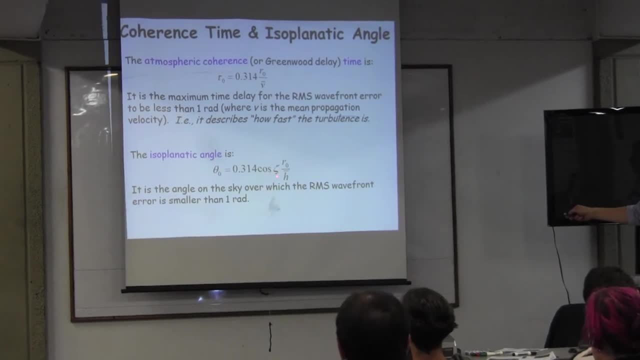 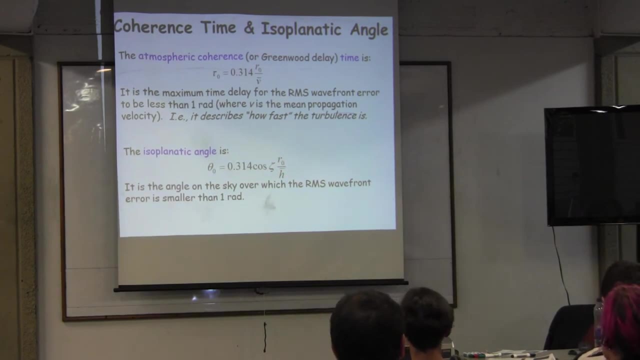 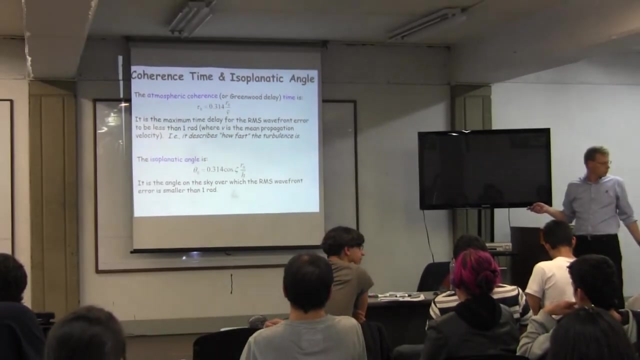 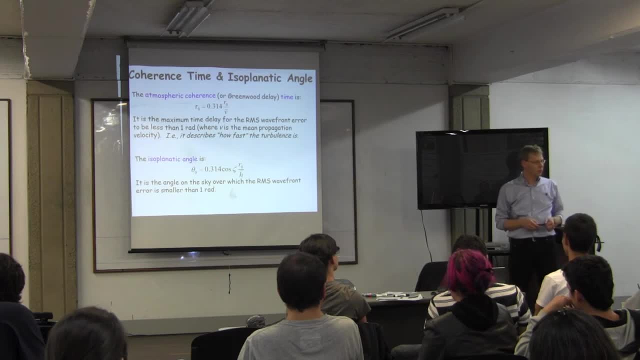 people building an eigen out the resistance to are actually worried about thinking better about, about computation speed, even including Moore's Law. You say, OK, I only need it in 10 years and I will do the processor speed now and then, Even then it's challenging because you 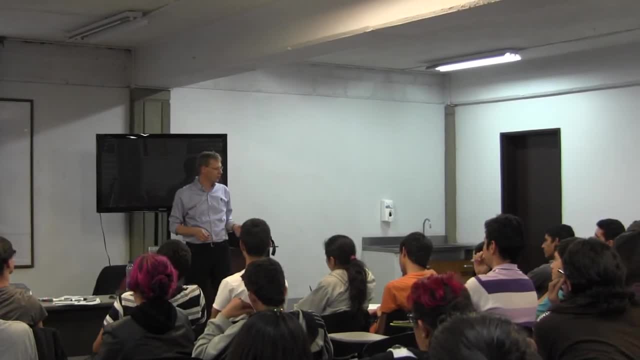 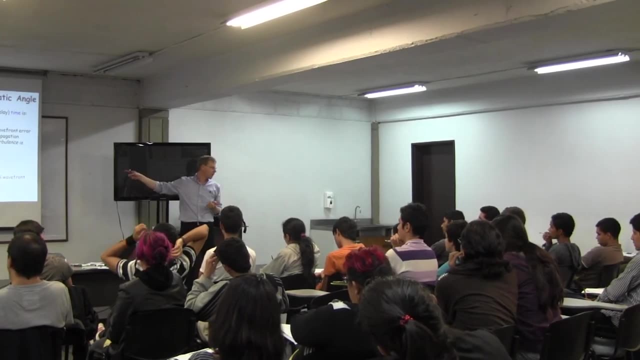 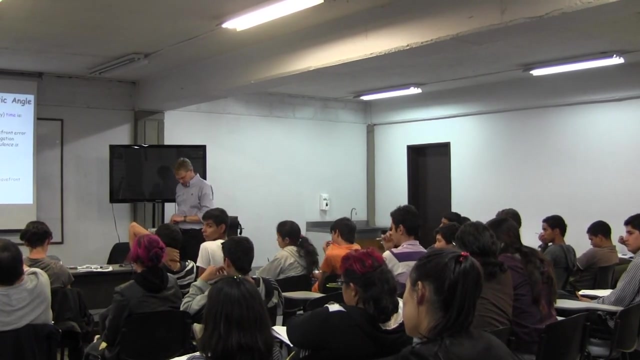 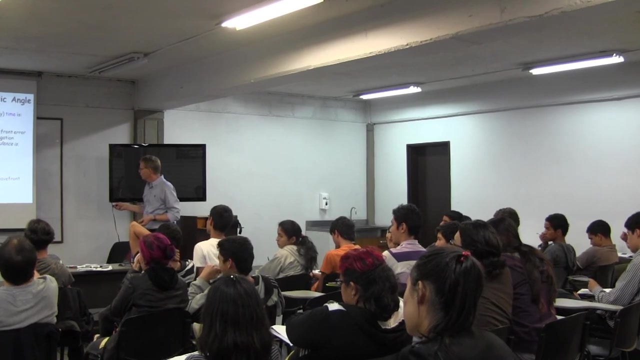 have to do all kinds of complex matrix inversions, with diagonalizations of matrices of 400 by 400 elements, and make my feelings exactly the same, Bernard, which is this cos, cos, this grid that I don't remember. I think that's the. That's only the Ah, OK Again. everything gets more difficult when you get close to the horizon. That's one of the reasons why most modern telescopes only work to 60 degrees. I mean, of course you can move them further. 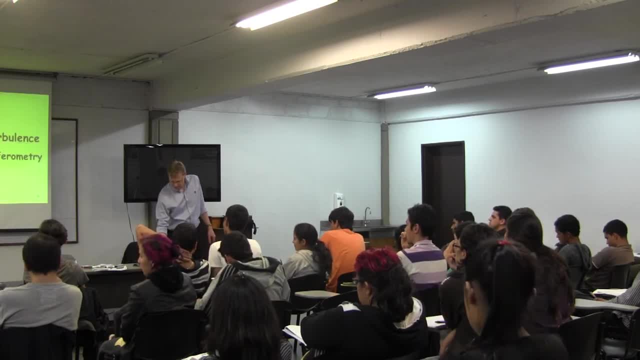 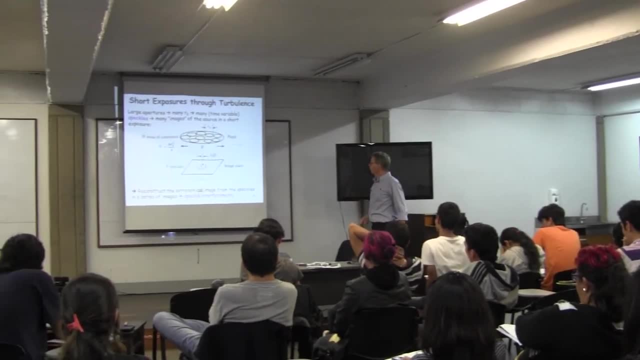 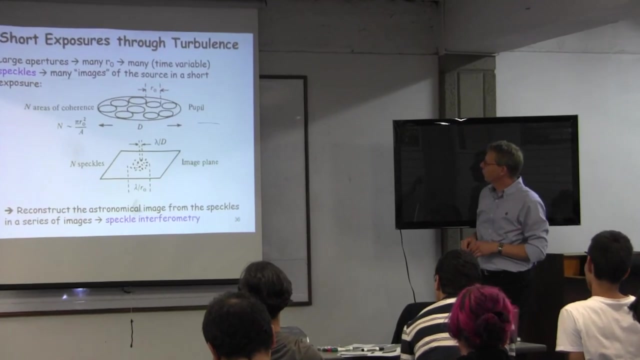 but OK, And now, finally, we talked about speckles, So this should not be new to you. I just thought if I show more many times the same thing again, it will become a bit more. So OK, we said you have a large telescope. 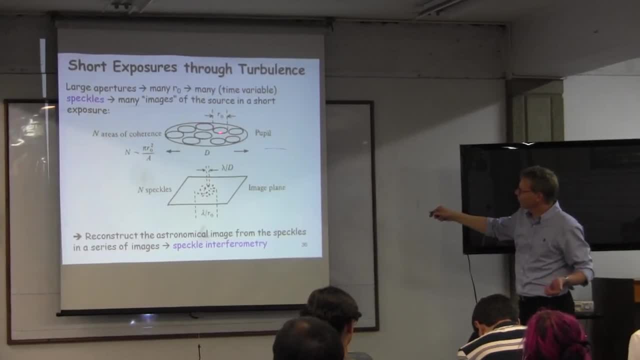 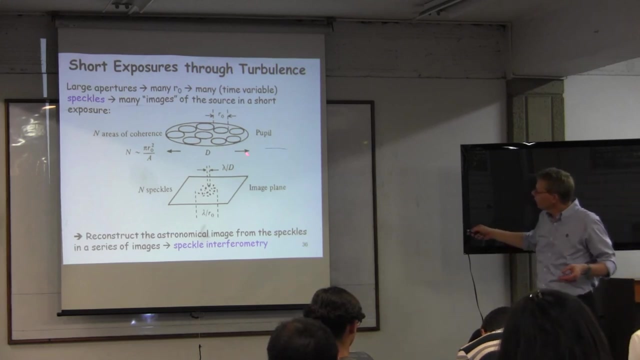 That means that there are many, of course, of these are not above the telescope. So this is your telescope temple here, And this is the effective size over which we set the wave from flatter than one radian, So in that all of those produce an image, 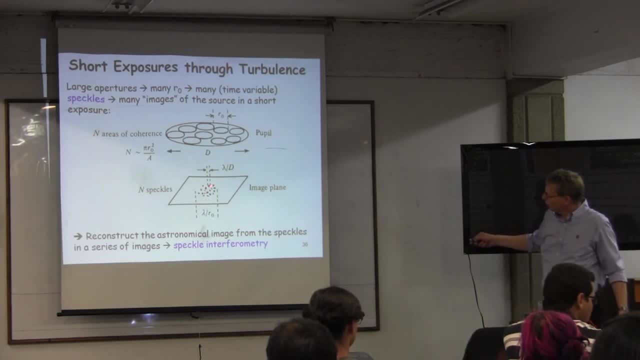 And this image would be sort of a diffraction image. one speckle here Where the size of the speckle cloud is lambda, over r0, right The time average that will give us the C cloud. But there is information in each individual speckle. 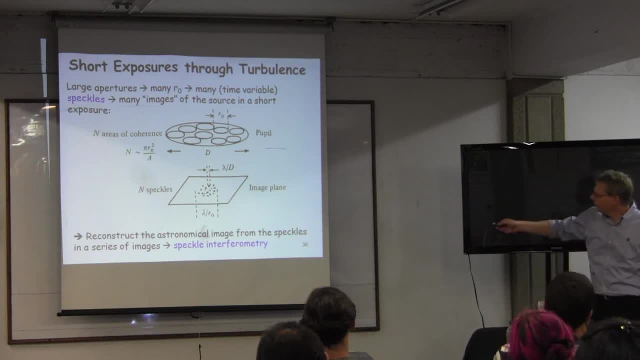 And so people said, oh, hold on, If I take short exposures, maybe I can preserve the information that's in each of those speckles. And the speckles tell us more about the object than the time average. That is all washed out over time. 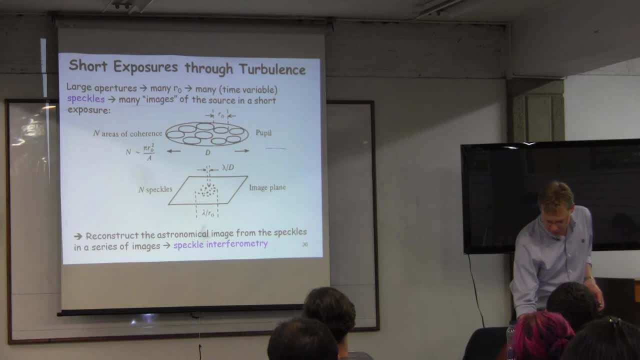 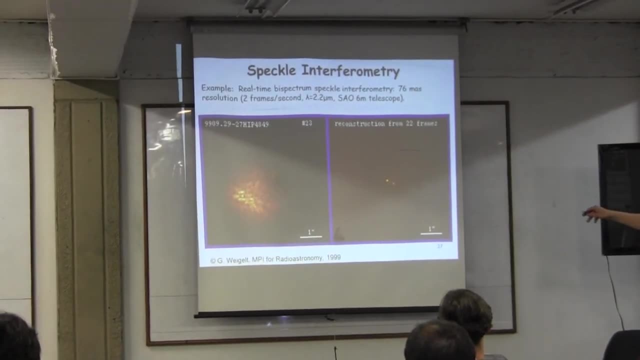 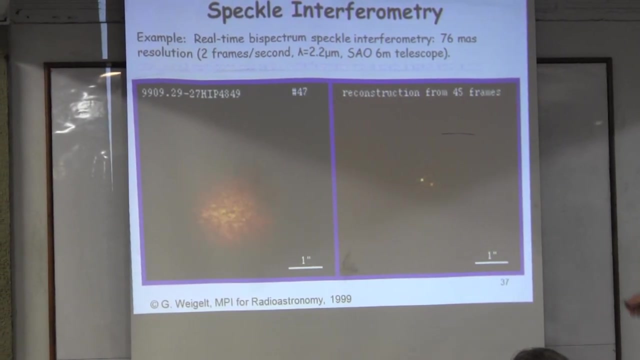 And this is called speckling. This is called speckling in interferometry, And I'll show you a movie here. This is adaptive optics. This is not adaptive optics. This is just taking serious. what you calculate is the coherence time. 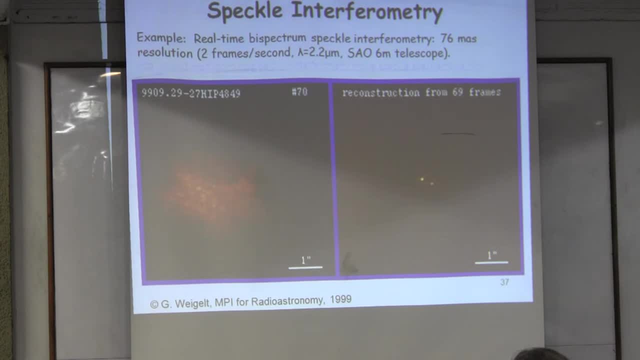 So obviously I have to take exposures that are shorter than the coherence time. Well, at maximum that makes sense, And if I do that, then during those I say the wavefront is constant, And then, OK, this is the integration time. 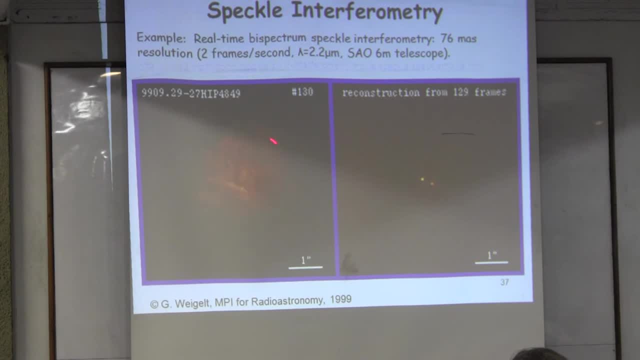 And that's shown here. So all of these images that you see here is essentially the image of the object And you can see it's moving around. Remember the overall image: motion. That's the tilt-tilt component, the overall tip of this wavefront. 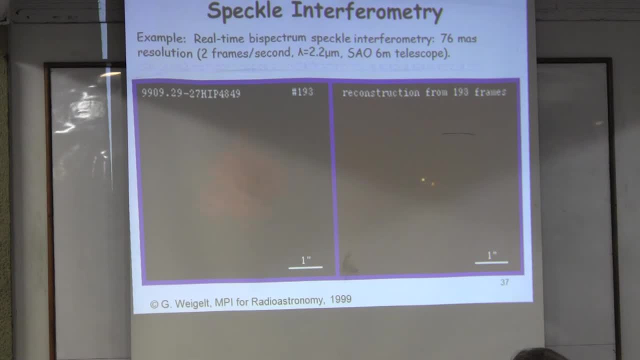 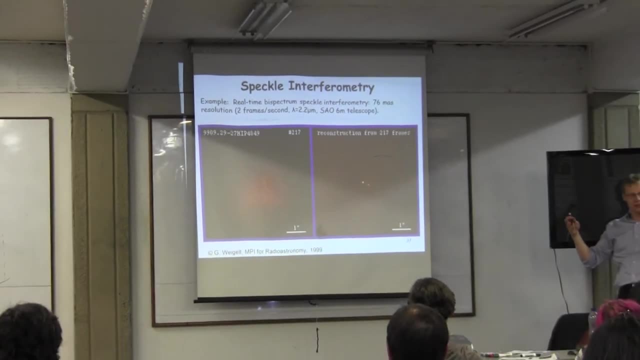 And you can also see how the amount of turbulence changes. I mean, now it's really bad, Right, It's not constant, It's really. sometimes it gets much worse. Sometimes, now it's getting better, The brighter the spots here are. 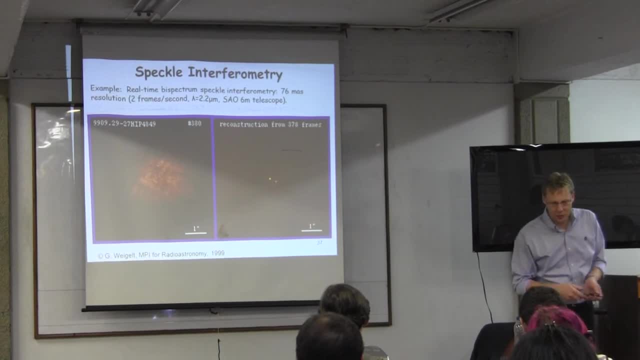 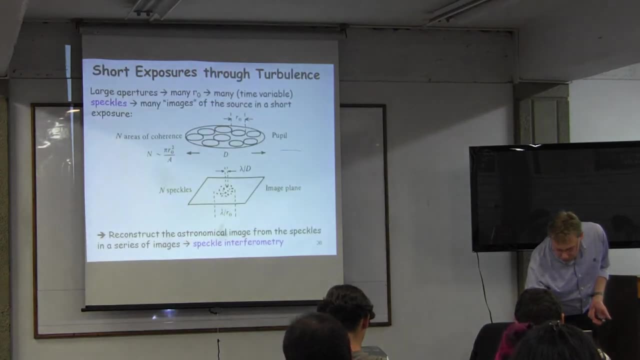 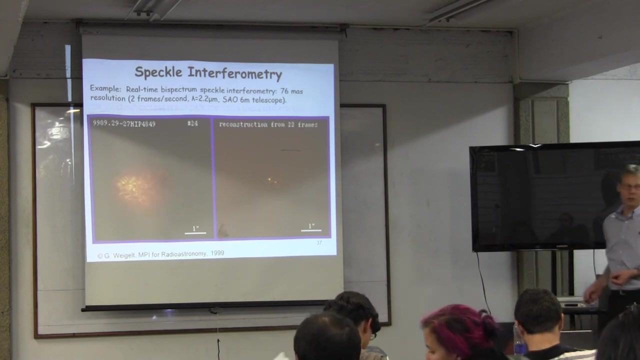 that means the more light actually is concentrated, And that's probably a significant sign. OK, and what people do then is to use that information mathematically- And we don't have to go into how this is done- But to use the information with cross-correlation. 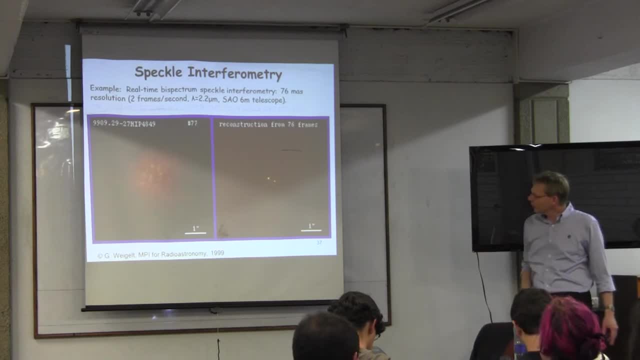 essentially of the various speckles in here and reconstruct an image, And what's shown on the right here is the reconstruction, taking information from all the images into account. So you have now, well, we are at frame number 120.. Again, we just we don't co-add them simply. 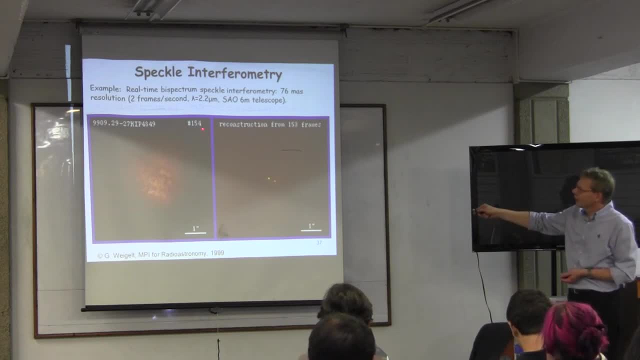 But a computer analyzes these images and then just adds the information from the individual images, not the images themselves, And then from the reconstruction. from the reconstructions, you get this image Right, And I think it's obvious what the game is right. 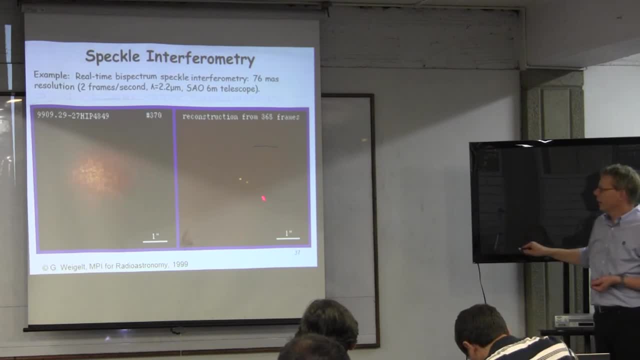 No one. if I show you that image, you would not have never guessed that it's a double star system. To what extent does speckle replace the? Yeah, That's a good point. The problem is, if you remember, the exposures have to be shorter. 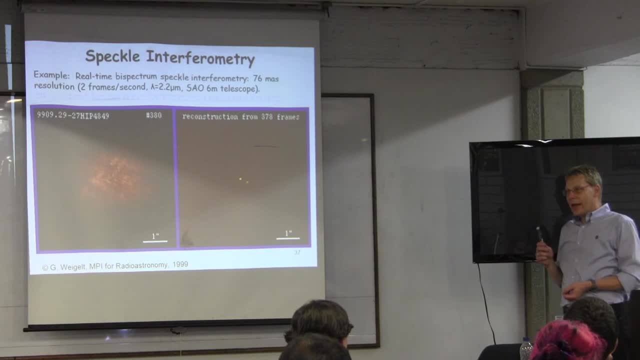 than the coherence time, And you need to. you need to be able to see the speckles, So the method is limited to objects that give you sufficient signal to noise in 100 milliseconds. So we need to. where are the detectors? 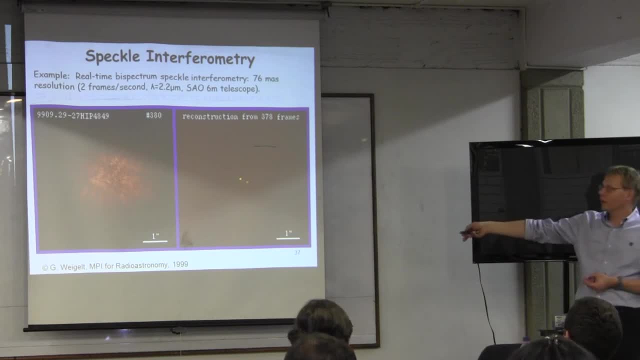 Well, it's a imagine you would like to, because you say: oh, I look at my gamma ray burst at the ratio of whatever seven or something. Right, It's a faint object And I want to see where it is in the gamut. 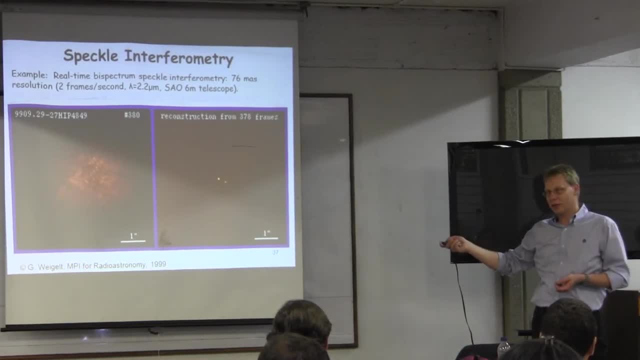 The problem is that you have to expose it maximum, say 100 milliseconds, And you will see nothing. So what's the computer going to do with that noisy image? It will not be able to reconstruct anything, And so this is very limited to. 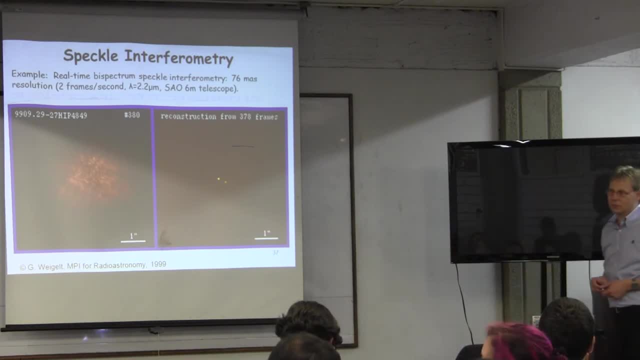 yeah, bright objects. You also need 410 more storage in your computer to get all these. Yeah, Move them.